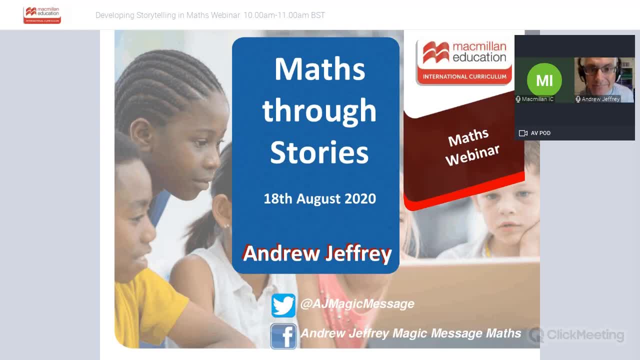 session focusing on maths through storytelling. If you have any questions, feel free to write them in the questions box. Lovely that you're all able to see one another's comments. As I mentioned earlier, please try to stick to the topics of the webinar itself, But of course, 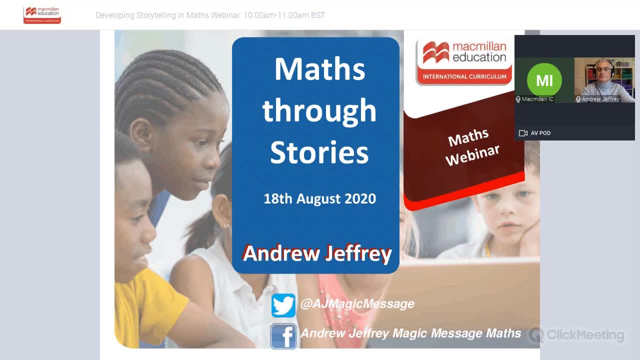 if you want to mention the weather, then feel free to do so as well. As I mentioned, CPD certificates and the PowerPoint presentation will be available automatically after the webinar, So do look out for that In your inbox. it may fall into your spam or junk folder, So do check that as well. 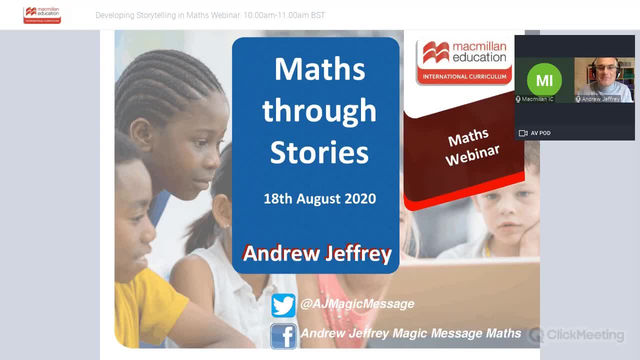 I will pass it over to Andrew now, Thank you. Thank you, Raina, Good morning, good afternoon, wherever you are. I see people are in Kuwait, Nice, to see you. My name is Andrew. As Raina said, I am a maths consultant and I love stories. 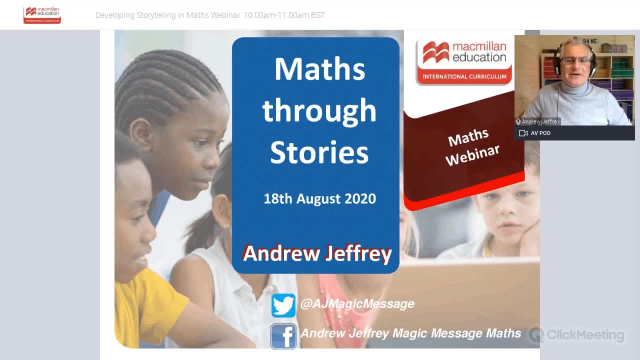 And I think that's one of the things I want to start with really is to look at why. Why maths through stories is a good thing. So I'm going to share some stories with you and I'm going to give you some ideas about how we might use those stories in a maths. 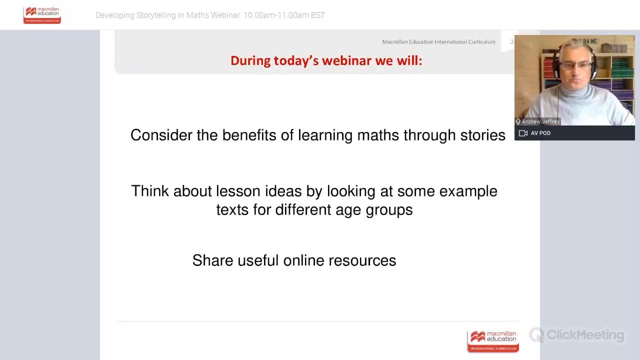 class OK, so let's crack on. I've got three goals for today's session. really, I want to first of all think about the benefits of learning maths and think about some lesson ideas by sort of got some primary and secondary. 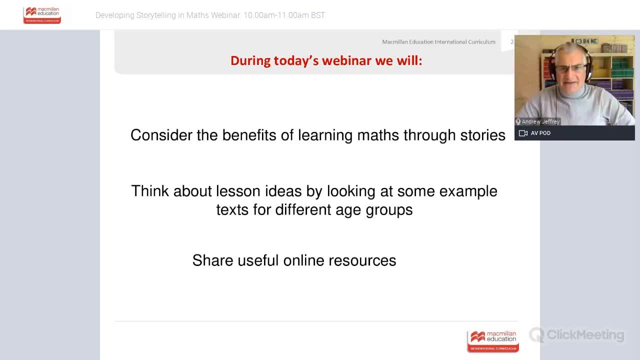 Ideas. And then, finally, I'm going to share with you the three best websites I've found for online resources, because I know sometimes, you know, not everyone has access to the books and that's a challenge. So, yeah, there's some. there's some good online resources. the three best that I found: 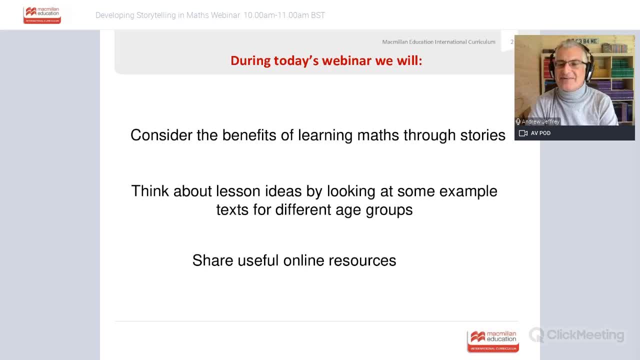 during my research. So I see we've got some Egyptian, Qatari. That's great It's, and there's a debate raging in the chat about whether it's morning or afternoon. So just hello, Oman, beautiful country. So here we go. I want to to first of all think about four reasons why. 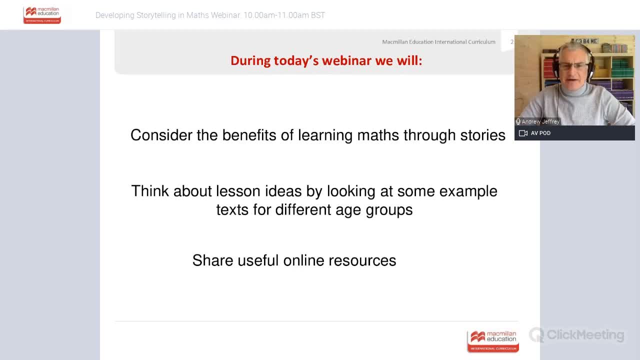 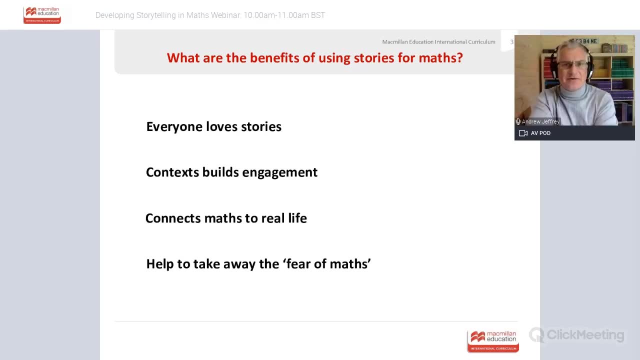 I personally believe that stories are a brilliant way for children to learn mathematics. So let's have just a brief run through of those four reasons. The first one is everybody loves stories. right now, I've never met anybody. You're a very friendly bunch. Look at this. I've never 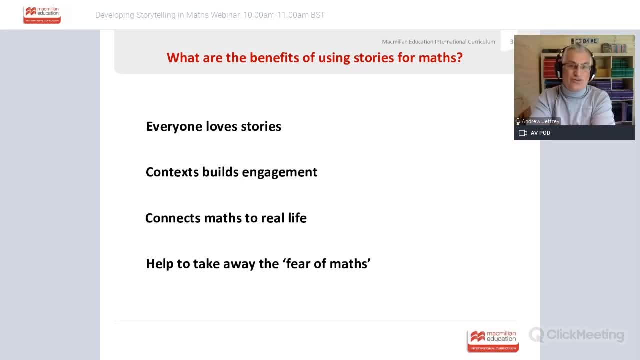 Chennai. reporting for duty. Good morning, I've never met anybody who doesn't like stories. I mean, we make sense of our life through the stories we tell about them. right, Have a story in our head, an ongoing story of of how life is for us and what we've. 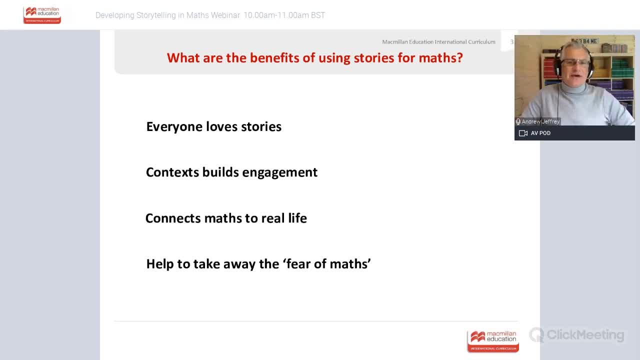 experienced And and everyone has a story. So instantly people can relate to stories in a way that they they will enjoy. So why not use stories? Secondly, those of you who enjoy maths will know it's just a fun thing to do, But there are many people who aren't in that position. 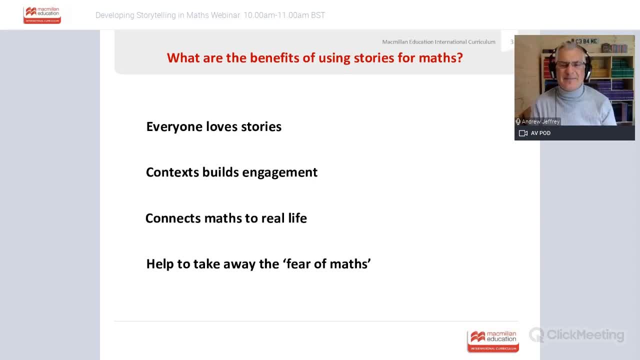 and who don't have that viewpoint because it seems a bit pointless. You know who cares what X is And it's changed its mind from yesterday anyway, that kind of thing. So I think, I think that putting a context on some math, making the maths about something, And in all the examples I've 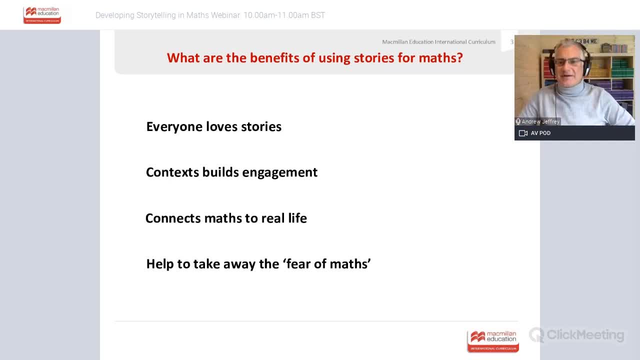 chosen maths that we're going to look at today. maths is about something, So context is important And it makes children care because, whatever you do, whenever you do mathematics, I asked some children in some primary schools in Sussex- around here, where I live in Brighton, and I asked some 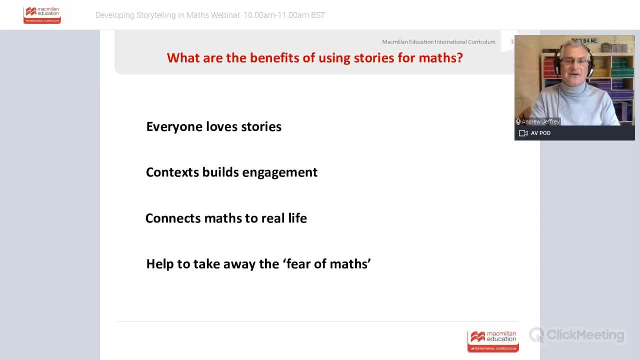 children, when do you do maths? And I ask in three different schools and seven different age groups, But I got the same answer, which is basically just before morning break. And that's such a shame, because you do maths when you cook, You do maths when you shop, You do. 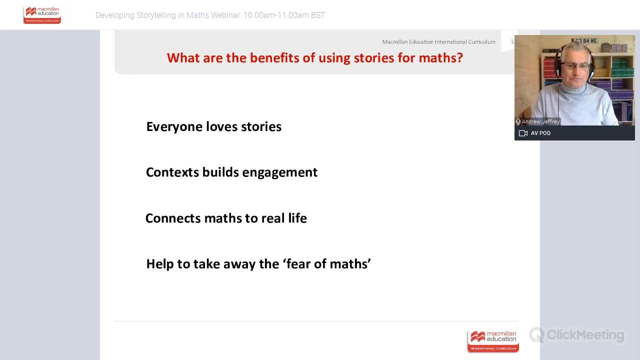 maths when you plan, You do maths when you travel, So you're always doing maths. So I want to connect maths to real life and for children to see mathematics in stories really helps them understand that maths isn't just something you do before break. 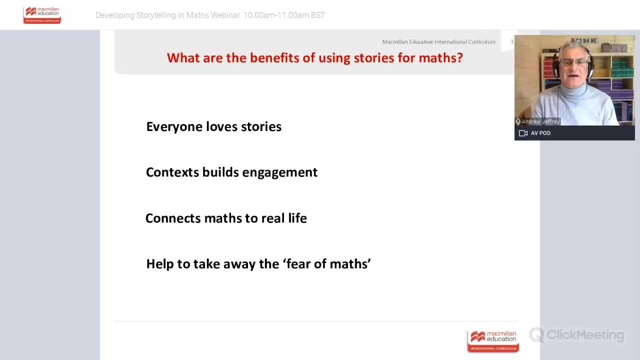 It's not just something you do to get a pass mark, an exam. And then finally, the fear of maths. No one's frightened of somebody reading a story to them. Nobody's frightened of that Because Even in the story, even in the frightening bits of a story, you know it's just a story. you know someone's just reading a book. 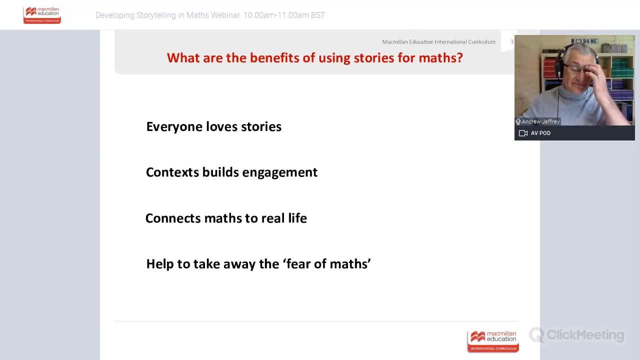 All right, And I think, if we see maths as something that you know, I'm going to give you a question. You must get it right. Is that? that can be frightening for some people, whereas I'm going to tell you a story and we'll start thinking about it is a lot less. 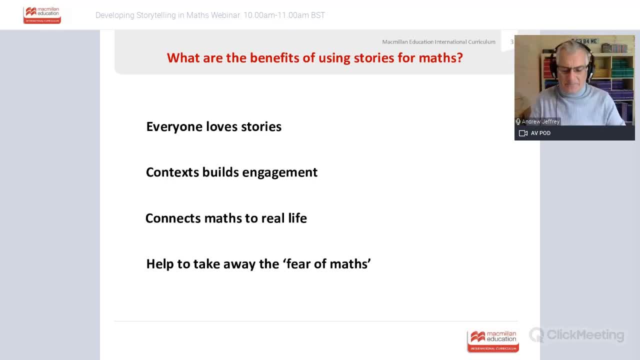 So I think the fear of mathematics can be improved by it, by stories, Right? So what stories are we going to look at? Well, I'm going to look at six or seven stories. I'm just going to talk about some of them briefly to give you some ideas. 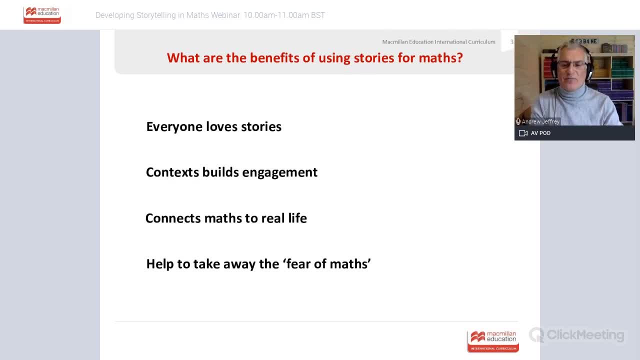 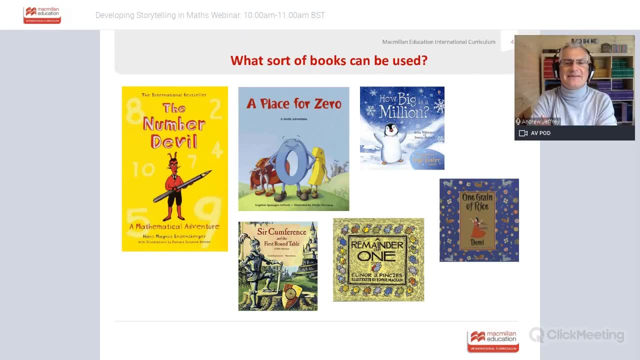 And then I'm going to give you some in a bit more depth, All right, So let me have a look at the first picture. Here we go. Here are some of the stories I'm going to talk about today. Pretty much all of these books have something in common, which is they were written specifically to help the reader think. 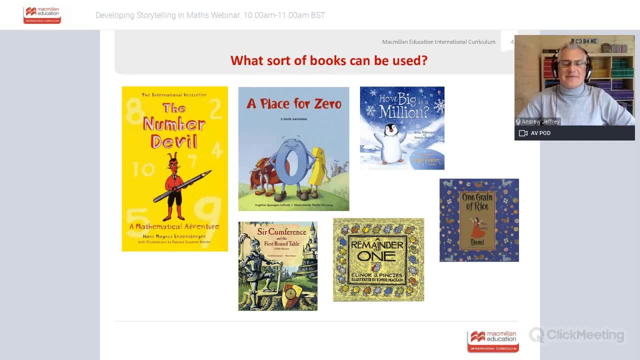 Think about an aspect of maths, OK, And there's stuff right from very basic mathematics up to some quite complicated mathematics too. So let's look at these, And we're going to start with one of my favourites, because I think it's a very, very clever book. 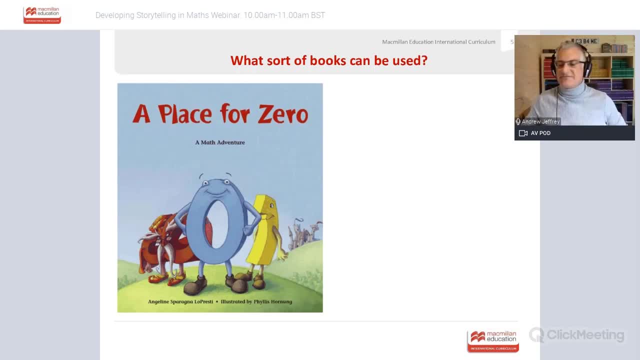 And I would say this is for younger primary children And it's called A Place for Zero. Now I'm interested. Has anyone heard of this book? Has anyone seen this book before? I have a live copy. Just give me a yes if you've seen this book before. 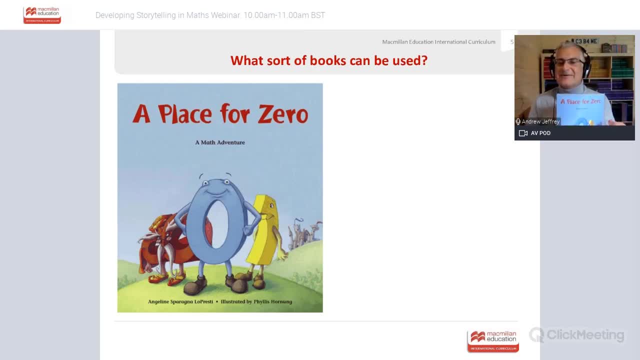 See, a few people are typing: Yeah, we've got a. no, We've got a yes, We've got a no, We've got a no, Yes, yes, yes, OK. So actually about half of you have seen this, maybe less than half. 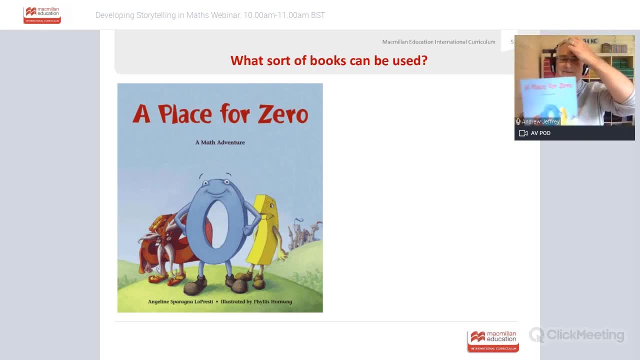 Oh, and Juliet's actually got a copy, So someone's already going to try and find it. Well, wait and see what you think. So this is a book that I thought. I just picked it up casually in a school library. I thought it was so clever that I bought one, because zero is a really difficult idea. 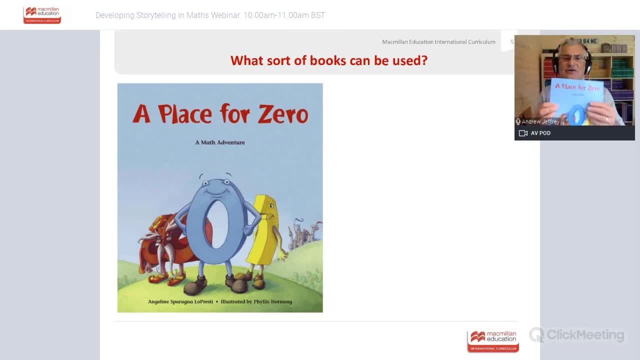 And so what we call Personification, the, the creating of a character, that zero, who doesn't see, who sees there's no place for anything in their life, They seem a bit pointless, is is a really powerful idea, I think. So let me start reading it. I'm not going to read it all, I'm going to turn to the side so you can see. 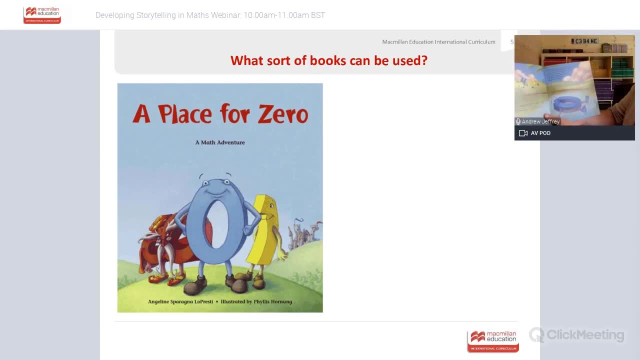 OK, Not long ago, zero lay floating on the calm waters of Central Lake. Did you remember to turn my mic around as well? He could hear the happy cries of the other numbers, one through nine, as they played in the meadow. Zero didn't play Adam up because he had nothing to add. 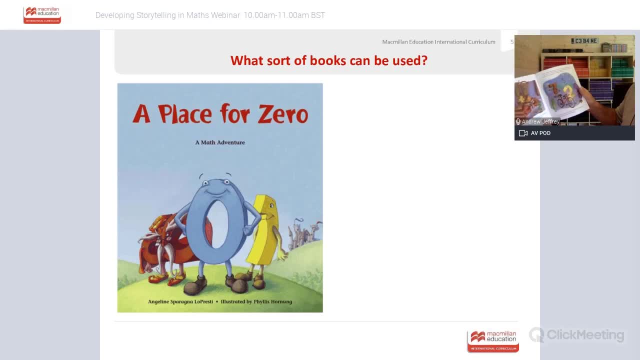 He felt he had no place among the other digits. Oh zero lived in Digitaria, a curious country ruled by King Multiplus and Queen Adeline. Their positive outlook helped the kingdom prosper, So I'm already chuckling Count Infinity, I love. 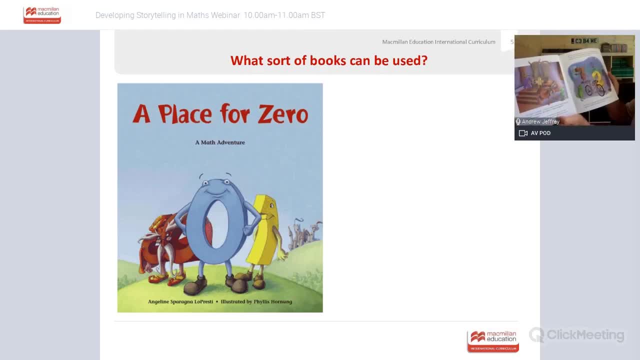 I love that name. Counting entity, the king's trusted advisor, was the one who shaped all the numbers. When old digits retired, he replaced them with shiny new numerals. Every number knew its place. A seven was the number of days in a week and five was the number of points on a star. 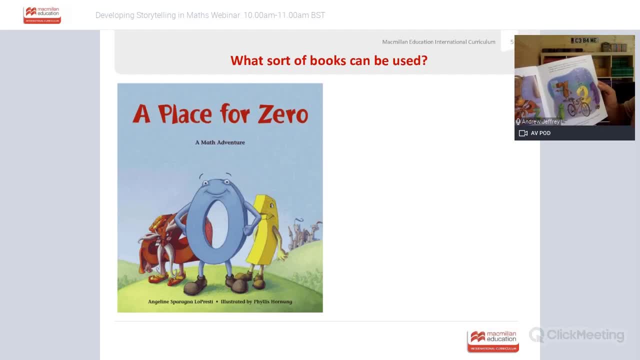 A two was handy for counting the wheels on a bicycle. The ones were important because Count Infinity added them together to make the other numbers. Now, don't worry, I'm not going to read every single page of this book. I'm going to read it to you, although some of you might quite like that. but it basically goes on to talk about how alone zero felt. 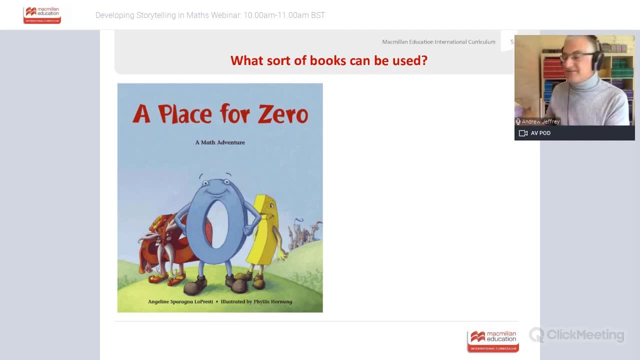 He had no place, OK, so he went to Count Infinity and Count Infinity has this number machine and he would put numbers in together to see what came out. and he put three and four in and out would come seven. And he tried putting a number one in with zero and out came one. and he said: oh, you see, that's what you are. 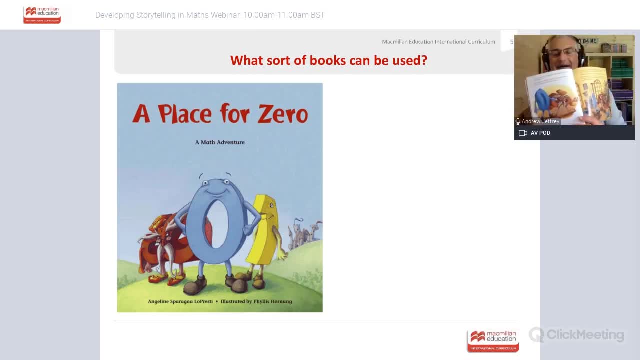 And he talks about His identity. he's so the clever use of the word identity that you see in in secondary. we think about identity that with the additive identity is zero. zero is the identity under addition And it's a big, big, big maths idea adding zero to anything. 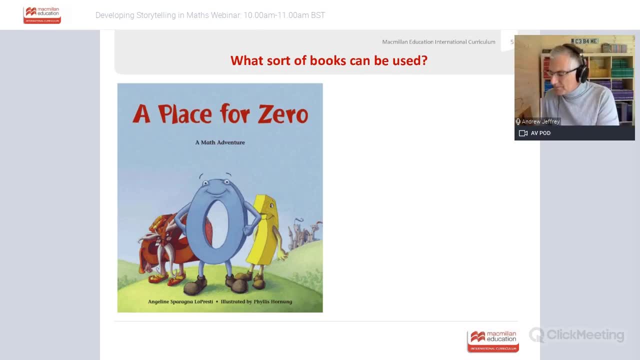 So they just make it into a story. Anyway, to cut a long story short, he hasn't found his place, He doesn't know his values. He goes to see the king, King Multiplus and he gets multiplied in this amazing machine that you put two factors and a product in. 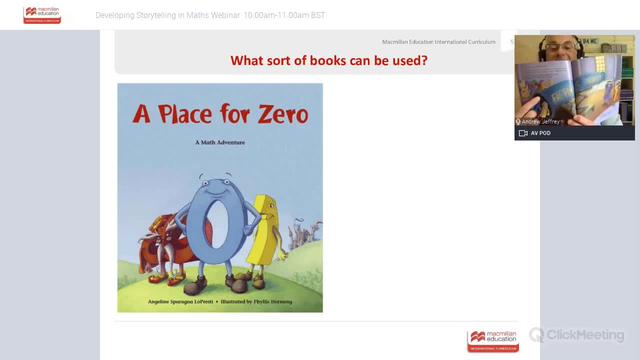 So you put three and five in and 15.. No, no, sorry, You put three and two in and six would shoot out the end. but no one had ever put zero in. So they put zero in with one and outcomes: another little zero. 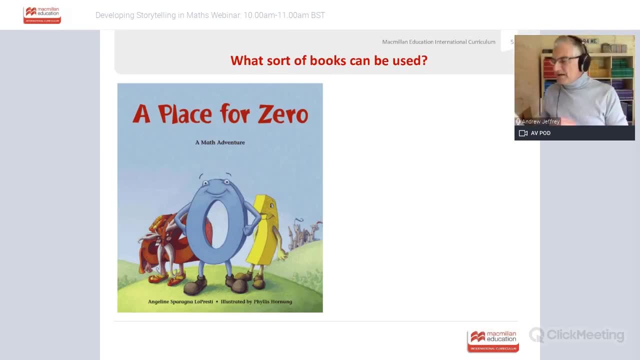 So now they've made something new and different And I love what's really going on under the surface of this book, because A place and an identity, OK, and we actually talk about place value. but I've never been a big fan of the phrase place value because I don't think the children of the age who are learning about place value, I don't think that phrase makes any sense, really does it. 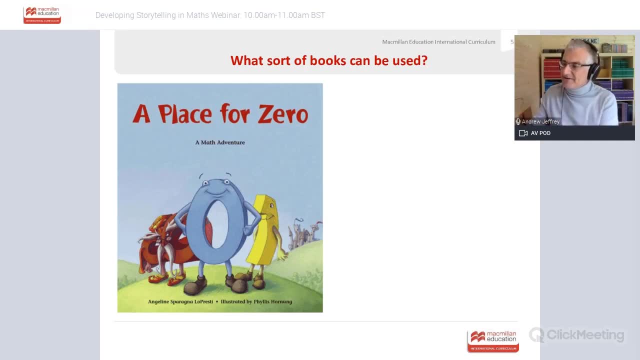 I mean, how do you relate a child to place value But zero doesn't feel valued and he doesn't have a place until Until they notice that the When zero Stood next to one and King Multiplus noticed. oh, we're not sure what happens if you get one plus nine. 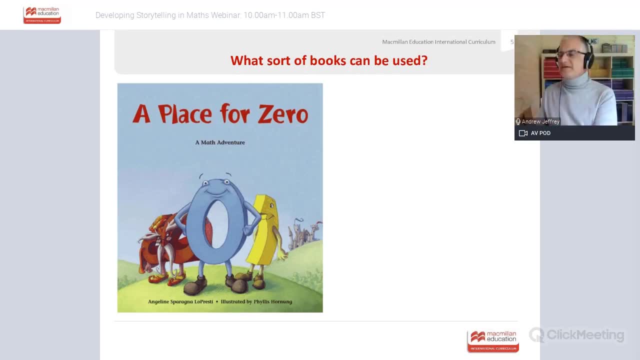 And so they decided that when zero stood next to one, that would be ten, And you can guess the rest of the story. really Suddenly, zero has an important role to play. He can make all the other numbers so much bigger. So this is a story that works for me on two really great levels. 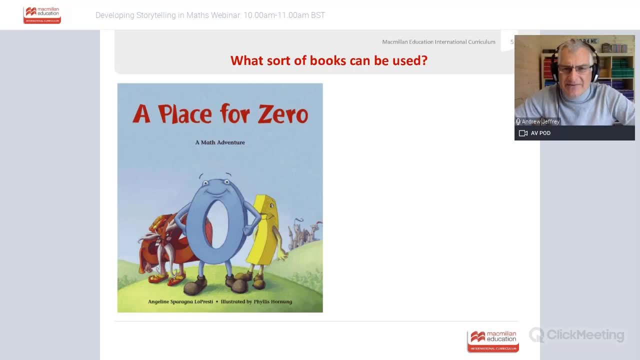 One is actually as a kind of a personal tale of you know, children need to know that they fit, They need to know that they belong, you know. so it's kind of a redemption story, for zero works very well as a metaphor. 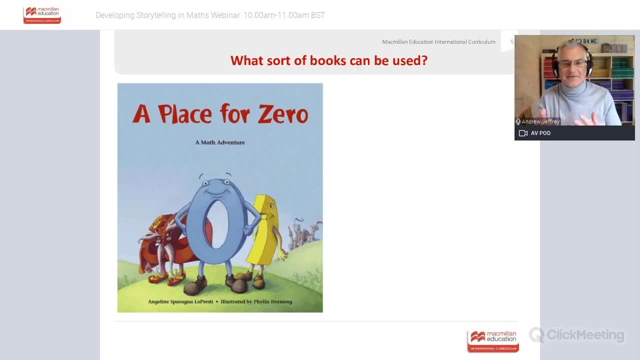 But it's also quite literal the effect that zero has on numbers, And I think I think there's a really clever idea running through this book, which is you don't need to understand everything about place value in three digit numbers to really appreciate this book. 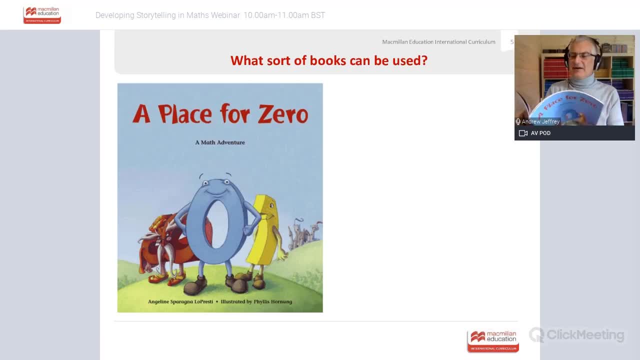 You can appreciate the book just by thinking about the clever things in it, Just by we could. we could put three numbers together. We can make thirty two threes to the next two, and the three would be ten times as much. And- and I think you can understand that even if you can't do mathematics- 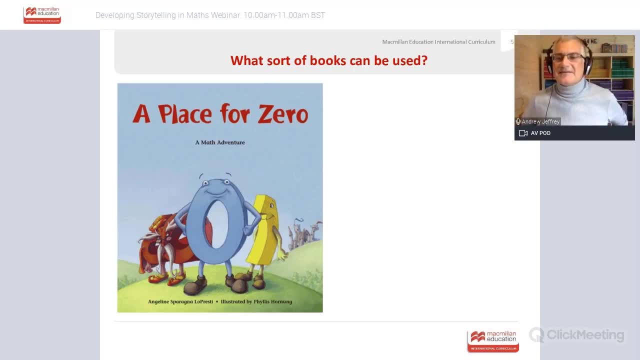 I think it's a terrific book. OK, now, someone's just quite correctly pointed out that zero is quite a new thing. We believe it was the Indians. They certainly is quite likely to have been the Indians, I think- who came up with that as a concept. 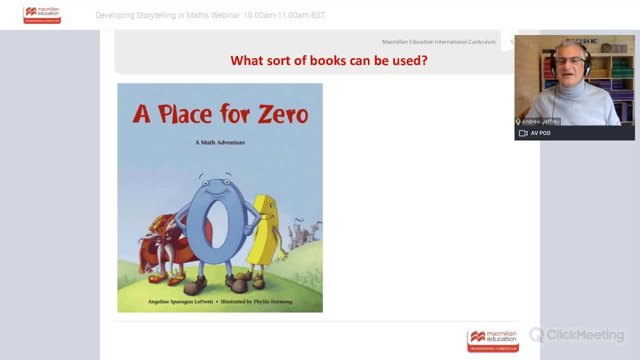 The Romans didn't have zero, And look how complicated Their number system was. So, yes, I'm thinking year three, four, I think. so I think the brilliance of this book is it can work between reception and year four OK, and not many stories can do that. 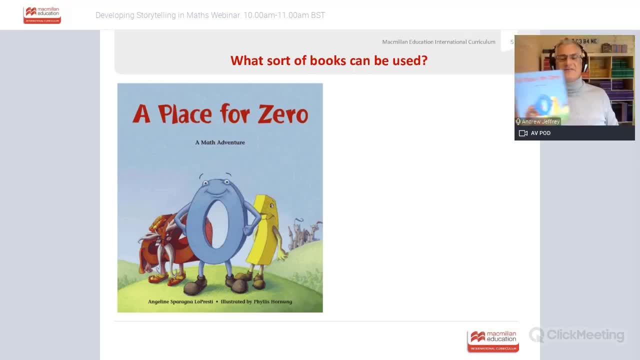 So reception can enjoy the story about: oh, that's nice, He found his place, Everyone's kind. Year four can go All right, OK. so multiplicative identities, addition, additive identities, So I think that's a really nice. 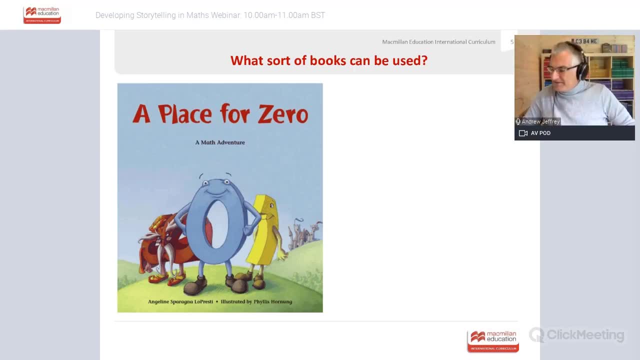 I hope you didn't mind me choosing that one to start with. A place for zero By Angelina Spadagnolo-Presti, which is a brilliant name, illustrated by Phyllis Hornung, And I think it's a really super book. 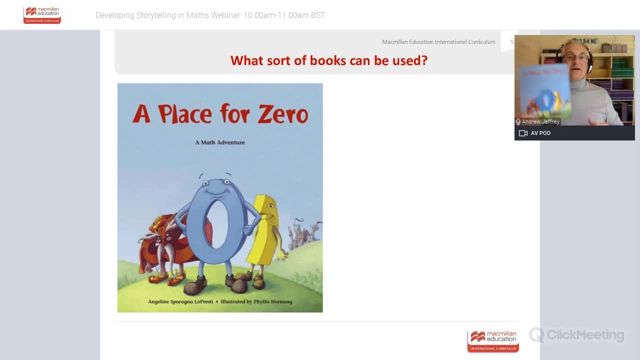 I'd say, not an expensive book, but a very, very clever story. OK, so that's one for younger children. Let's have a look at one for older children now. Now, this book, it's called A Grain, One Grain of Rice. 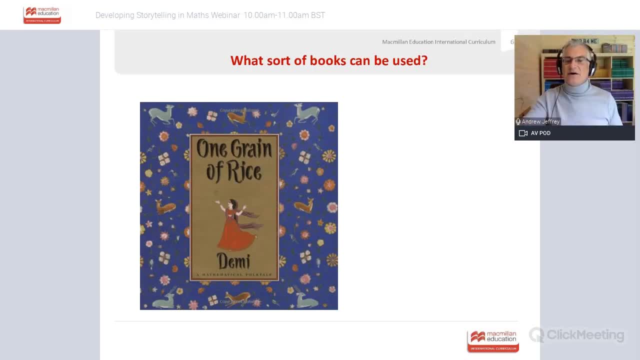 It's not so well known. Has anyone seen this One Grain of Rice? No, OK, I'm going to share One Grain of Rice with you. Oh, someone used it in year five. Excellent stuff, All right, It's a famous story. 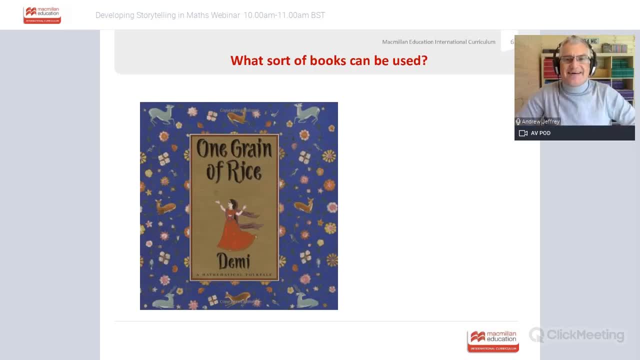 And this is just one version of the story. There are many, many incarnations of this story involving rice. So the basic, I don't have this one. I have to confess one or two of the books my wife was using with her class at school. 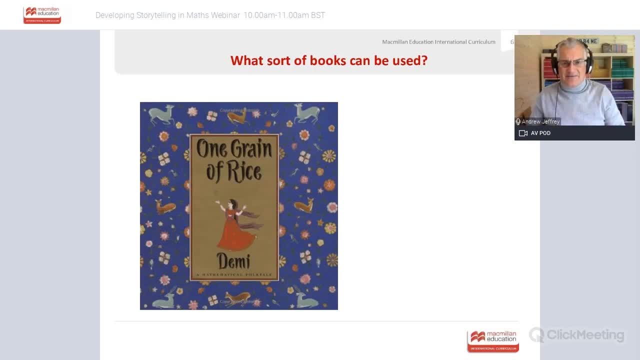 she's a teacher And when I was, I was preparing for this webinar. but she's for COVID. She's not allowed. for safety, health and safety reasons She's not allowed back into the school building. So we couldn't rescue those books back from school. 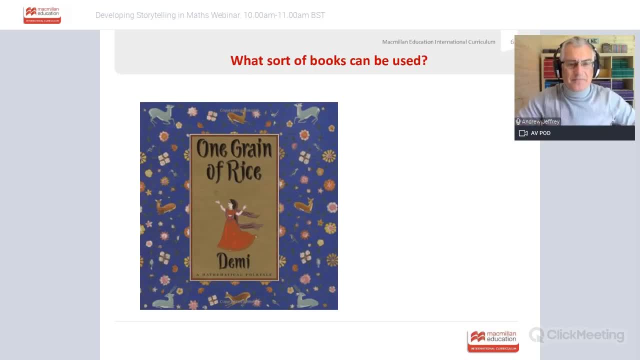 But that's OK. I've done something else for those which I'll share with you in a minute. So this is the story of a chessboard And the. there are various versions of the story, but all of them basically contain the same detail. 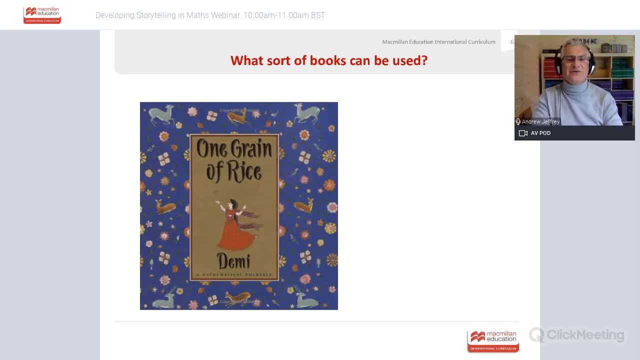 which is that the king wants to show gratitude to, in this case a girl, in other cases a man. It doesn't matter what's to show gratitude and offers. What would you like? What gift can I get you? And the answer is: I'd like a chessboard, which is obviously an eight by eight grid. 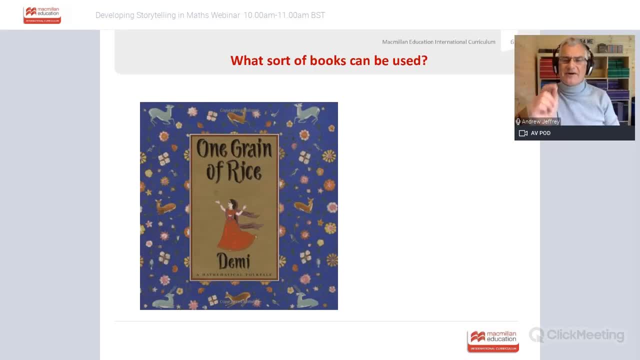 So 64 little squares And I'd like one grain of rice on the first square and then double it for the next. So two grains of rice on the next square, four grains of rice on the third square, eight grains of rice on the fourth square. 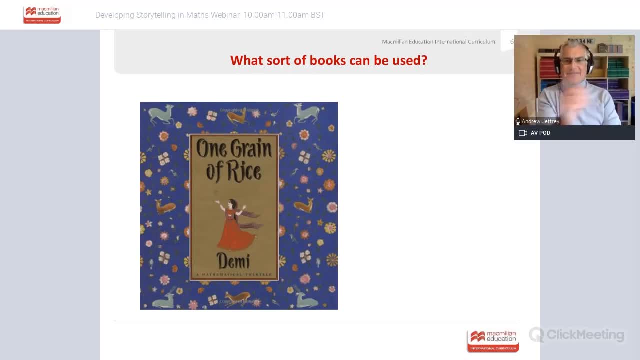 And we're sort of halfway along the top line. OK, I don't keep going till you get to the end. All right, Now I want. I want to generate a wow factor for you. So I want to do with you what I always do with children. 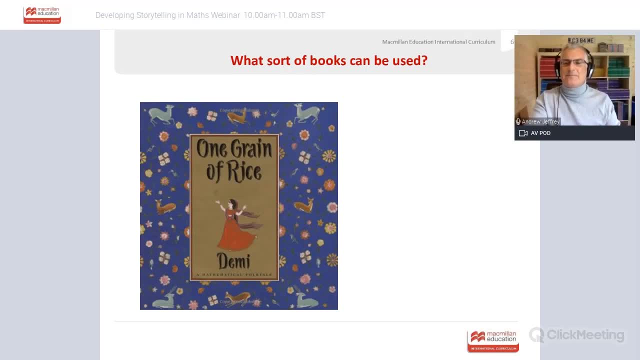 Would you write down, please, in the box, would you write down how many grains of rice you think there will be on the last square? Just have a guess, even if it's an estimate. I can see lots of people are typing. now, here we come. 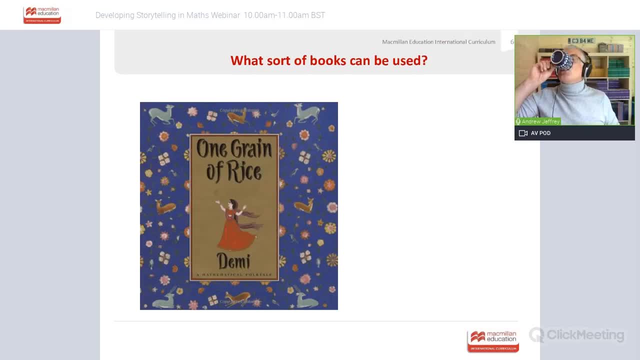 You may, You may already know, of course. OK, a mountain, a huge amount. I heard the story. Yeah, OK, ten, OK, it's impossible to give the amount of rice. No, it isn't. It isn't impossible to give the amount of rice. 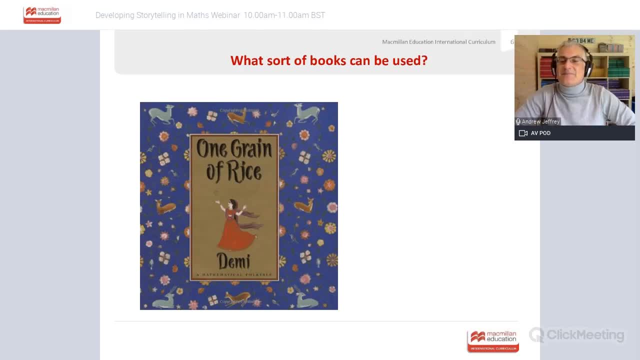 It can be worked out exactly. But actually I see the right answer from a Pambabachu: Yes, There isn't enough rice in the world to fulfill this. You cannot, And it's an extraordinarily big number. It doesn't feel that way because you go. what the top row is? one, two, four, eight, 16,, 32,, 64,, 128.. 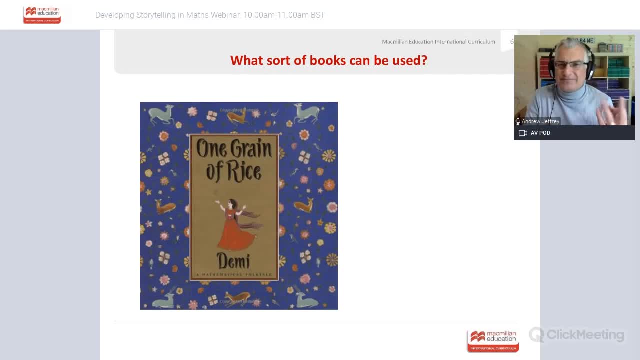 So 128 grains of rice, That's less than a portion, Yeah, that's less than one portion of rice. Hundred and twenty eight grains. It's not, it's not Fibonacci, actually. No, it's not, It's so. it's called the exponential. 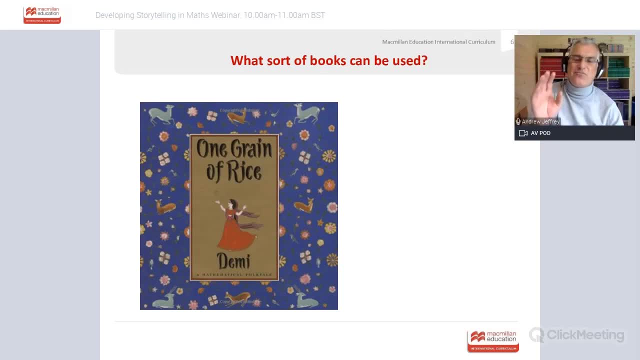 Exponential is the powers of two. So two to the power of one on the second square, two to the power of two on the third square, and so on. But two to the power of 63 is so many trillion grains of rice. There just isn't enough rice in the known universe. 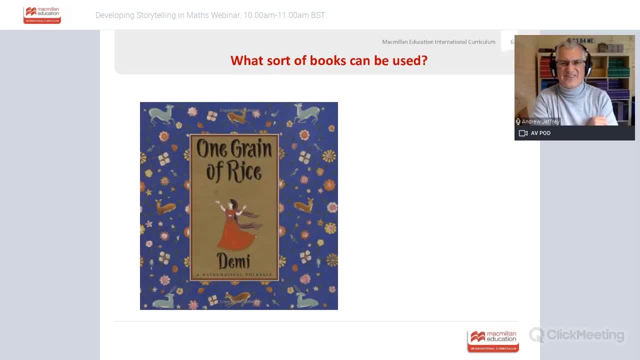 OK, and- and this is such a shock to people- like it's just a 64 squares, Right, But it is an absolutely phenomenal thing. And to think that there's not enough, Oh, there you go. Look one billion, says Elizabeth. I haven't worked that out. I could be right. If you type two to the power of 63 on your calculator, it will give you the answer. That could well be it. I'm just going to believe you. Oh no, that's an odd number. 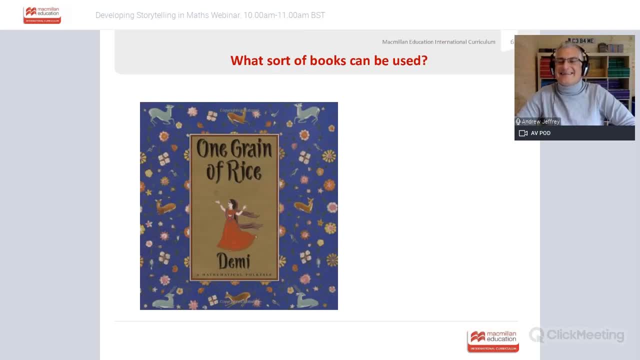 It definitely isn't an odd number, but it could guess it's. it's phenomenally huge And the power of doubling up, And of course the king realizes how wise the person has been and how unwise the king has been. Sometimes I've heard a version of the story where the king says to his children: how much do you want? 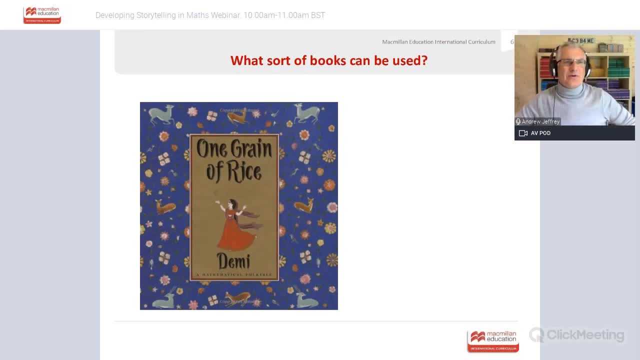 How much do you want? How much do you want lungs? How much do you want? Sometimes everyone is. You know it can't be another past now. like: o're you angry with me? You've got It's one of those things. so I'm just going to let you know how active that is. 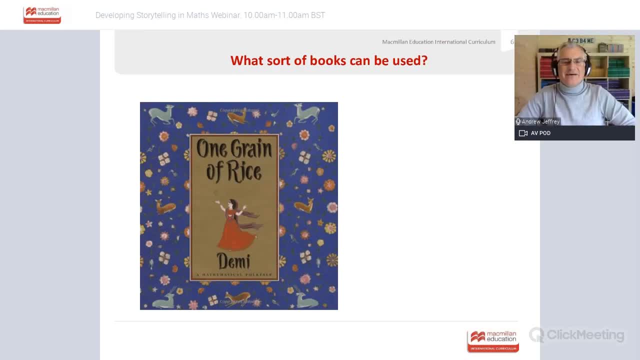 love me and one of the doses. I love you more than salt. No one of the courses I love you more than salt. And that's not a very well received after a, but then they start doing it with salt. That's not a very well received after a, but then they start doing it with salt. want to add, if you? 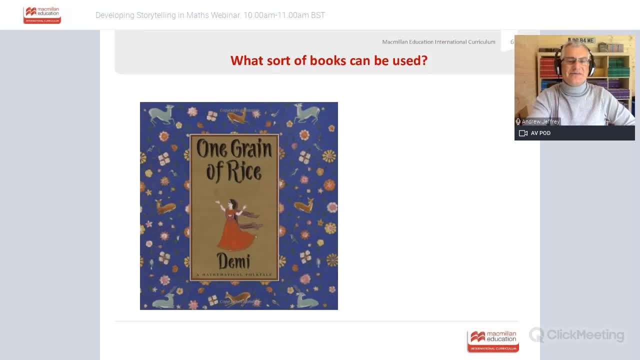 And if you, Oh, someone says Sarah says: correctly pointed out Up, campus correction: rightly pointed out. Thank you, Sarah. yeah, Up, it actually shows you the numbers. I didn't want to do a spoiler, obviously for this, but it actually shows his numbers 1 to 4816, 32 and them. 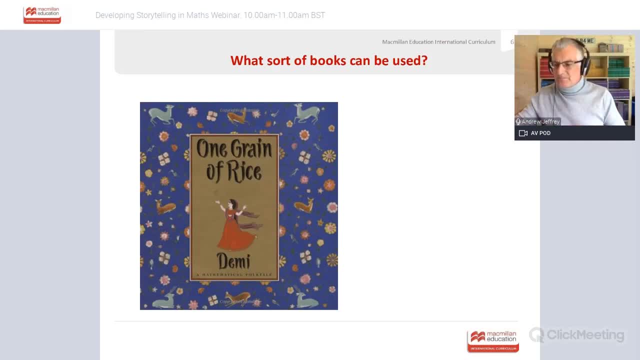 on. excuse me, excuse me, sorry, a bit more my drink. ah, i do beg your pardon. right um one other fantastic idea for this. this makes a superb assembly because it has that real wow factor in primary or secondary. it makes the lovely assembly um something else that you could do. 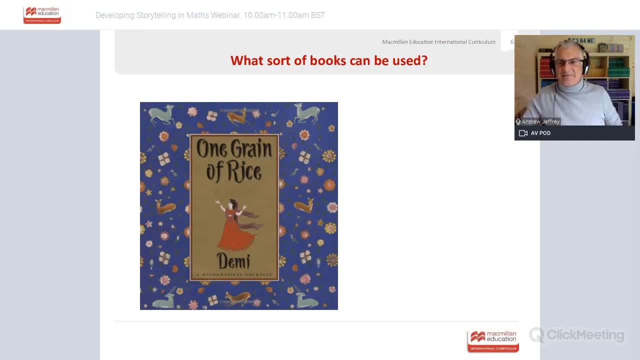 years ago- and you can probably find it on my youtube channel if you search andrew jeffrey maths on youtube- i made um with my kids, who are much older now and slightly embarrassed by this video. i made a video about pocket money where um one of my children said: can i have 10 pounds a? 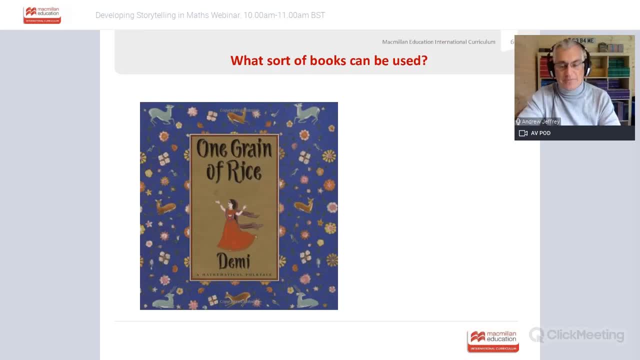 day or something. another one said: can i have 1p on the first day, 2p on the second day, 4p on the third day, 8p on the fourth day, and so on? um and uh, and i sort of posed the challenge, like you know. 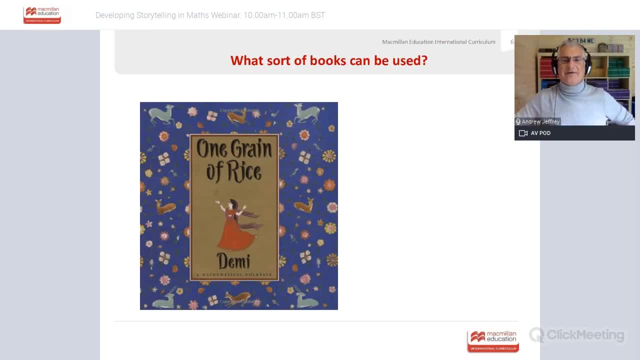 who's who's going to get more money. well, it turns out you've become that, with 1p, 2p, 4p, 8p, you are a millionaire before the end of the month, which is quite extraordinary. um and uh, in a couple of months you become, um, a multi, multi-millionaire. so, uh, all that by the end. 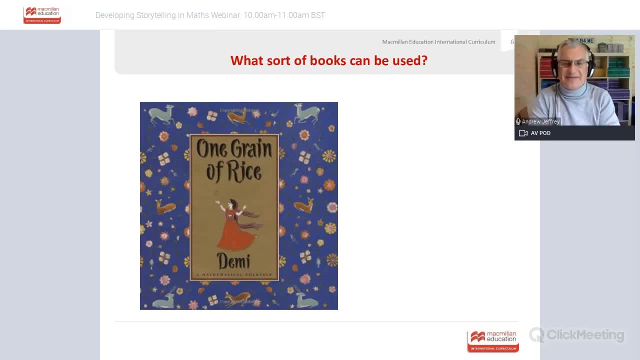 of by january, the 31st, that have a look on youtube. i've done a video on it anyway and it's a super idea and and it really does show you the wow factor of numbers and sometimes, i think, wow factors, for you know, it's just like it's too ah, just mundane. you know, do this calculation now, do this. 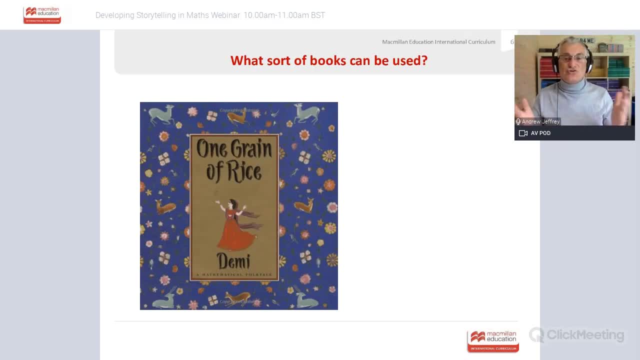 calculation. now do this one, but that's just just the simple times two, which i have to say as a little aside. multiplying and dividing by two is one of the most important things i think children can do. or 10, um, i think if you can do that mentally, you're well on your way to be able to catch lots. 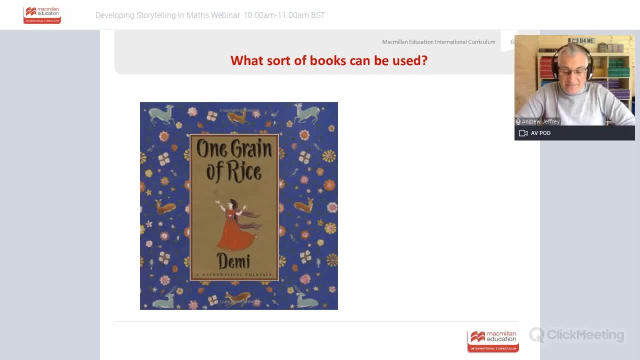 of things, so, um, mental arithmetic things. so from that point of view it's good and just imagine that kind of that amount of calculation. so i can really really recommend, uh, one grain of rice, or sometimes it's called salt, but any. this is just one. i like the cover of, actually, but any version. 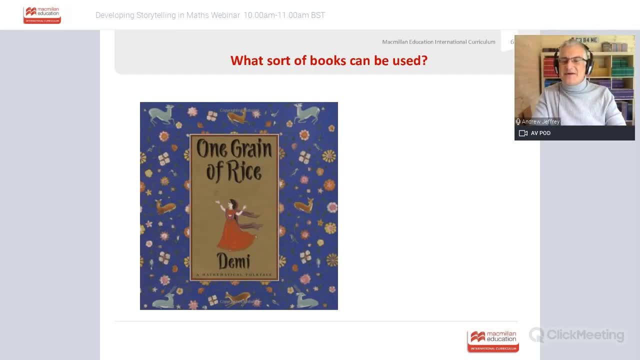 of this story is a superb story. i like what sarah's just put. let children adjust their estimates as they go along, because you can't begin to estimate- um, you can't begin to estimate sensibly what two to the power of 63 is. uh, it's just a fantastic number, and also from right, from very young. 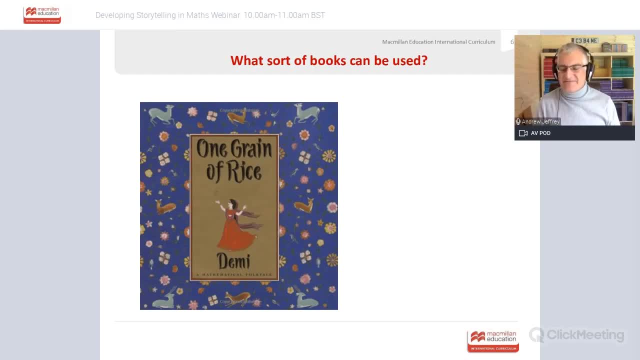 children love massive numbers, don't you notice? like so when they're. when they're small, they think that 10 is the biggest number in the world, and that's mainly because of the stories that we teach kindergarten children, isn't it, where almost every story seems to have the numbers from one to five? 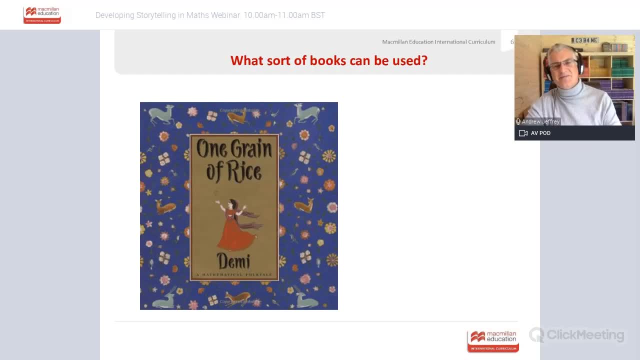 or one to ten, in order. and then songs: five little ducks went swimming one day, ten sausages sizzling in a pan, ten green bottles, so many, uh, of the songs that we teach young, young children. um are, or the stories are quite rightly contain those numbers either. 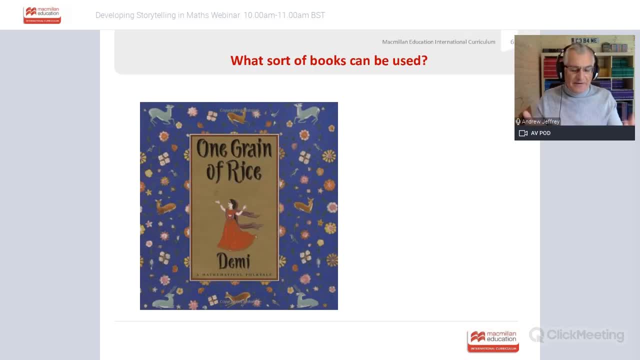 on or back, and that's to familiarize themselves. but the song itself, the sound of the number and the way you write the number, neither of those are the number. so so to start with they think, oh, ten is the biggest number. then they realize they're wrong. okay, they realize that actually. 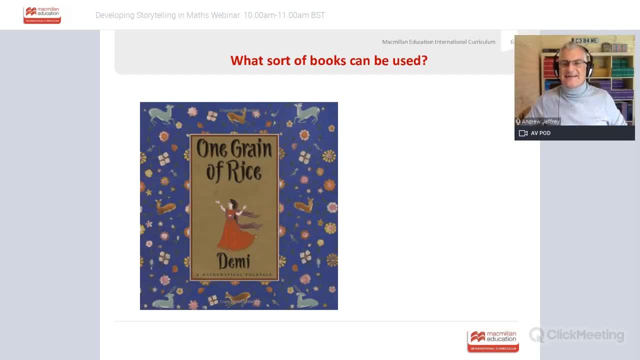 20 is the biggest and and then they get obsessed and uh, i love that. brenda said: yeah, they, they've gone on to a hundred. the hundred is a massive and they love it huge number. um, then by the time they're kind of seven, eight, they've decided that a million. 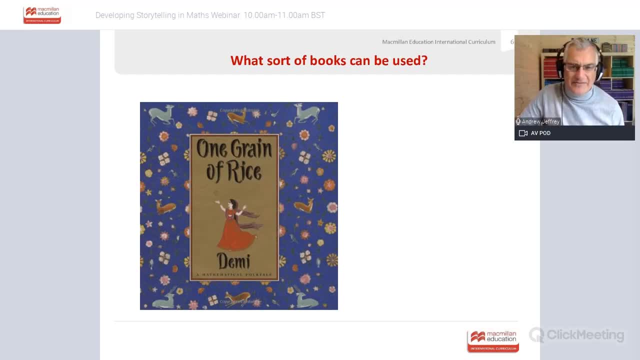 is the biggest number, and and then they come up with various versions depending on what they've heard. and then, when they're about nine, the children often like to tell me that infinity is the biggest number in the world, right, which is funny, because it's not even a number. but let's not 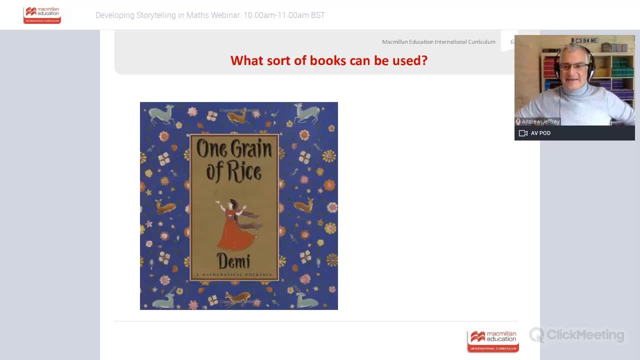 go there. okay, uh, it's certainly not the biggest number in the world and uh, and then i just kind of love this idea that numbers are so fascinating and they, they just will love this story. okay, they love this story. so, um, yeah, i love. i love that friend. i used to say uh to my kids. what's the? 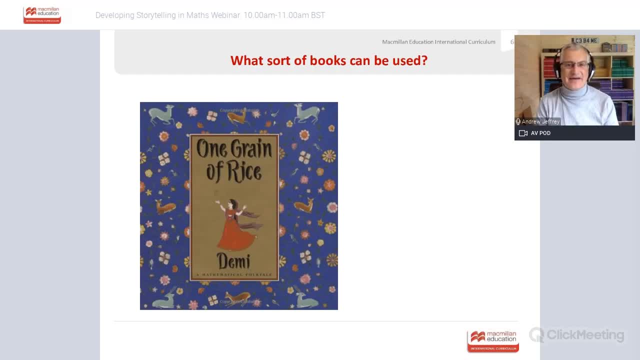 biggest number in the world, and they'd say something like 113, like what happens if you add one, and i'd get a couple of minutes of silence. it was quite nice. okay, right, talking of one, uh, talking about adding one, here is uh a brilliant book next. okay, this is an absolutely stunning book. 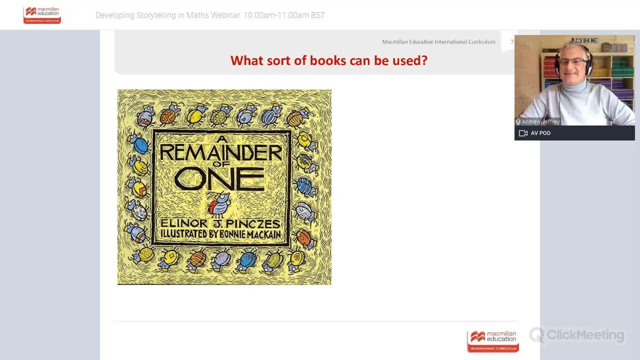 it's called a remainder of one. now, who has done this? has anyone seen this book before? this is? i think this is the first book i saw that's mathematically brilliant. um, that was specifically designed. no, no one's seen this. okay, well, again, this is one of the 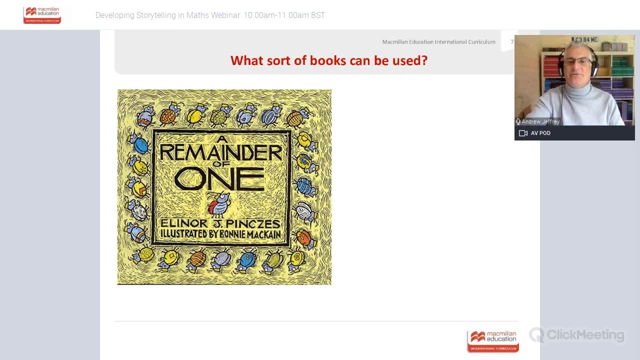 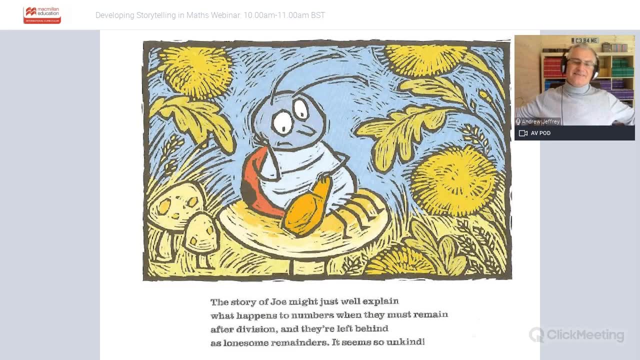 ones that i'm afraid i couldn't get hold of um for this webinar. so, because i've got your back, folks, uh, i've got screenshots of all the pages. yeah, okay, um right, i'm gonna read it out to you. um, not every single page, but enough for you to get the detail. and i want you to think about how much brilliant. 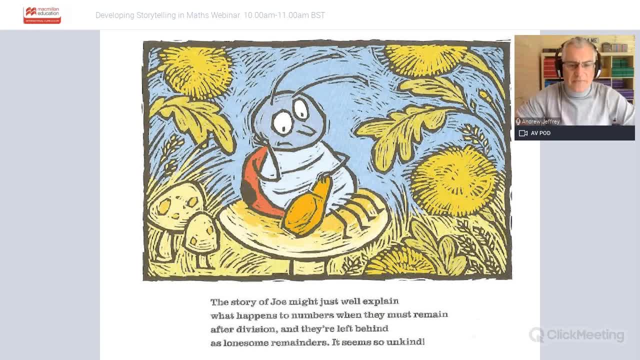 mathematics. you can get from this, uh in a lesson. so um, the, the illustrations and the mathematical ideas, i have to be honest, are a lot better than the slightly iffy poetry, but it works well enough. the story of joe might just well explain what happens to numbers when they must remain. 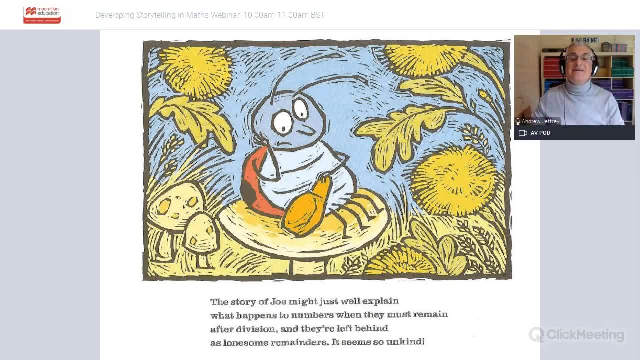 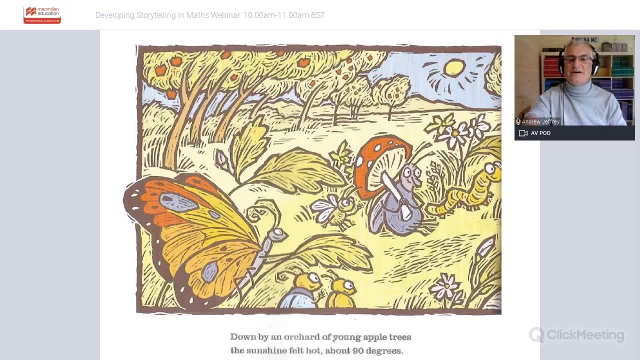 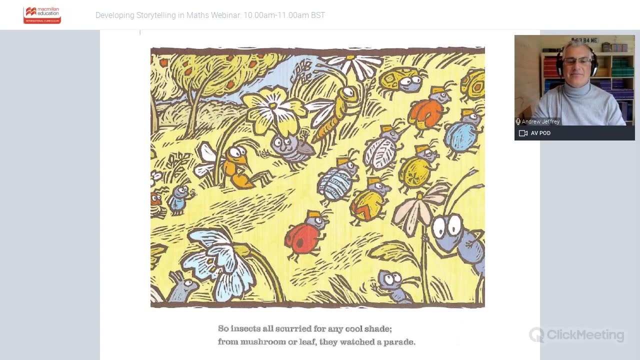 after division and they're left behind as lonesome remainders, it seems so unkind. did warn you about the poetry down by an orchard of young apple trees. the sunshine felt hot about 90 degrees, so insects all scurried for any cool shade from mushroom or leaf. they watched a parade. 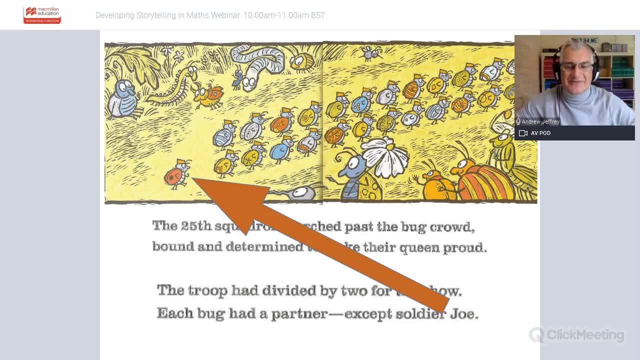 the 20. no, sorry about this dirty gray arrow. this is because, um, the software we're using, click meeting- didn't really like showing my powerpoint, so we've had to have my powerpoint, uh, with all the animations built in, which means there's a huge great. 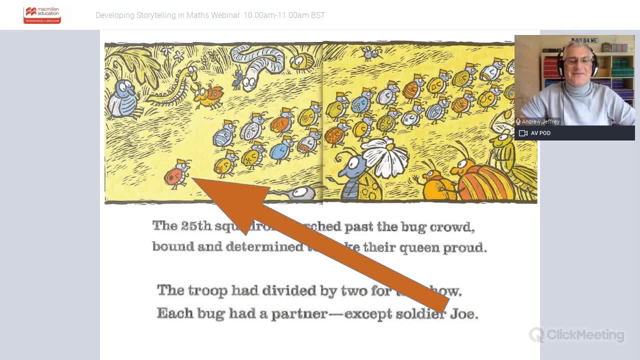 arrow across the text, but i'll try to remember what it said for you. the 25th squadron marched past the bug, crowd bound and determined to make their queen proud. the troop had divided by two for the show. each bug had a partner, except soldier joe, at which point the arrow was supposed to. 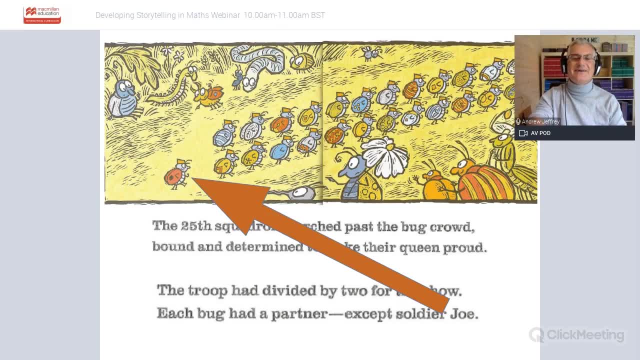 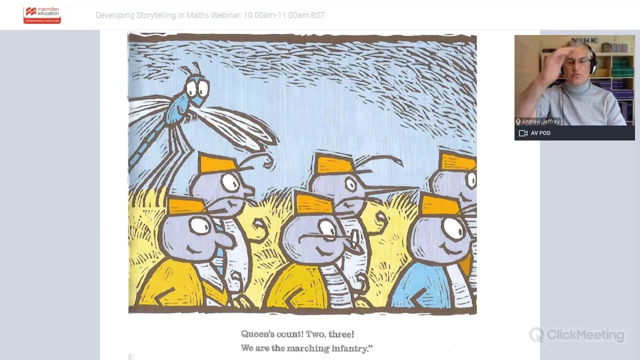 dramatically fly in. but there you go. so joe's on his own at the back. okay, at this point, uh, the idea of the 25th squadron is quite is quite an interesting, uh clever idea. all right, now let's see what happens. queen's count: two, three, we are the marching infantry. two, three, four, we're in the. 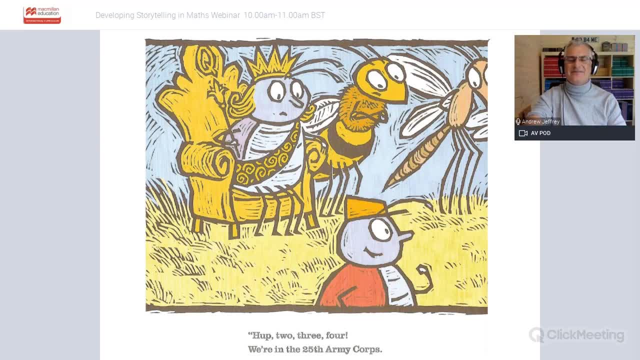 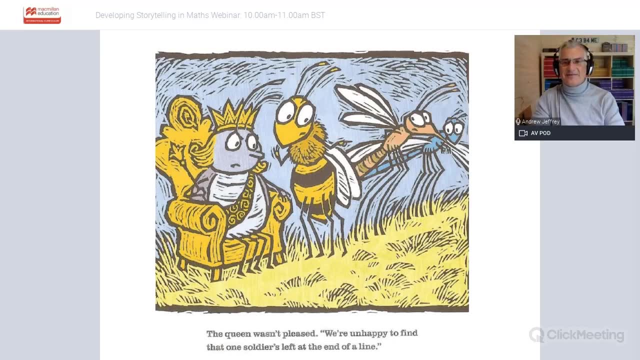 25th army core. and then you see there the queen looking at joe, who's, at this stage, fairly unaware that he's being observed by the queen. the queen wasn't pleased- we're unhappy- to find that one soldiers left at the end of a line. she didn't like that. 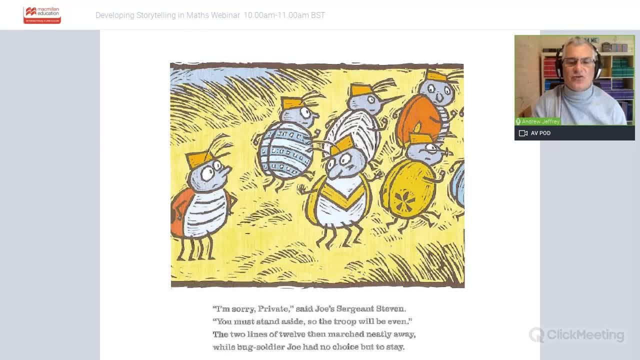 well, i'm sorry, private, said joe. sergeant steven, you must stand aside, so the troop will be even. the two lines of 12 then marched neatly away, while bug soldier joe had no choice but to stay. oh, okay, no, i've skipped a bit, sorry, okay. um a honeybee hovered above lone joe's head, the queen. 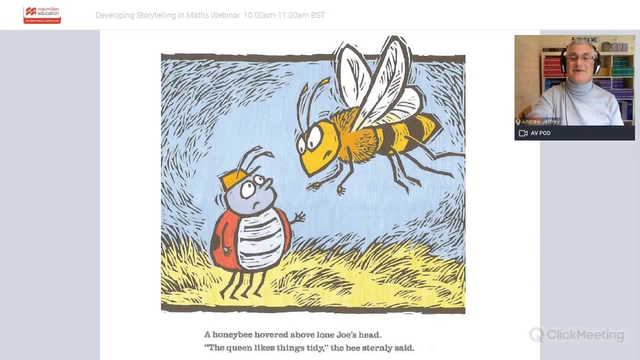 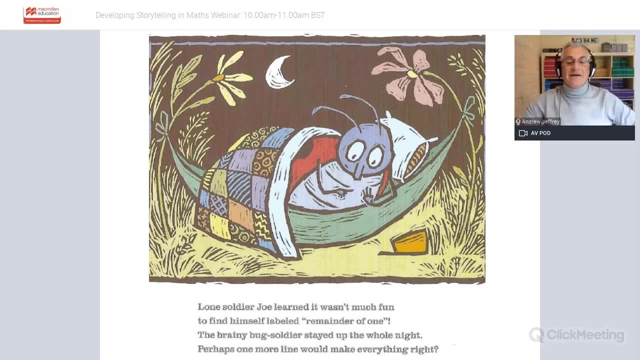 likes things tidy. the bee sternly said: oh dear, been told off. lone soldier joe learned it wasn't enough to find himself labeled remainder of one. now, at this point, i i want to share an idea with you. can you remember at school being the one that wasn't picked when the teacher says: get into pairs. 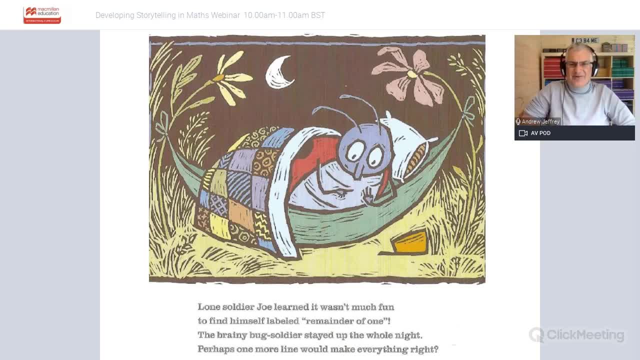 find a partner and nobody wants to be your partner, or you haven't paired up quickly enough, and it's a kind of a sad feeling, and so this is tapping into what children already understand. okay, so children understand this idea and i i think children get right behind. joe, you know, if you 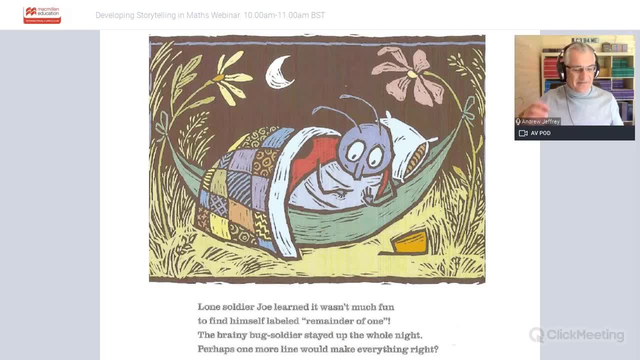 weren't very good at something, you wouldn't have been able to do it. if you weren't very good at something, you wouldn't have been able to do it. if you weren't very good at something, you wouldn't have sport or something and you were the that, that dreadful thing where the captains get to pick. 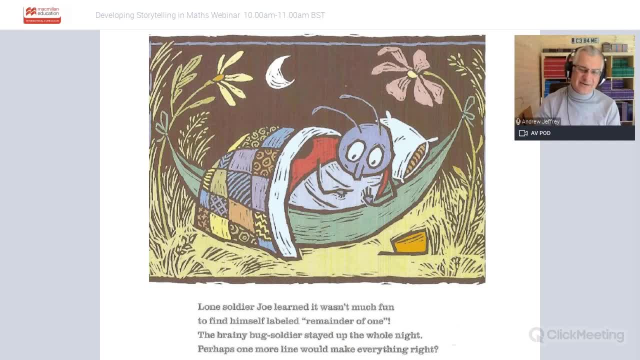 teams that we used to do- and i don't want to be the last one, i don't want to be in this team, or i don't want to be your partner, and there's always somebody left or two people left who won't pair up because they don't like each other, and this is kind of real life of school. so i think 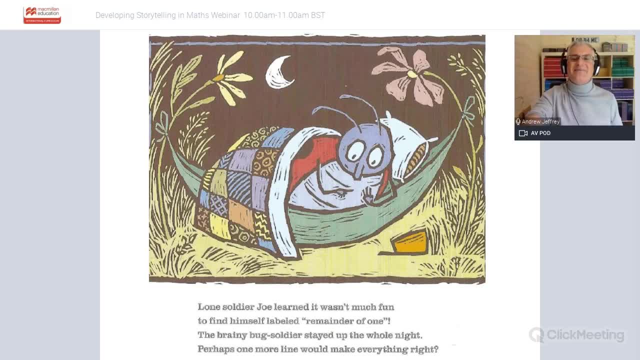 i think children can really relate to poor old joe. you know, they don't realize they're doing any maths yet, which is very clever. the brainy bug soldiers stayed up the whole night. perhaps one more line would make everything right. maybe let's see what happens if. 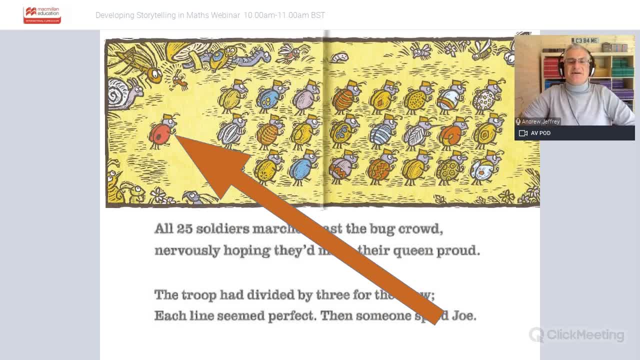 they put one more line. in all, 25 soldiers march past the bug crowd nervously hoping they'd make their queen proud. the troop had divided by three for the show. each line seemed perfect. then someone spied joe, oh dear. up. two, three, four, we're the 25th army corps, queen's. 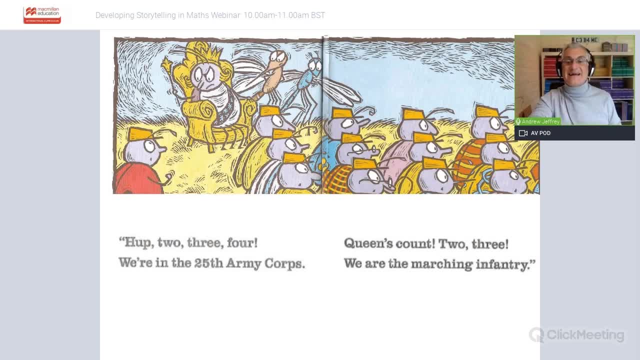 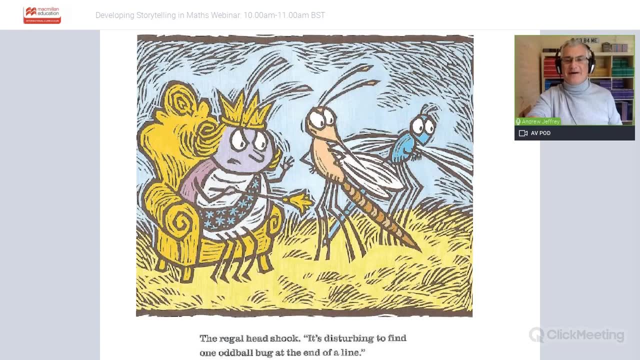 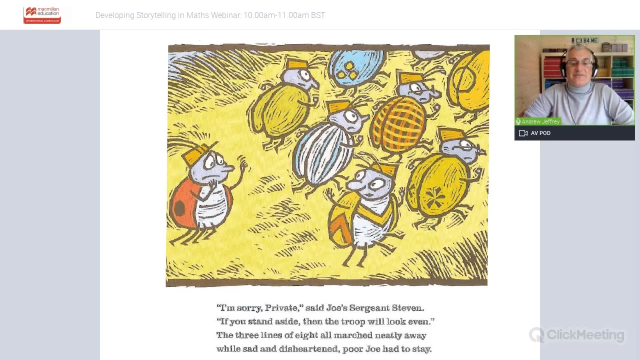 count two, three. we're the marching infantry there. she is glaring at him. i love this so funny. the regal head shook. it's disturbing to find one oddball bug at the end of the line. i'm sorry, private said joe sergeant. stephen, if you stand aside, the troop will look even. 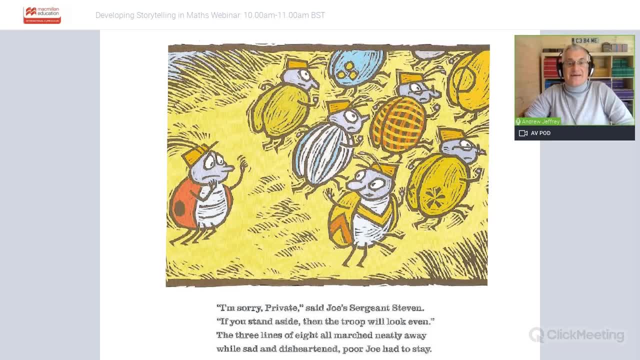 the three lines of eight all march neatly away while sad and disheartened poor joe had to say: now the really kind of switched on kids would realize that the 25th army corps had 25 members in, because it does give you clues, doesn't? it talks about the 212s, the 3, 8s. 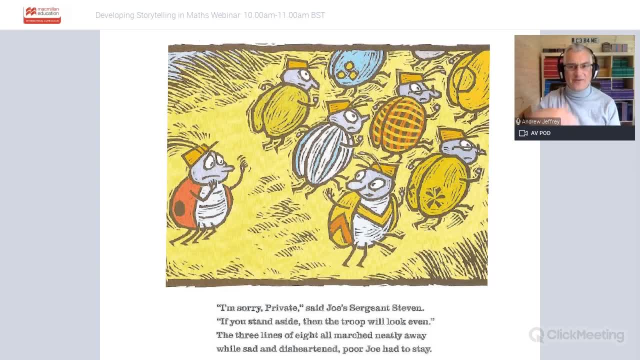 okay, now i won't read the whole story to you, but i'm going to read it to you because by now you're beginning to see the pattern, and the pattern and the repetition and the predictability are really important in stories. that's why we're going on a. 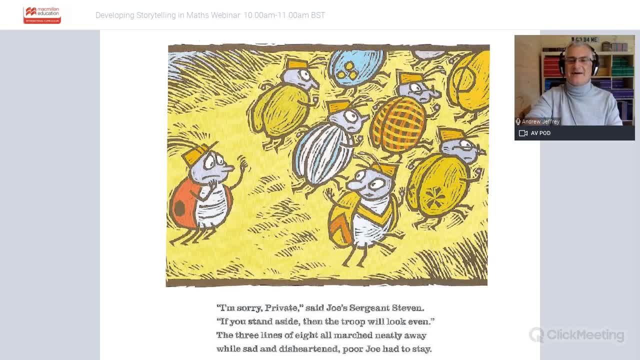 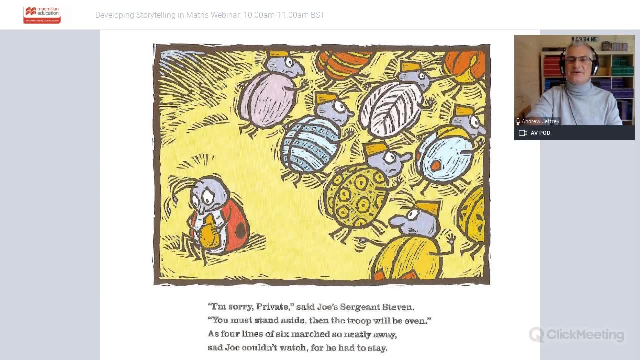 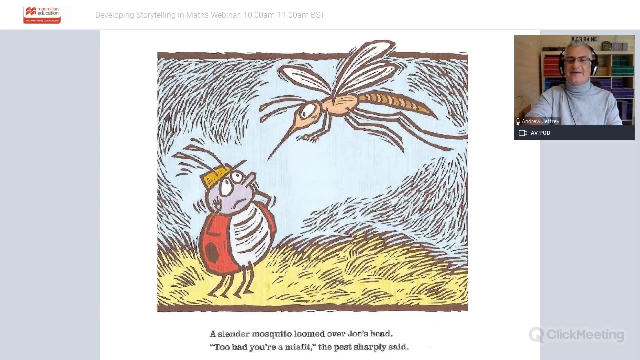 bear hunt is such a popular book and this repeats again, so i'm sure you can guess what happens. uh, queen has a look, um, he gets sent away, um, he gets told off by some. a different bug, okay, uh, no, it's this one. okay, uh, and then um, 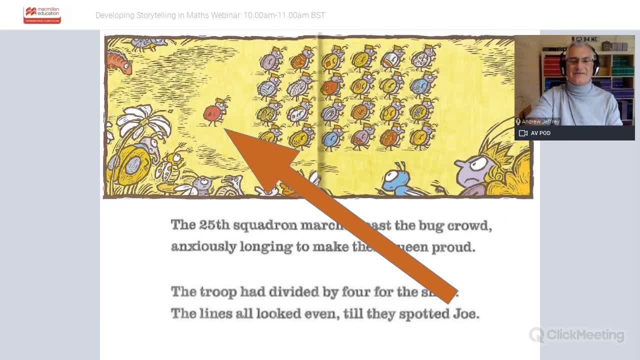 he gets sent away. um, he gets told off by some a different bug. okay, uh, no, he gets told off by some a different bug. okay, uh, no, he gets told off by some a different bug. okay, uh, no, he gets told off by some usual things. six lines of four, then joe at the back queen looking grumpy. so very predictable and safe. 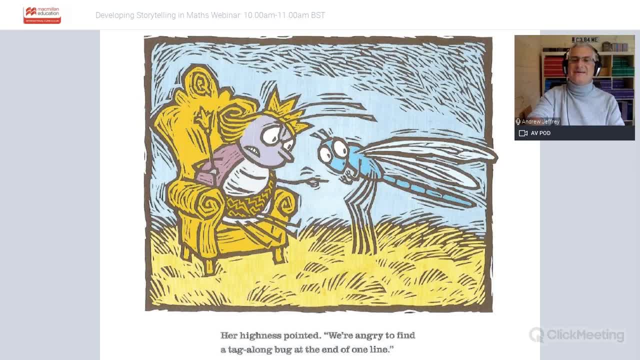 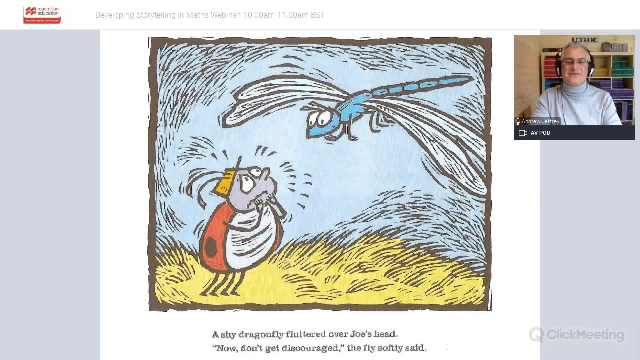 environment for children. okay, uh, queen expresses her displeasure, sergeant says you can't play. and then i kind of like this. i missed this until this morning. a shy dragonfly fluttered over joe's head- though don't get discouraged. the fly softly said: um, i've never noticed that. uh, and, and then 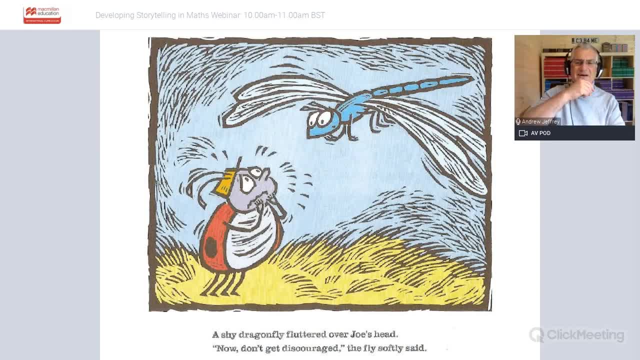 it's going to work out. you're probably ahead of the book. you know we're going to get into rows of five, but sometimes a little word of encouragement is is what it takes, and i thought that's just a clever, clever twist in the story that i'd never picked up before. so he goes to bed and goes okay. 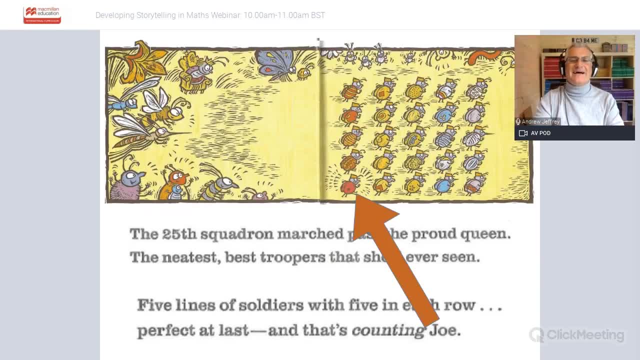 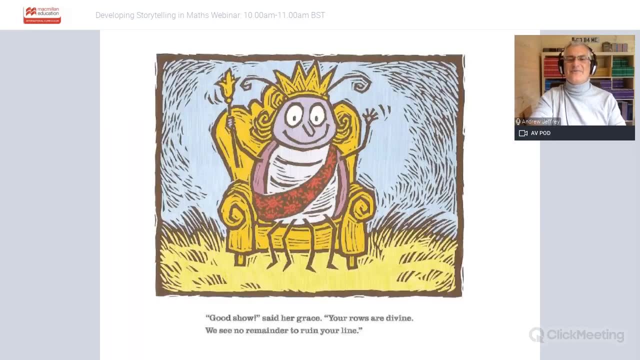 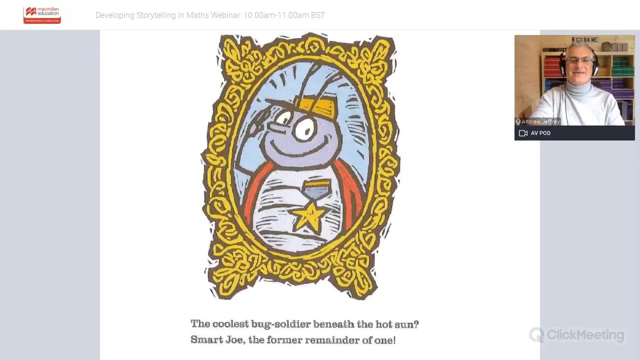 we'll try lines of five and then, of course, aha, there we go, there's joe. but now look, five lines of five. everyone's in a line, everyone's happy, the queen is happy. um, there we go. joe is happy because- and what a great story. and i, i think that's a smart joke. there we go, i think that's a. 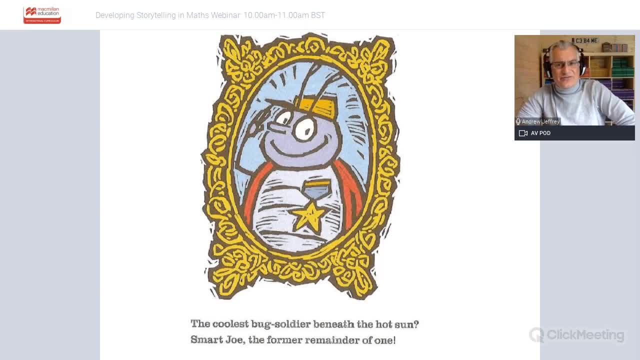 tremendous story um. a is very clever. b- it addresses human emotion. c- it addresses the biggest need that we all have, um, the biggest need that we all have, which is to matter, to fit in, to belong somewhere right, um, to find our tribe, to put it in a more modern way. and so i think that's. 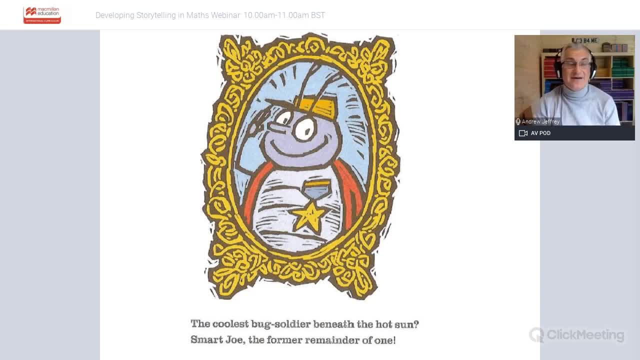 absolutely genius. and what a wonderful way to talk about division and remainders. okay, because division and remainders can be quite a dry uh story. but as soon as i saw this i thought that is a very clever idea. so i didn't mean to say dry story, i meant to say dry topic. 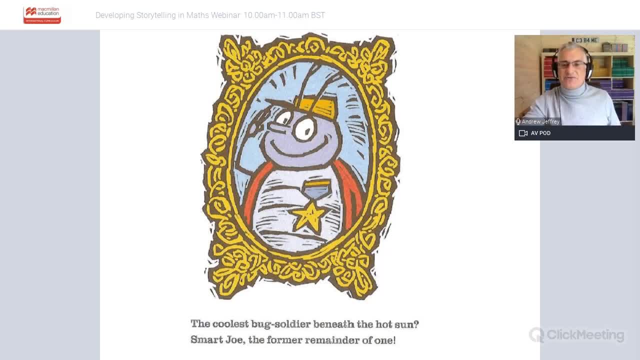 but i thought that's a very clever idea. now, what you would do with this, what you would do with this is you wouldn't just read the story, because the stories are lovely, but this is about. this is a webinar about maths. you would give them 25 counters, or 25 coins, or, uh, 25. 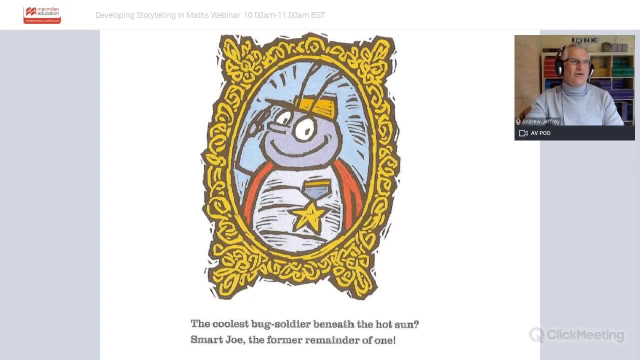 little cubes, maybe linking cubes, whatever, and and you'd say, can you, can you make? can you tell the story to your friend by using the cubes? or what if they were? how many people are there in this class? let's have a cube each and see what we can make. so you start to build the idea of an array, and an array is one of the truly big ideas. 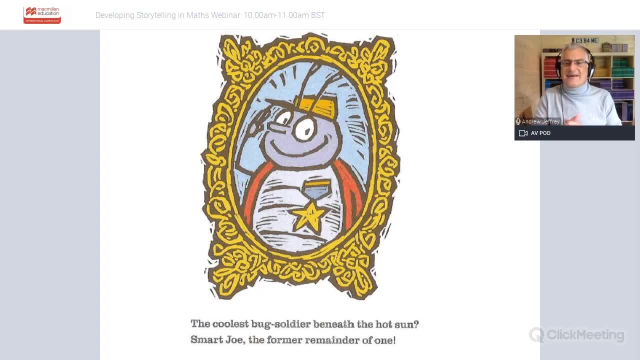 of mathematics, isn't it? multiplication and division? okay, terrific thing to to think about. so, um, you could then say: with other numbers, all right. so you guys, why don't you take, uh, 15 to 15 encounters and see if you can make there be one odd man out, or two odd people out, or three odd? 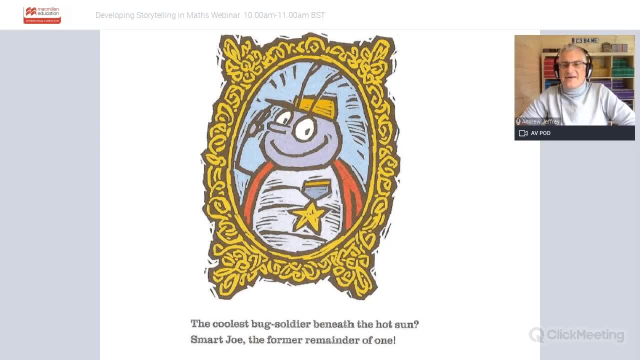 people out, you know, see if you can have joke and have a friend or or create your others, um, so you could really have i mean this. this links to- i've seen someone said it links to art and drama. yes, it does. it links to pshe, doesn't it? it links to pe: get into teams and groups. um, it's such a genius. 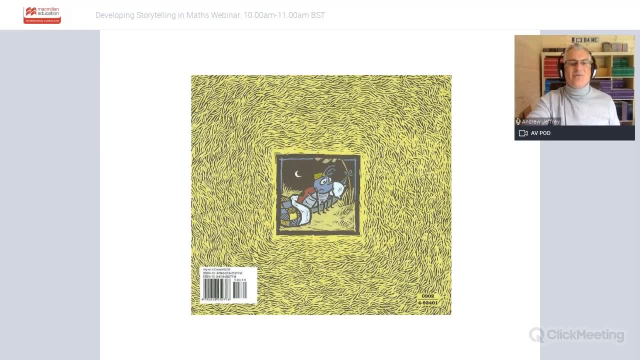 book. so, uh, there it is. it's called a remainder of one. i absolutely adore a remainder of one, i think. i think, as i may have said this before, it's what got me into thinking that maths lessons could be stories. okay, i want to move on to a slightly different type of book now. this is this book. 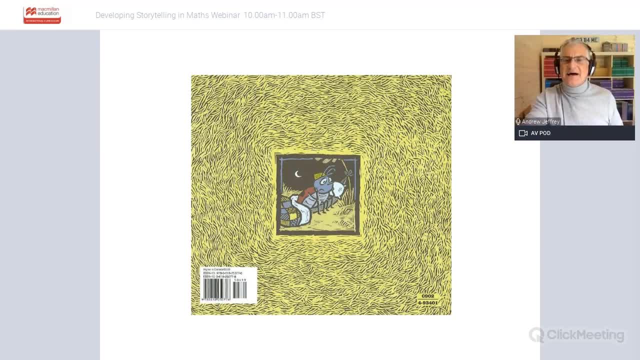 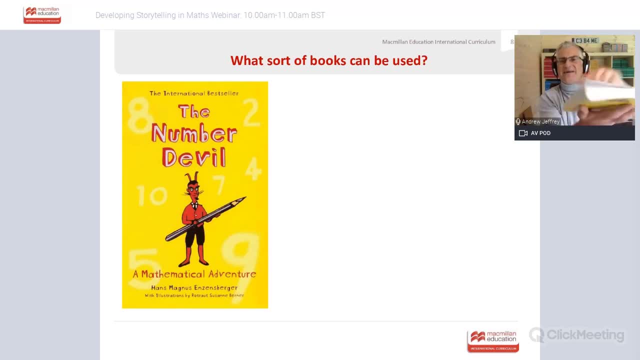 is the odd one out, okay, um, and it's the odd one out in my list because it is quite a thick book here. it is okay and it's quite a. it's not like a, although there are pictures in it. you certainly wouldn't call it an actual picture, but you can see. you know, this is not a book you want to be, uh, just giving a. 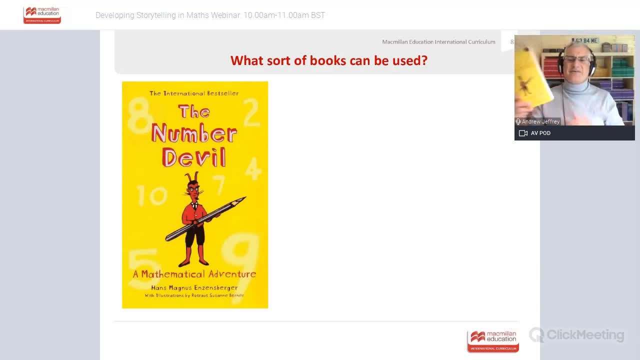 seven-year-old, uh, to read or whatever. um, i i would say i pitched this at 10 to 13 year olds probably, maybe maybe 14, i don't know. i mean, don't get me wrong, it does have pictures. this is the story of the bonacci and the rabbits. okay, there's another one about pascal's triangle. 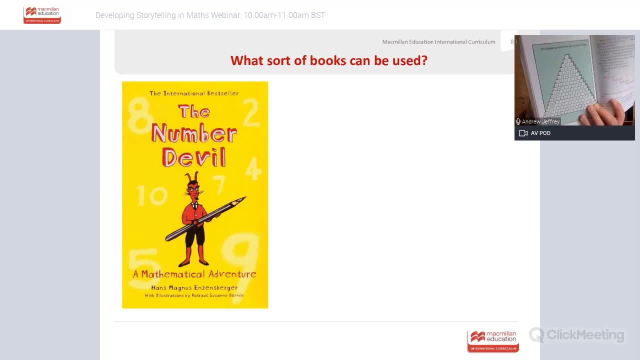 okay, how you. and this is a good example, because basically the number devil very clear. it's been translated into english. it was, uh, uh, hans magnus edson burger wrote this and it was translated into english. he's a german and it's a. it's a superb story and it's a. again, it's some good psychology. 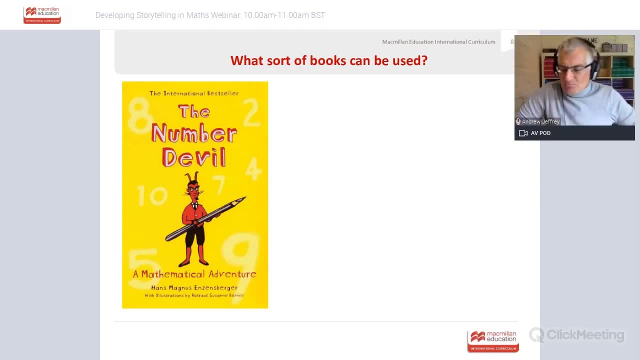 so what happens is there's a boy, um, who, uh, is in bed one night and he has a dream that this number devil comes to him and he hates math. this boy really hates math. he hates his math teacher. uh, uh, who's painted in a stereotypically not great way, to be honest, and um, and then the number. 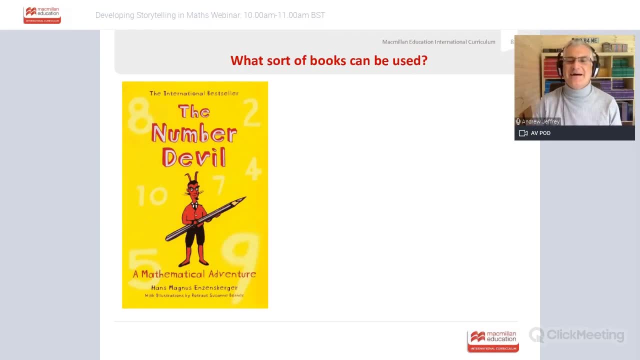 devil says: what do you mean? you hate math. numbers are great. and he takes him on this journey where he says: uh, he starts with one. he says: all you really need is one. everything comes from one. and then you build it up. and the boy: i mean: it's a very predictable journey, but it's a the boy's. 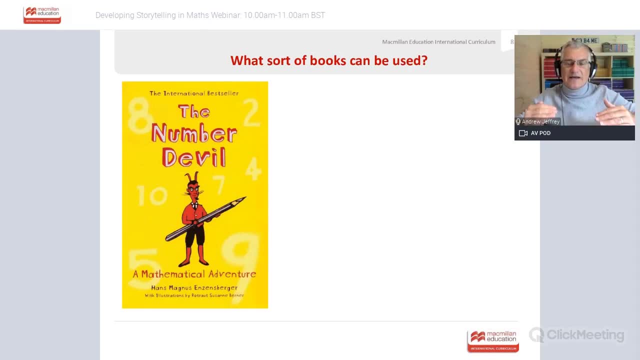 attitude slowly changes and his resistance slowly falls away. um, as he learns about the amazing patterns in mathematics and it's really uh. and then, and then, finally, at the end- spoiler alert- he's given a question by his math teacher in class and he smashes it before anybody else, basically, so, so for he goes from being 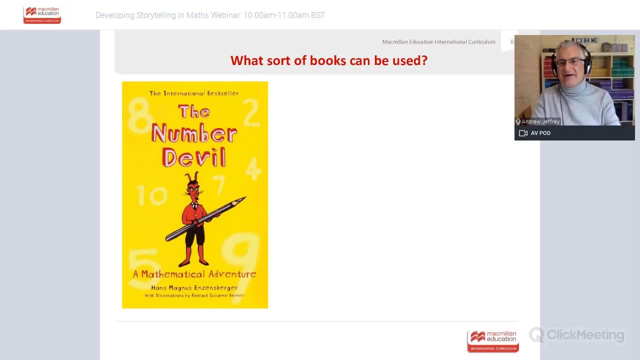 you know not very good, or thinking he's not very good, to actually really quite enjoying it and and seeing visualizing mathematics. um, it's a superb story. i mean it's the language is good, uh, it's well written. uh, considering it's a translation, i mean they talk about, uh, combination. 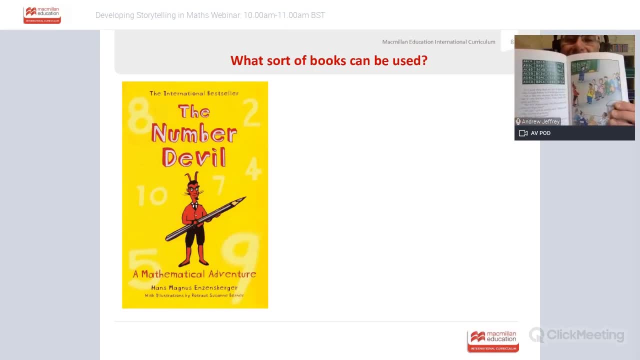 of rhetorics and permutations by literally thinking about the different ways the kids could come in and sit down and it's. it's that, it's all practical stuff. um, there's uh graph theories, you know really accessible things um fibonacci sequence, um the handshake problem done as a node. 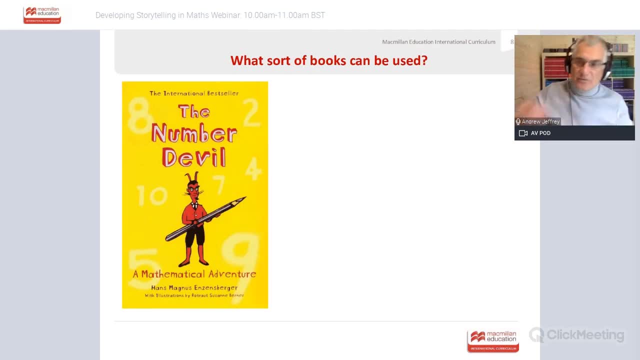 uh and uh, vertices problem, vertex problem. so quite, quite big ideas in math, but in a really simple way. they use fun language. that's a very unusual book. i enjoyed reading that myself as an adult because i think it gave me nice ways to teach us. okay, um, nice ways for for me to teach uh others, sorry, to teach children, and so. 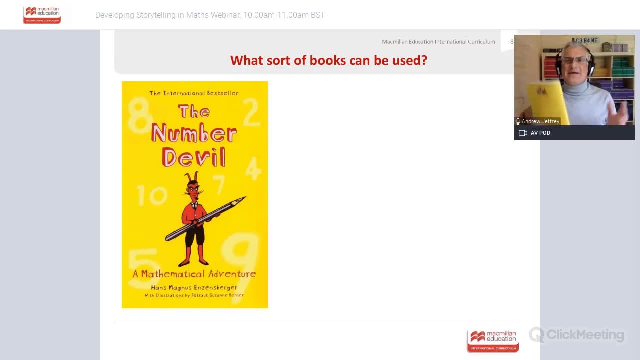 let's try and get the numbers that come in, so many of the big ideas in mathematics- in a in a great way, and it just takes him through like 10 different nights of his life when he has 10 different dreams, um, and he goes to number heaven and oh, it's very, very, very clever. 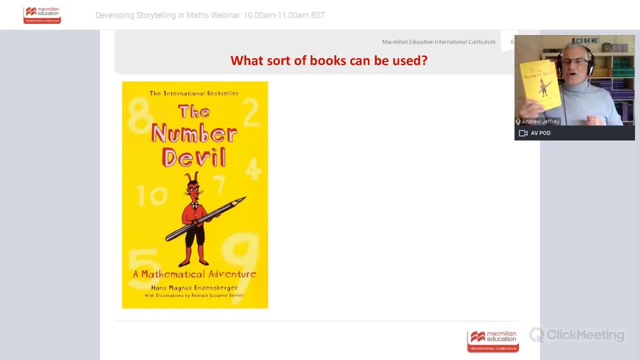 story. I can totally, um totally, uh, recommend this. okay, um, I've seen some some chat in the chat at the chat in the chat. at the end of this webinar, I will show you um a slide which, yes, you will get as a PDF, um with through the three very best websites that my research was able to turn up. 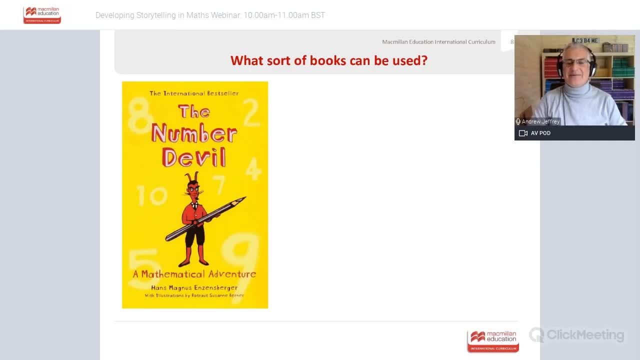 when I was preparing this webinar for you. okay, so, um, it will contain good ones for kindergarten, more or less anything for kindergarten that has, oh, someone's put a link in. thank you, okay, um, there are so many people have done so much work on it, but anything that. 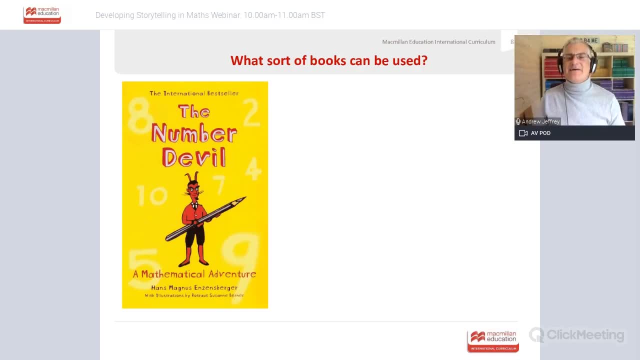 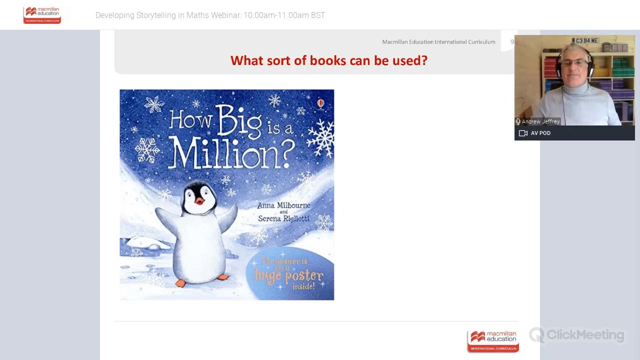 to do with number. anything to do is shape. anything to do with vocabulary as well. um, not the next one, but the one after I'm going to talk to you about vocabulary. so the next book I want to talk about was one of our favorites with our children. how big is a million? this is a brilliant and entirely 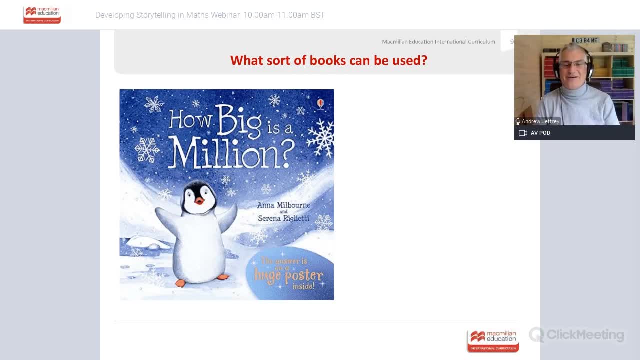 impractical book because it comes with a poster- okay, and the poster is enormous. it's the biggest you've ever seen, like film size poster, okay. so, um, this is a story of a very cute little penguin. this our kids all loved this. but the number of times we had to mend the poster with sellotape. 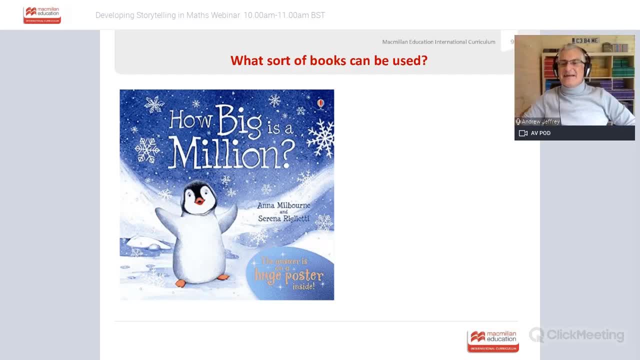 because it's so unwieldy. has anyone seen how big is a million? let me know if you've seen how big is a million. um, while I, while I'm waiting for you to type in there, um, I, uh. so this little penguin, he wants to know what a million looks like. he's never seen a million of anything, so he says his mom, I'm. 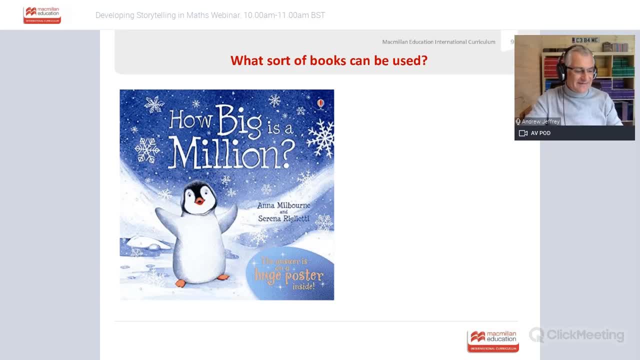 going to go out and find what a million of something is. and he goes out and he sees- I don't know if it's 10, 10 fish or something like that, and that's not a million. he sees 100 penguins. oh sorry, there we go. we've got a fan. Sarah's, Sarah's. 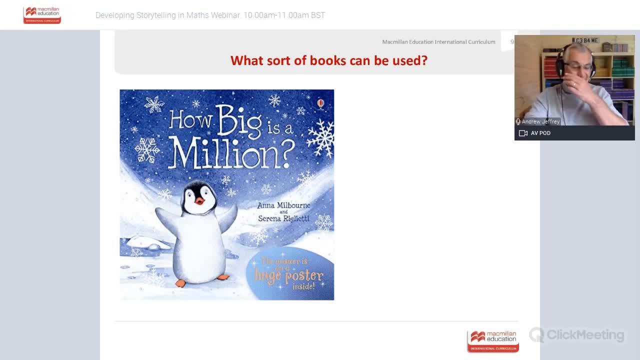 favorite book. how big is a million? um, definitely. uh, I've used this as a parent more than I've used it as a teacher. uh, that's how good it is. um and um. I still remember the shop I saw the day I bought this book. I couldn't write, I couldn't wait to get home. and then he sees a hundred penguins and he 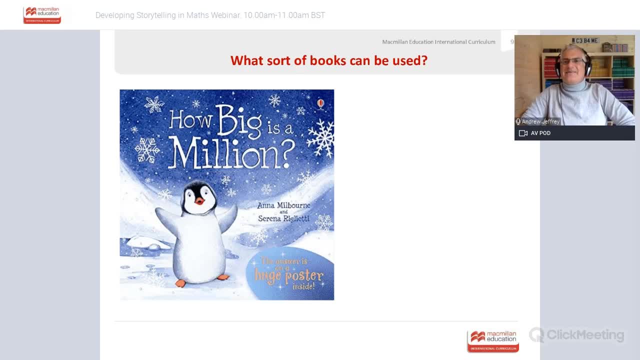 says it's not a million, and he makes a friend and he plays, uh snowballs with that friend and uh, he looks at the snowflakes and that's not a million, it's about a thousand. and it's getting later the day and he's really tired, he hasn't seen a million and he's very disgruntled and he goes home. I mean. 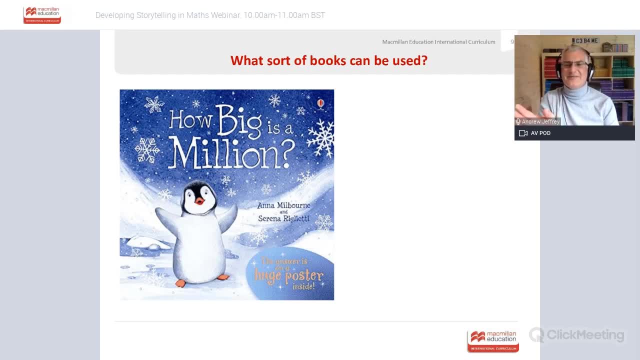 I'm obviously power paraphrasing beautiful illustrations, beautiful in this book. he goes home and he sees his mom and he's a bit sad and you know, like mom's do she's, so don't worry, she looks outside. they look up into the sky and by now it's dark and there are a million stars and 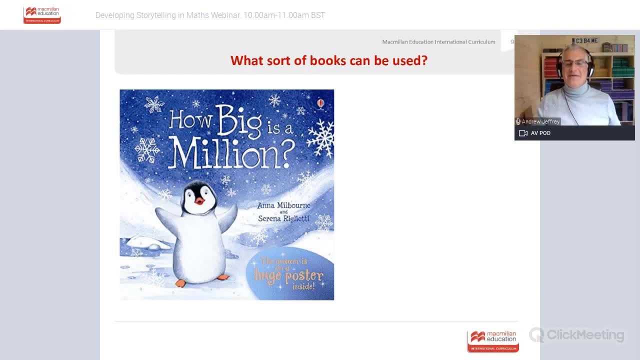 you open the poster and it's got a million stars on it. goodness only knows how they did this, but it's. I mean, this is a ginormous poster with a million stars on. I haven't counted them, no. so if there aren't a million, don't sue me, but I just think. I just think, um mil. yes, I can relate to that. 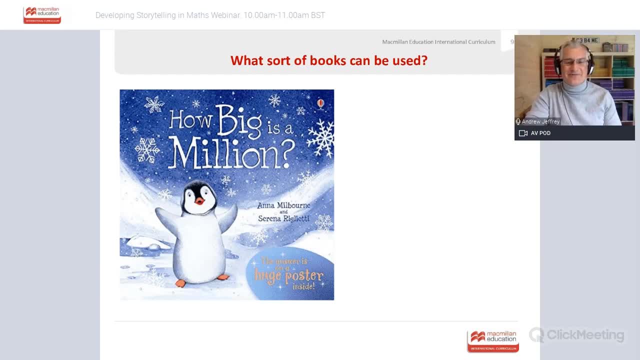 it's just got so much sellotape on it, um, from from having to unfold it and refold it, and so on and so on, um, so you can. you can tell whether a book is loved by how much sellotape, how many times it's. 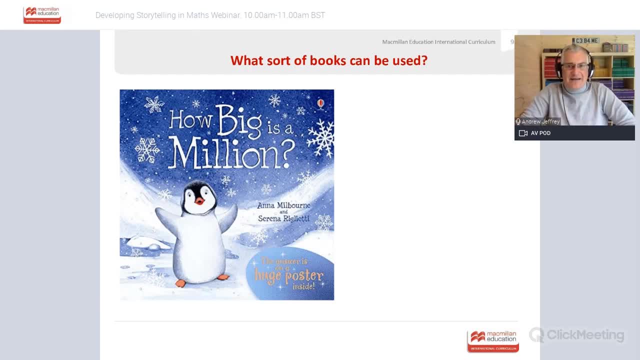 been mended um, but children have never seen a million. I mean, have you ever seen a million? I've seen a million pounds once in a uh in a museum in a glass case and uh, and that was quite fascinating. but a million of something, wow. I mean really well. 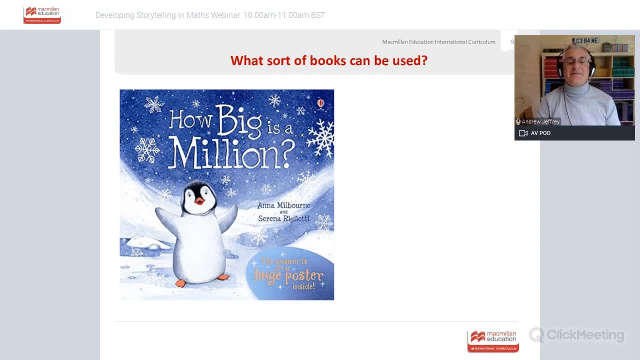 so, um, I I could thoroughly, thoroughly recommend this, but I'm so sorry, I couldn't like get it out and show you. they'd only just about be enough room in my office to lay this poster out. I can just show you my, my new. it's my new office. I'm only showing off because it's today. it's today. 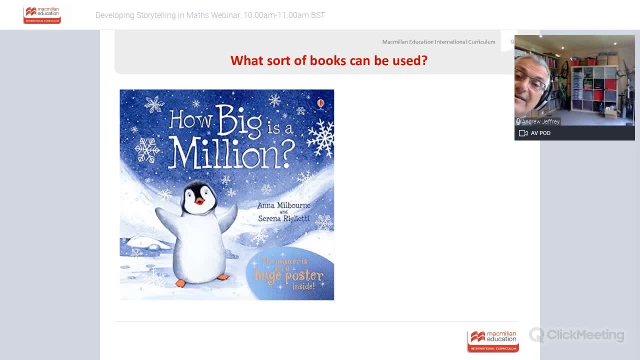 years old. this is the first day I've had my my brand new office, so you can see it, and I could probably just about lay the poster out on the floor. that's how big, how big it is, but what a wonderful thing. um, oh, you've just written a week of ideas for year five. 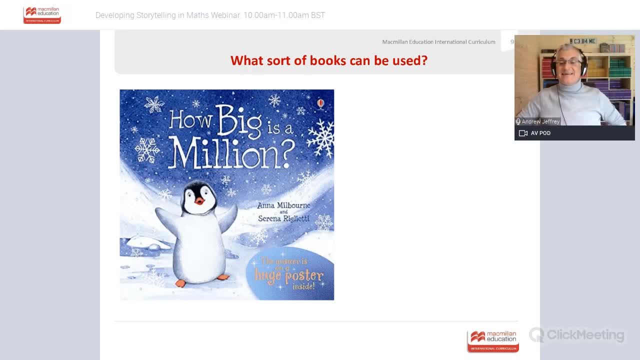 for this book. there you go, so a million comes into the key stage two curriculum. yes, thanks, it is a bit of a nice place here. uh, um, so I think, please- yes, you've just offered- to share it. that will be super. and, uh, my next webinar on bathroom stories will include a credit to you. um, so there. 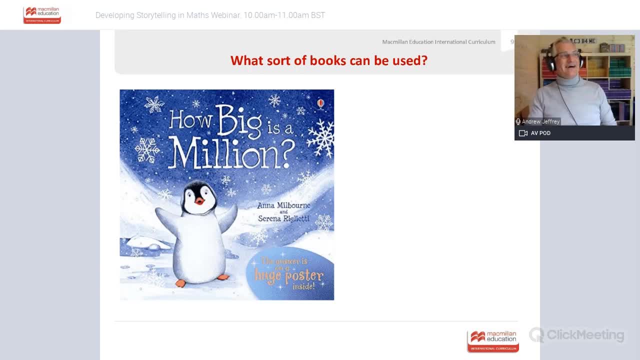 we go: how big is a million? it's beautifully illustrated and then you've got that bang, smack, surprise at the end. and I love the fact that it's not a surprise at all because they know it's, but they still want to see it. it's absolutely super okay. so the word million, as I said earlier, 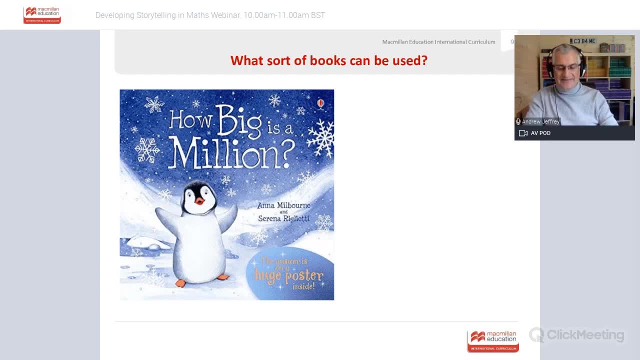 it's like one of those wonderful words that, uh, children in year one or year two are very, very excited to hear. uh, because it's such a big big number, um, but but here we go. lots of nice, completely irrelevant comments, so I can show you my office. I'm just like, I'm like a kid with a new. 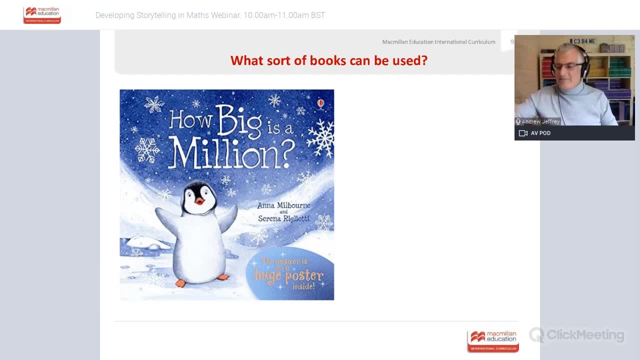 toy with my new office. so, um, so I want to talk about the next book I want to talk about. our book is, um, a very, very funny. well, I think it's funny, but that's because I like puns and and word play and vocabulary and crosswords and this kind of thing. so I, uh, I, I want to recommend to. 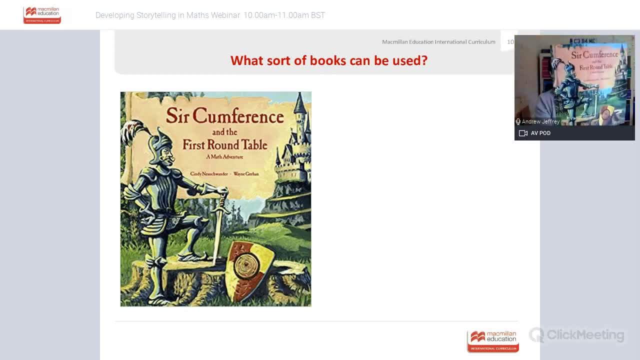 you this book and it's called circumference and the round, the first round table. I've got a copy here and if you're sitting comfortably then I'll begin. but but the vocabulary? even though as an adult you can see the jokes coming, they're still great, I think so. 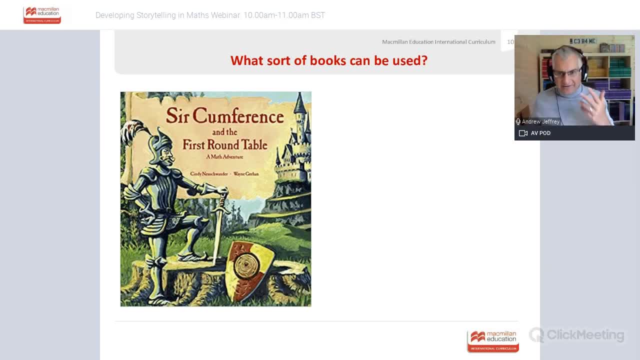 I'm going to do what I did with the previous books. you just not read them all to you because that's a bit tedious, but I'm going to read a few bits so that you get turn that around, so that you get the hang of it. so here we go. long ago, in a land known as Camelot, there lived many Knights. 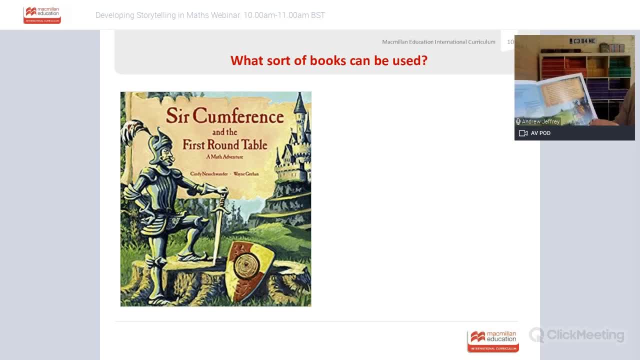 and ladies. their ruler was a mighty but gracious man named King Arthur. during many years of peace and good Harvests, the people lived happily. ah, the trouble began when they saw the army of their neighbors to the north gathering at the border. these people, known as the circumscribers, looked as if they might be preparing to make war. King Arthur called them. 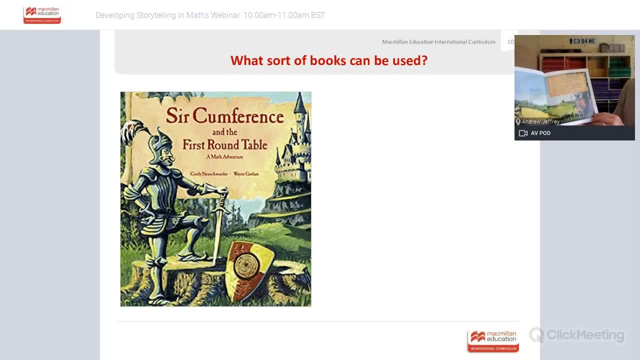 on his bravest and most trusted Knights to plan what to do. okay, so here they are. they're sitting at the table. it's a long old table. now I'm going to cut a long story short, swing back round for you. um, circumference was married to Lady Di from the town of amateur, I know right, and they had. 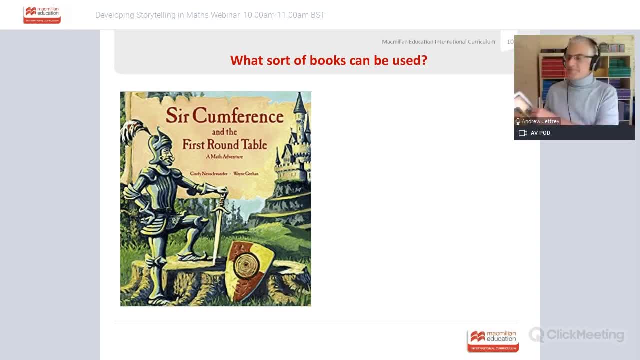 a son called radius. you can definitely see where this is going, okay and uh, he was complaining one night to his wife that he had a sore throat from shouting the length of this long table at all his nights. so they had an idea. and you can do this, you can actually give. 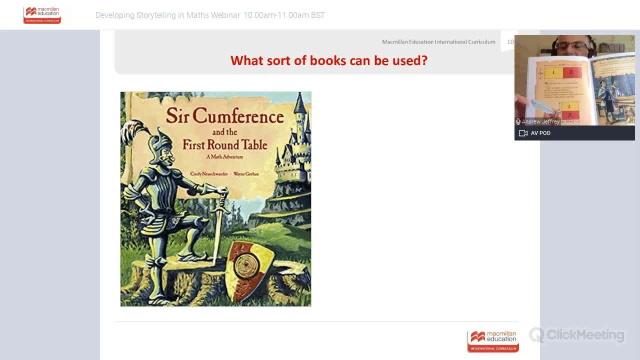 them paper and get them to cut them up. so they cut the long table so that they still have the same amount of table, but they cut it in half and made it into a square. now let me digress slightly. here's my white board. when we got um interactive whiteboards like this. this is just a normal one when 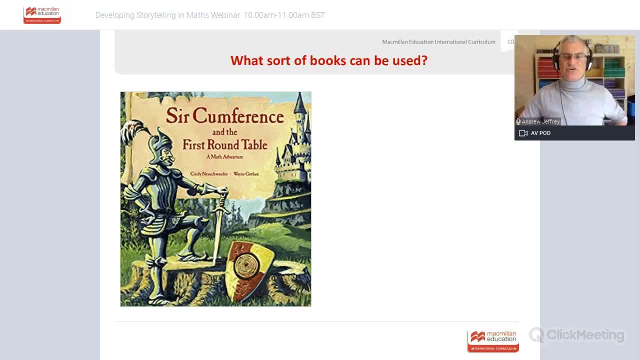 we got interactive whiteboards in schools. I think there was so much we could do on them. like for the first time ever, I could actually draw a proper regular Pentagon, which is great, okay, uh and um. but I think we lost something. we lost that tangibility of learning shape by folding paper. 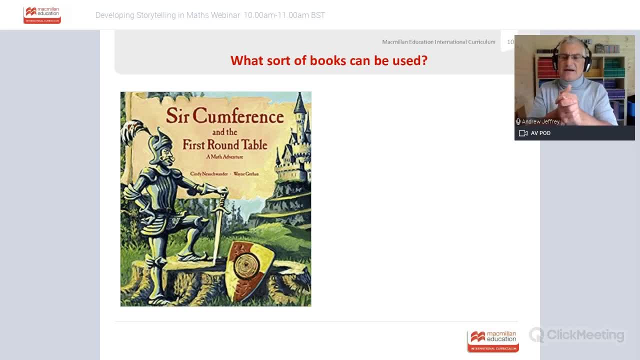 and I think that the idea of symmetry, uh, just, uh, just to answer those questions, there are ISBN numbers on the backs of these and uh, if you just type these into um, type the names of the titles and you're into any website, uh, or any online book seller. I can't think of any online book sellers at. 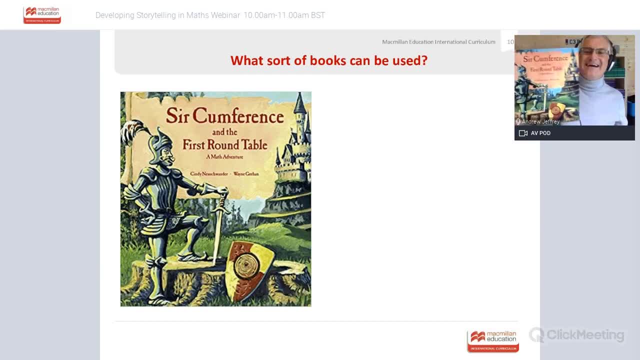 the moment, but you know, if one comes, oh there we go. sorry, I just bought my son um book depository is good. uh, thank you, Kerry. that's where I got some, because they're often uh, secondhand and cheap, but in good, Nick, okay, so I I think I paid like four pounds for a place for zero and that sort of thing. 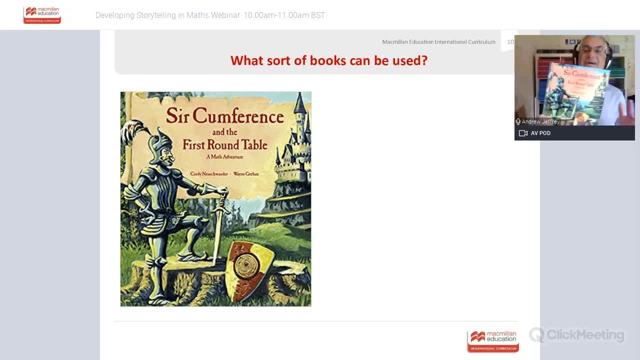 five dollars. so, um, you don't need a first-hand copy, you don't need a brand new copy. uh, if money's tight, so just Amazon. yes, obviously happened anyway. um, so they worked on this square table and I think we should give children a piece of paper and say: change it, change the area, redesign it. you could. 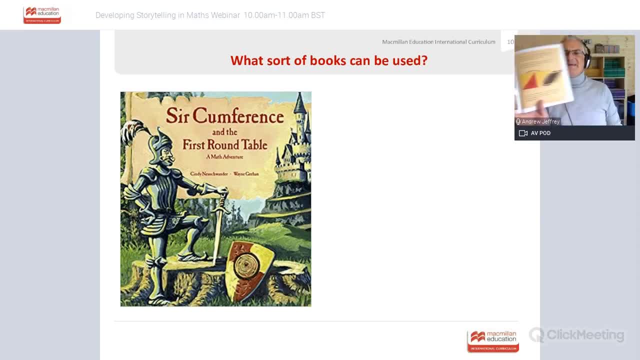 get them to redesign it. um, but then then they realize that at the square table everyone's chatting at different, uh, four corners. so they say they reconstruct it into a parallelogram by cutting it in half along the angle and making it para. I just think that's brilliant, I mean, that's actually. 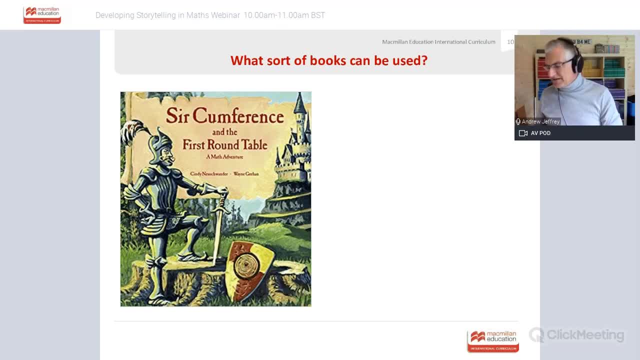 uh, but you could say that's not a mathematical terminal, that sort of stuff. so now it's a rhombus and now the king doesn't like that. anyway, they go through various different permutations. then there's another construction you could get them to do, which is to cut the rhombus into an octagon. 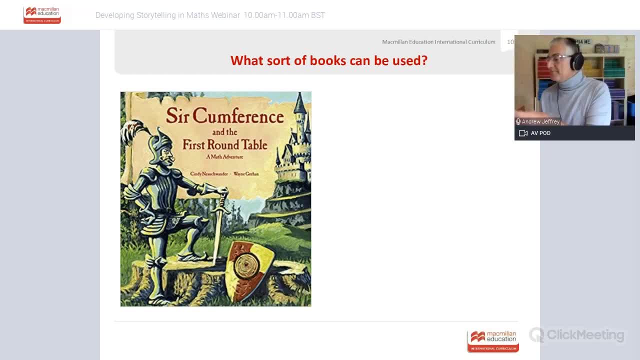 I've never seen that construction anywhere before. okay, um, and that's that's not working. okay, that's not working because there's 12 nights and, uh, there's 12 nights and only one, uh, only eight sides, so that's not working. and then, of course, you probably guess what happens. 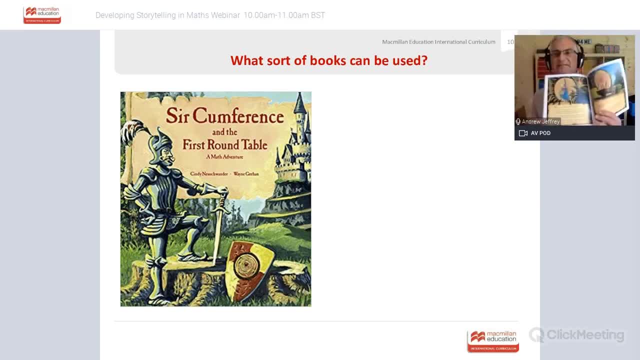 um, they're out, they're basically out for a ride, and circumference finds a lovely tree. they cut a cross section of it. they take it back. he says: leave the bark on, it's nice. um, and now they sit at a round table, okay, and the king's very happy. and, um, he said uh, he said because, um, because, lady. 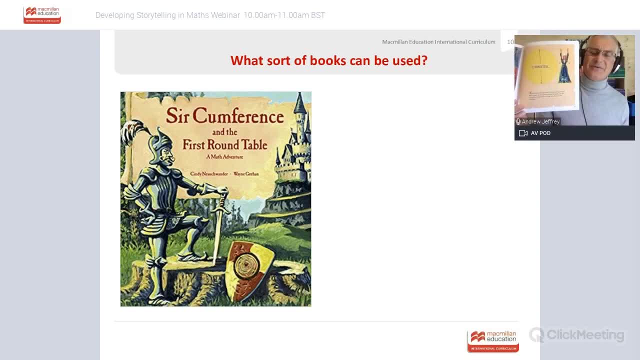 die of. uh, amateur is the same height as the table. we're going to call this. um, this distance, the diameter, which is just brilliant, right, corny, but it works okay. um then, their sun radius is. is honored by being named the uh, the height from the center downwards. 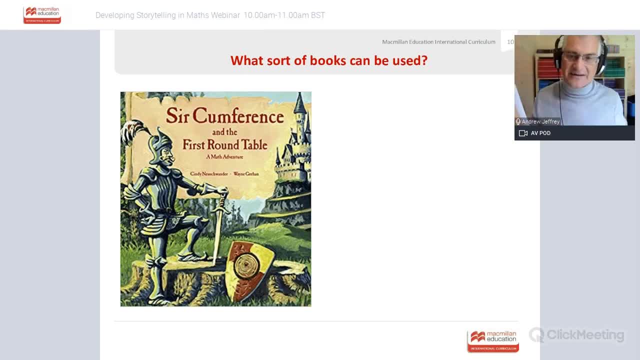 um, and then, of course, because, uh, circumference, the night circumference, decided to leave the bark on around the outside. then the distance around the outside is called circumference. okay, it's witty, it's not the most you know, it's not stand-up comedy, funny, but it is funny. and 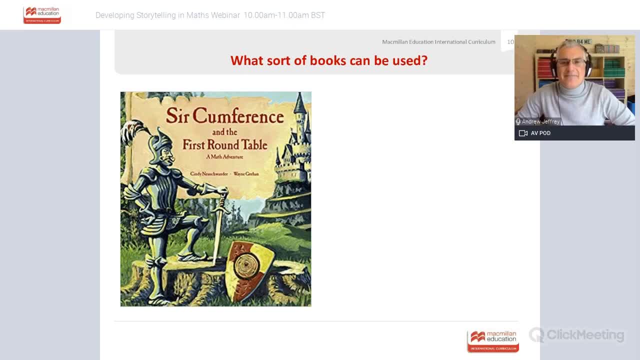 it's quite a nice way of remembering the difference between diameter, circumference and radius, and it's, and it's a brilliant for vocab. I I just it made me laugh. it made me laugh so much I had to buy it, okay, uh, and it is. it is a really clever way. if you have children with um, you have. 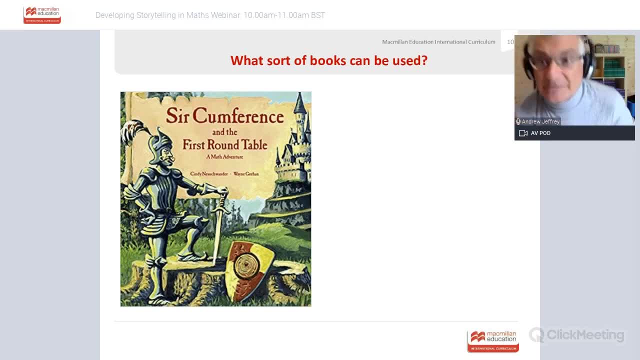 children with learning problems. uh, if they have difficulty with memory or vocabulary- I have, I have issues with my memory, very specific difficulty with my memory. so for me something like that would have been brilliant at school so I wouldn't have to remember, and anything that helps you like that, uh with with mathematical vocabulary has to be a good 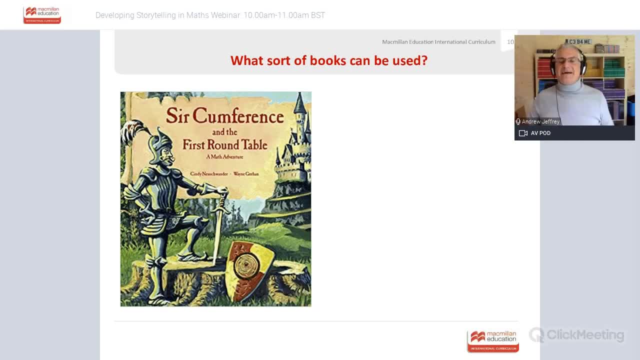 thing if it makes it a punny, corny thing. okay, right time for another on-screen book now. um, now, I should just say, before I leave this one, that this is, this is just one in a series of books. there's a lot of circumference, maybe five, six, seven, eight circumference books. so if 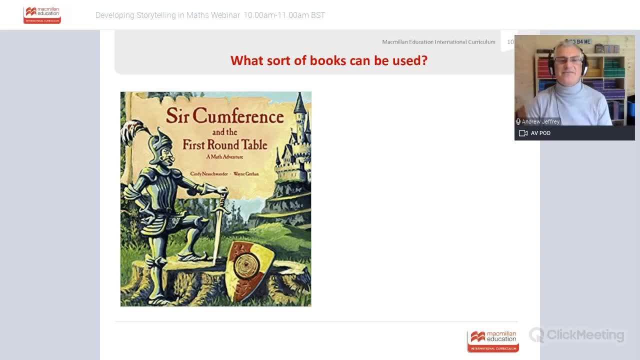 you go on to uh Amazon or wherever, and type circumference and the first round table, it'll probably just give you all the other circumference books. this is the only one I have, uh, personally, because I'm trying to pare down my- um, as you can see, rather excessive library of books, books. 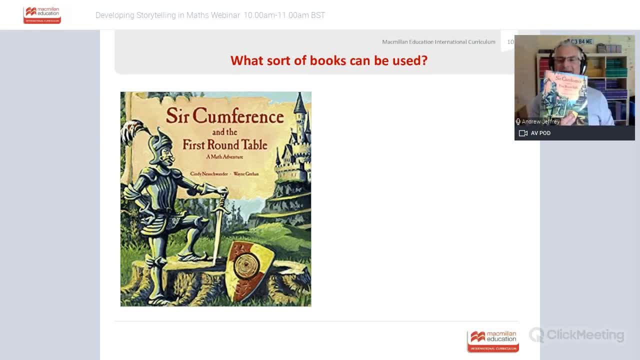 um, but this one I couldn't get rid of because it just makes me smile at the ingenuity of the story and I think, and you can see, can't you have to use that in a lesson. give children a rectangle, give them some scissors, give them a pencil, give them a ruler, get them to redesign the table. all right, get them to. 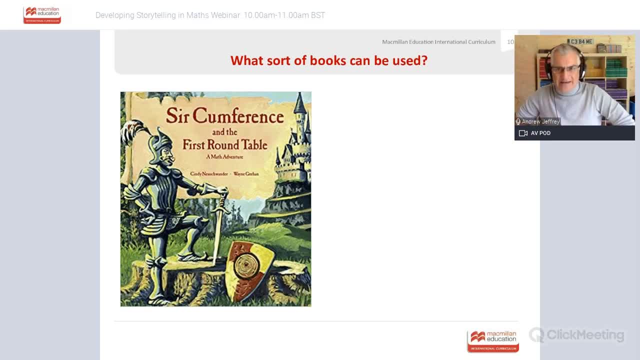 think about, uh, why a circle is such a fair way and- and of course this PSHE here- a round table has no head. it has. there's nobody at the head of the table, uh, and so that's why round tables are popular in some cultures, because they they are equality equalizers. nobody's like more important um in. 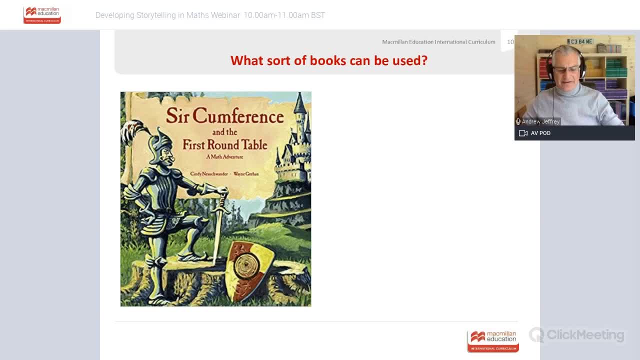 fact, I remember um this, the story of the last supper, when, uh, in the Bible, and people were clamoring to sit next to Jesus, like that was the important place. well, everyone has an equal place on a round table, so I think that's a marvelous one, right? let's go down to um. let's go down to the next one, and this is the last book we're going to. 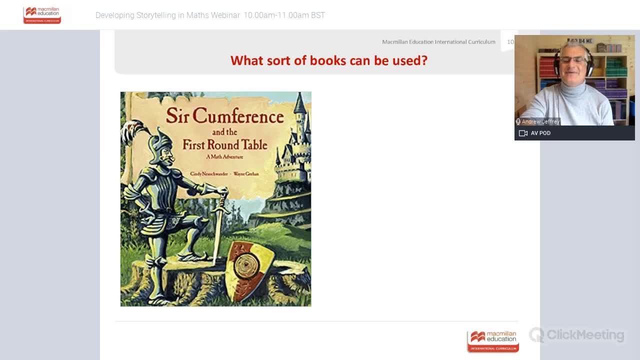 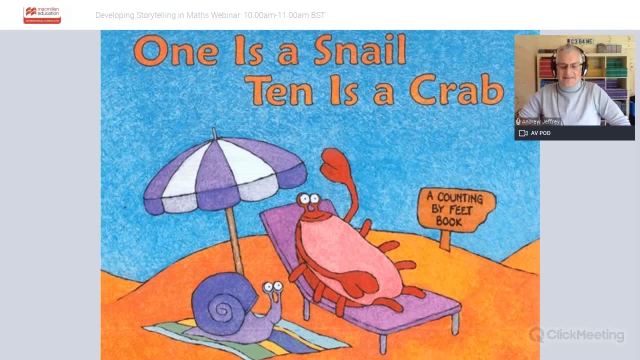 look at today. uh, it's a an absolute beauty. it was very popular in the UK about four or five years ago and it is called: one is a snail, ten is a crab. so just, uh, just put a hand up by saying yes, if you've heard this one, uh, if you've seen this story. 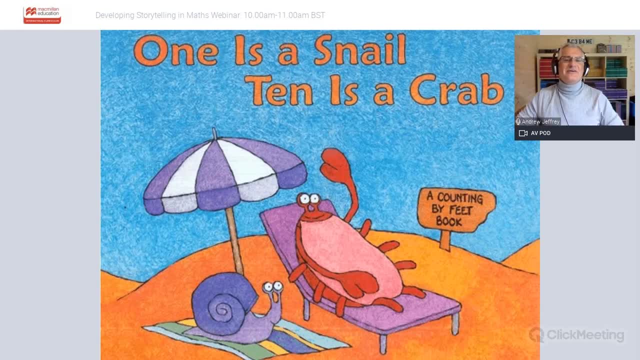 there we go. we've got a fan- Juliet's a fan of this one. um, I wonder if you you may have read it or you may not have read it, but it's a super book and also, more importantly, I think this is a fabulous book for teaching about um part part whole. you might not have thought of it as a part part whole. 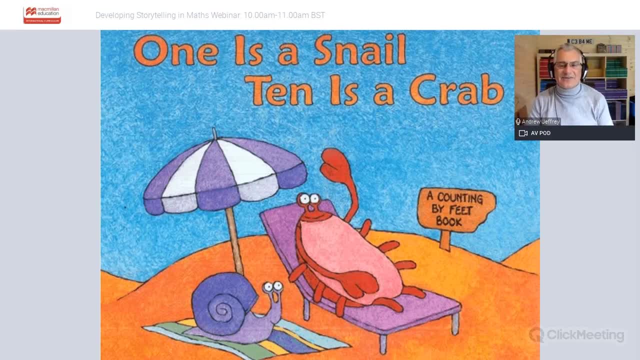 resource um, and not just that, uh. there's also the idea of uh, of like mental arithmetic of arrays gosh. there's so much that you can do with this book, plus it's funny, plus you can do guessing and predicting. so if you have um, if you have seen this book, that's. 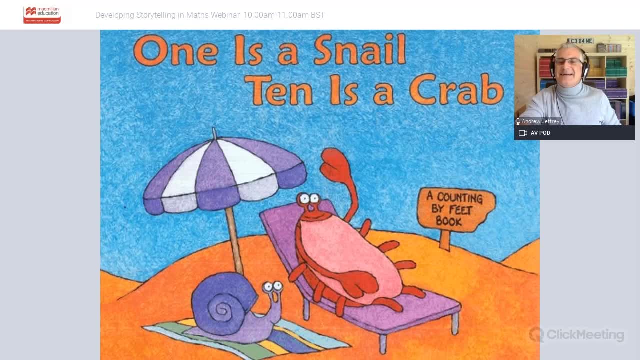 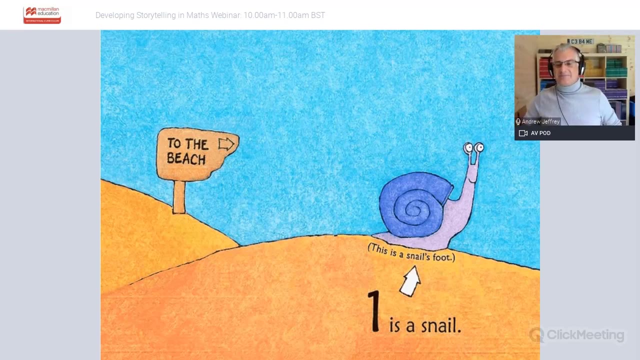 fair enough, okay, um, try not to try not to let on too much. okay, because there's quite a lot of people here who won't have seen the book. so, um, let's, let's go for it. I think the illustrations are just hilarious. I there's those. the way they do the eyes. I think it's brilliant. one is a snail. 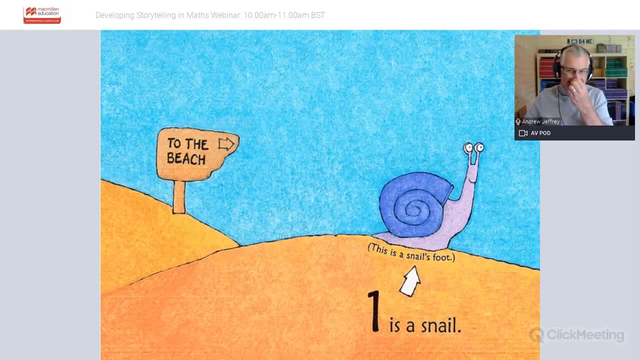 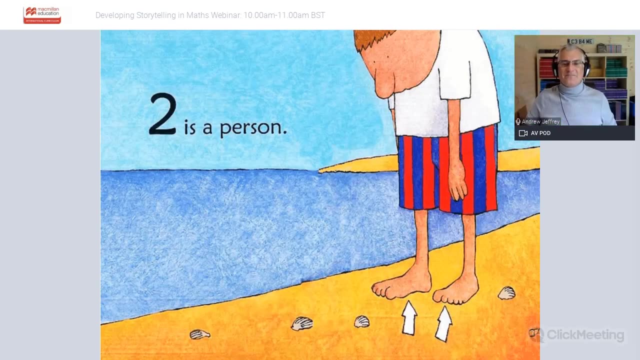 this is a snail's foot. that's interesting, isn't it? this is a snail, so that's what it says. one is a snail, two is a person, and now it's got two arrows to the feet, so it begins to give you a clue as to 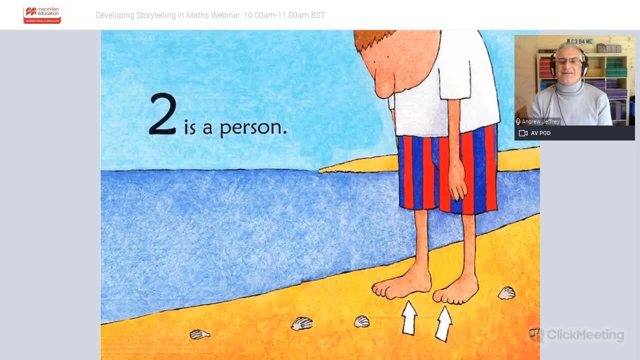 what this book's really trying to say. okay, so if one is a snail and two is a person, let's play a little game. I did this this morning. it was good fun. type into the box a tricycle, excellent- a stool. the answers are already better than the first session we ran. 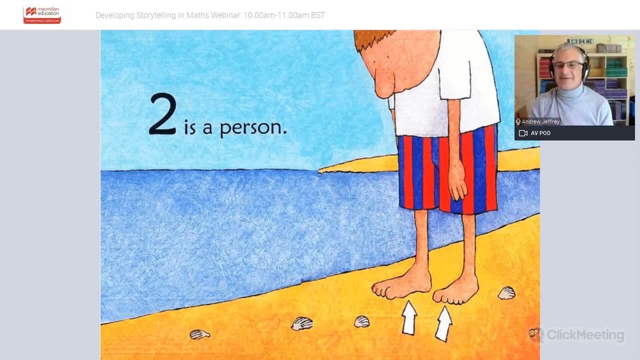 well done, okay, very good. anyone else it says: five people are typing right now an auto. okay, tricycle, I like that. well done, tiger tots. yep, okay tripod. thank you those you know for not giving it away. okay a tripod, all right. quite a few votes for tripod. 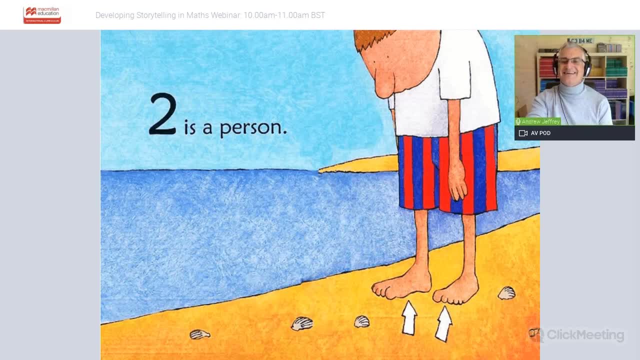 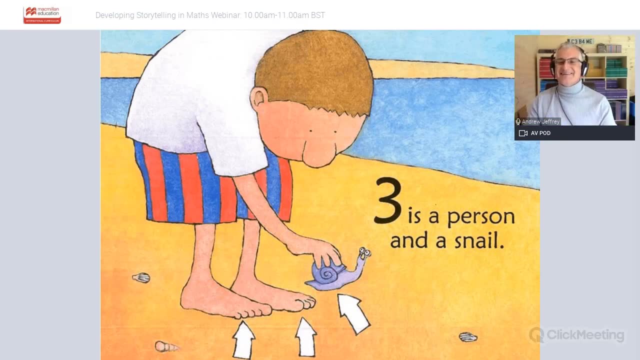 you're very creative. okay, i'm going to show you what three. is you ready? that's a person and a snail. i love them. uh, we overthink things sometimes, don't we? a snail and a person. okay, i'm gonna, i'm gonna. i'm gonna assume, elizabeth, that you definitely were typing that. 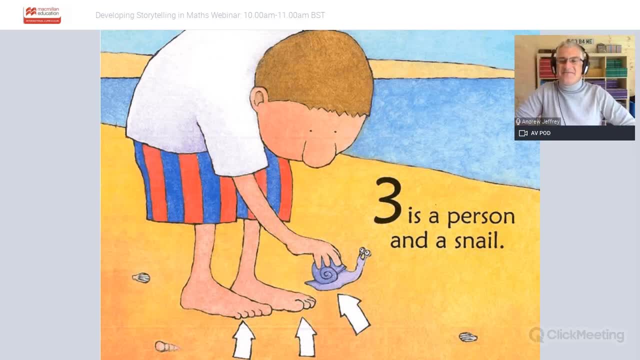 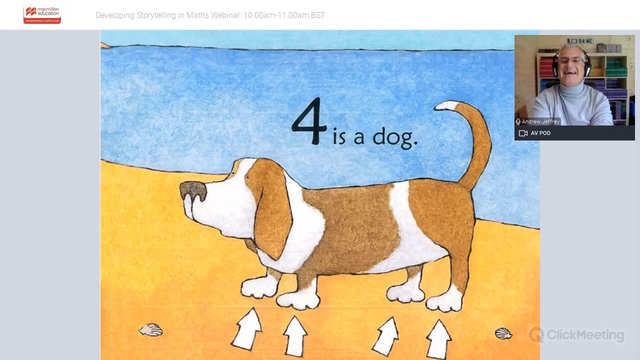 before i showed you. so you get that. i'm gonna give you the the benefit of the doubt, because i'm a trusting person. it's a personal style, all right. and uh, four, anybody want to guess? four, yeah, yeah, okay, you've all got that. it's a dog, falls a dog, okay, and again with a class: this: 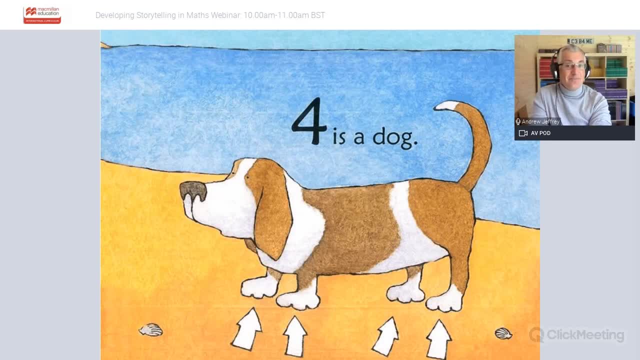 is hilarious, because it could be two persons, couldn't it? or it could be four snails, or a person and two snails- um, they don't think they're doing maths. five is elephant. oh, that's. that's the comment of the day. you win a prize. you win a round of applause from me for. 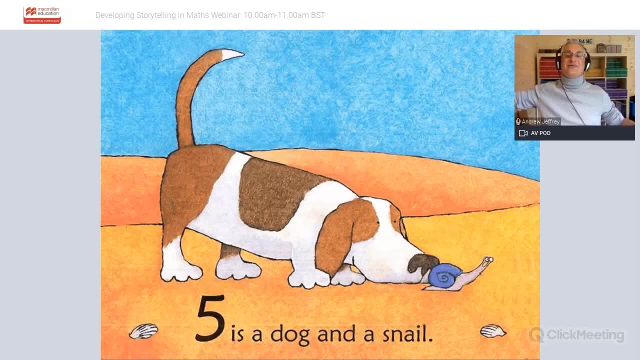 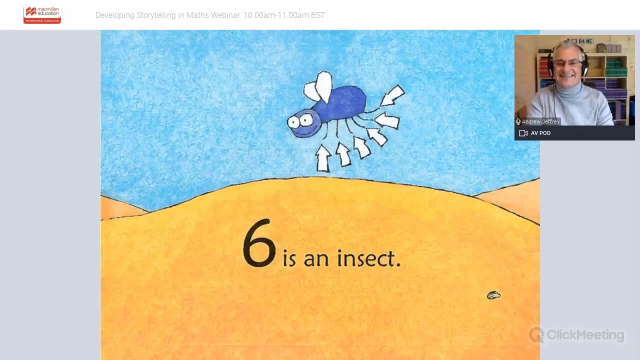 five is an elephant. that's genius. but in fact five is not an elephant, it is a dog, and a snail elephant would have been funnier. okay, now we move away from dogs to six, and six is an insect. so there you go. a bit of science in here as well. 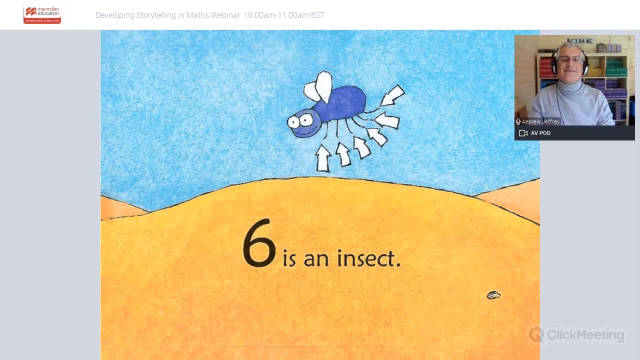 maybe it's just me, but i just think this is hilarious, but hilarious with a really serious thing going on. what's going on here is partitioning of numbers, right. what's going on here is the ability to create numbers from building blocks of other. which insect is that? sorry, i can't answer that. this is a. this is not a science. um, uh, a science webinar. 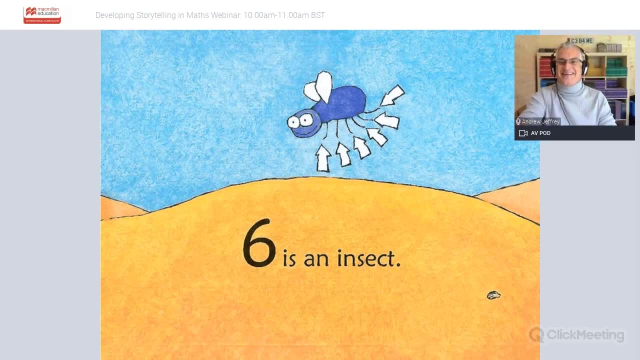 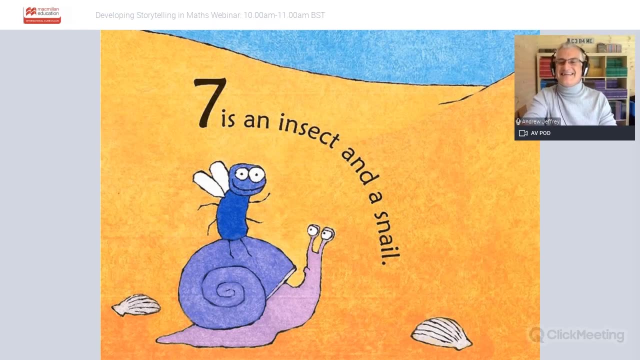 um, i haven't got a clue what insect that is, but i do know that when it sits on a snail that'll be seven, that's all right, so you'll get the hang of this now. eight: anyone didn't even realize a fly has six legs. well, wasn't it worth you coming today. 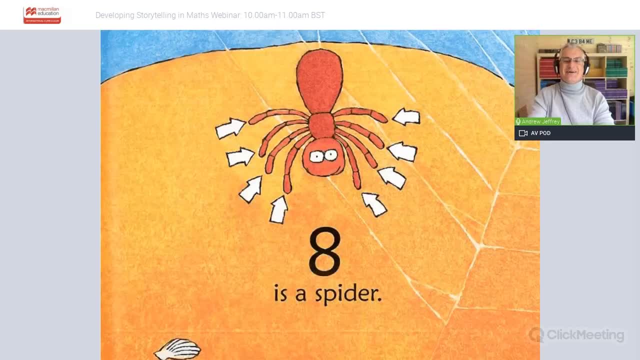 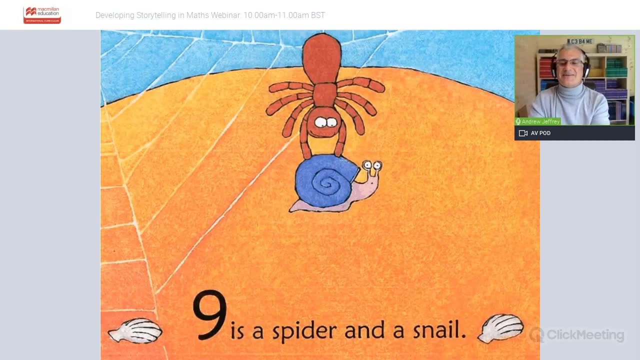 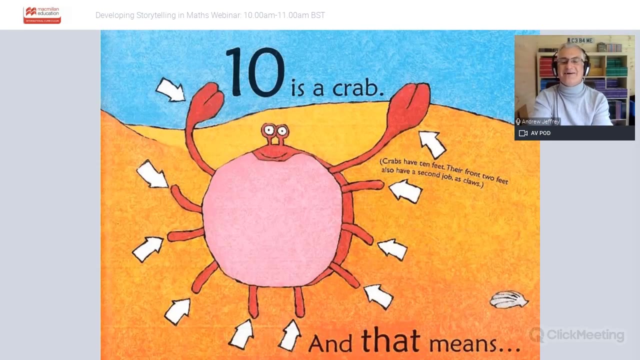 i guessed octopus. i was also wrong, it's a spider. okay, eight is a spider, and you can have great fun with spiders. and of course, a spider with a snail is nine. and then, finally, if you remember the title of the book, you'll know about ten. oh, two dogs could have been eight. very nice, yes, you see. but 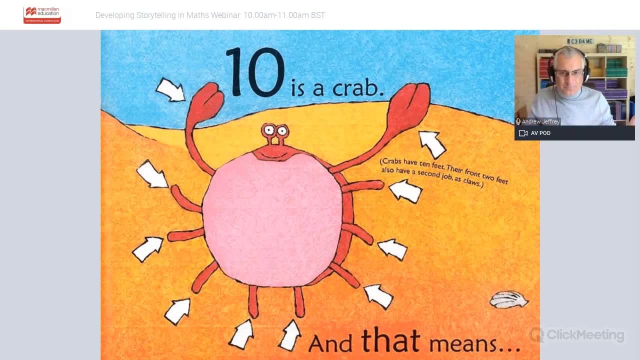 what's brilliant is two dogs is eight, and so if you're a spider, you can have great fun with spiders. so we start to, as with our little brains, are starting to think: oh, there's different ways of making numbers. okay, now, uh, leg a little bit of science. crabs have 10 feet, and so on. crabs looks. 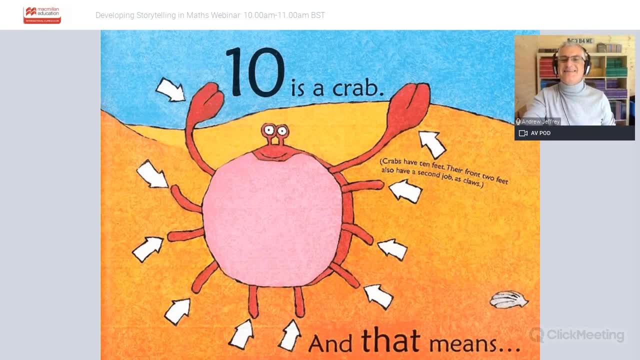 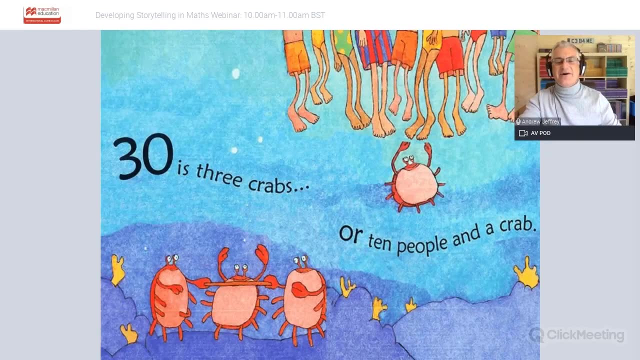 like a little drum. okay, don't hit it, that would be cruel. okay, 20, any idea about 20? we could play this game all day, but actually i'm just keeping a wary eye on the time, so we can't. it's three crabs, or 10 people and a crab. or or or. and here's the thing you could give children: a big bit of paper. 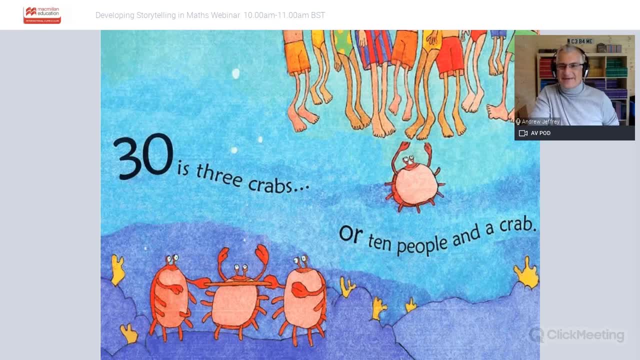 you've given some, uh, probably numicon would be the best thing, wouldn't it? um, and ask them to make 20 or draw 30 or whatever. how many different ways could you find? and so completely differentiable. um, rose, you've just put your finger on it. this is hilarious, it absolutely is hilarious. and if 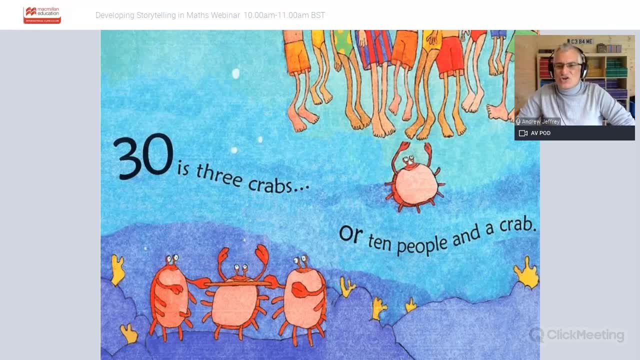 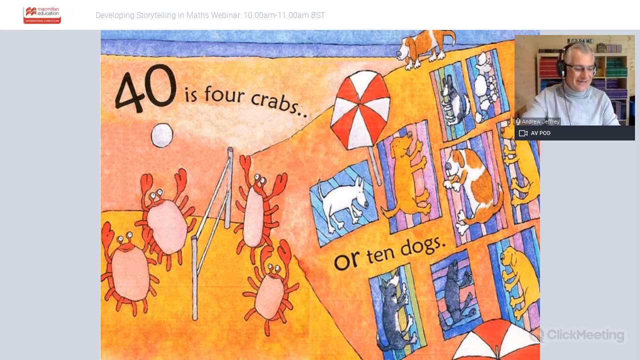 you're having fun with numbers. if you're enjoying numbers, you're winning, right, okay, and it's a great way in. so for the sake of completion, i'll look at the comments. everyone loves this book. four crabs or 10 dogs? i love 10, 10 sunbathing dogs. i've never seen a dog on a beach being still they. they're far too excited. 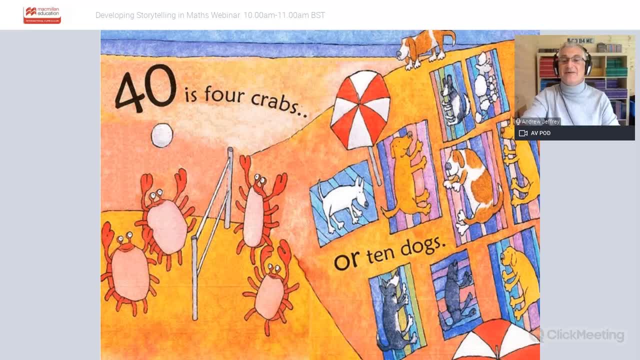 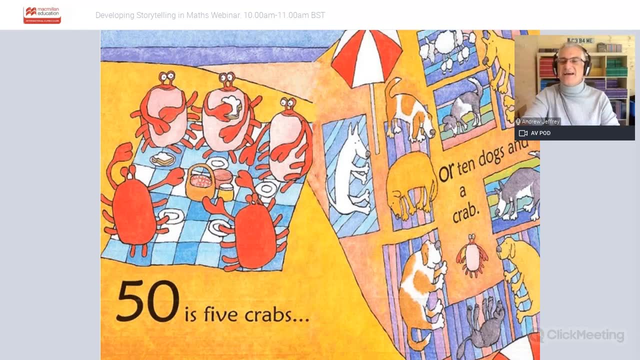 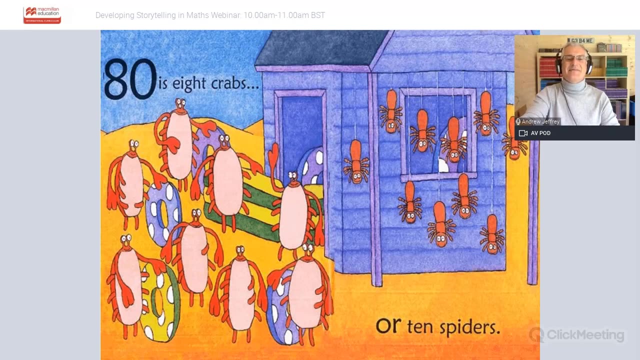 but there you go, my dear. to be fair, i haven't seen four crabs playing volleyball, so 50 is five crabs, or 10 dogs and the crab. imagine mathematics you're doing to check these. okay, i'll just keep going: 60, 70, 80, and they become more and more creative. now this one i particularly like because 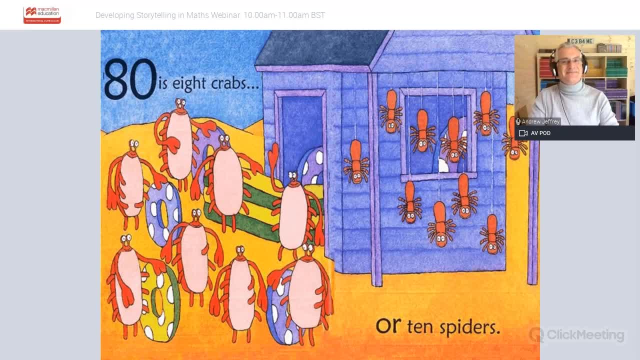 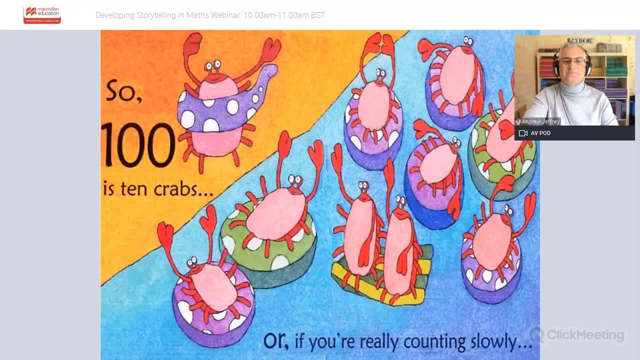 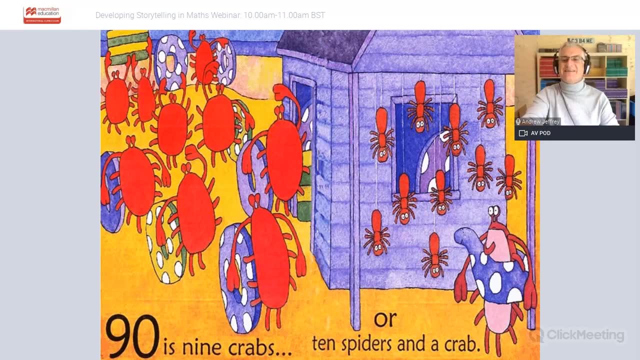 the people saying the pictures are great. um 90. oh, hang on, miss 99 crabs, or 10 spiders and the crab. so we had 80 here. we just added a 10. now 100 is 10 crabs, or if you're counting really slowly. 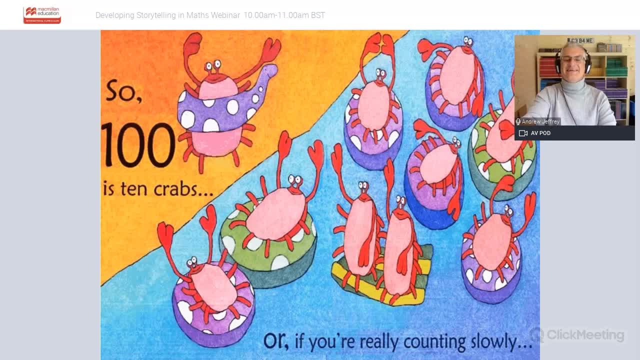 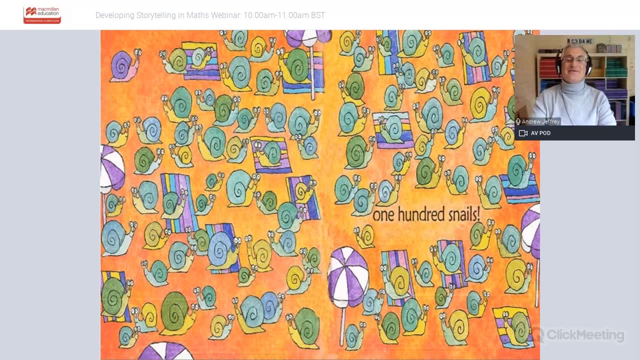 and i'm sure you've all guessed the ending. if you're counting really slowly, 100, i love it. i'm so sorry i haven't got a copy of it here to share with you, but that's the. that's probably even better to see on there. now your mind should be racing at what you can do with. 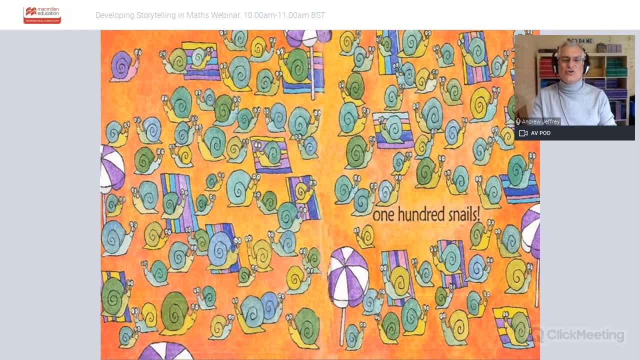 this. all right, so you can say: so, we've got one, two, uh, we haven't got a three, we've got a four animal, we haven't got a five, we've got a six animal, we haven't got a seven, we've got an eight and a ten. so what can you do? what can you do with those numbers? 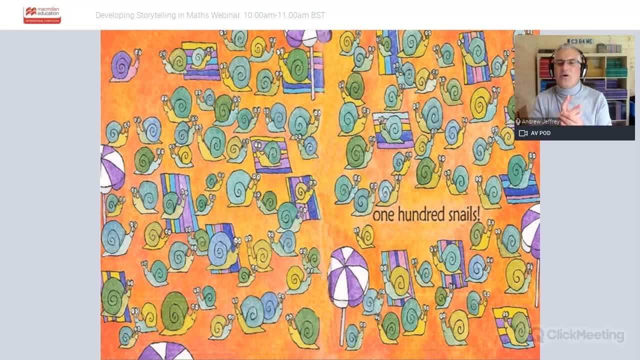 are there any numbers in the world you can't make or if you take out of, if you take out snails? so what you could do is draw. or, if you're not very good at drawing, just screenshot some of these- uh, earlier ones where it's like single. let's just go back to where it's a single one. 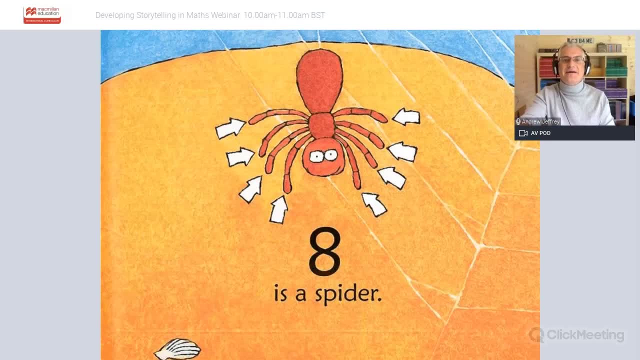 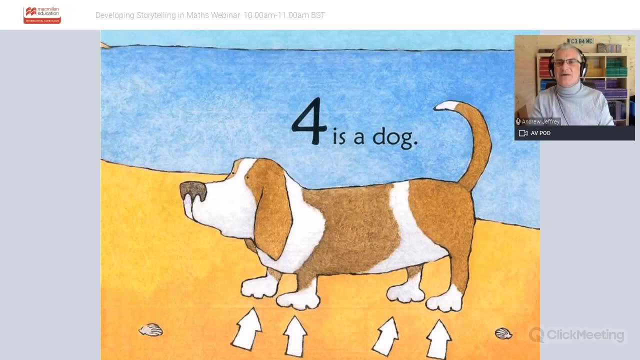 yeah, you can screenshot the crab, you could screenshot the spider, you could screenshot the insect, you could screenshot the dog and say, all right, what can you make? or there are 20 legs on the beach. what's here and the? okay? they just think they're doing art, but the mathematics they're doing is 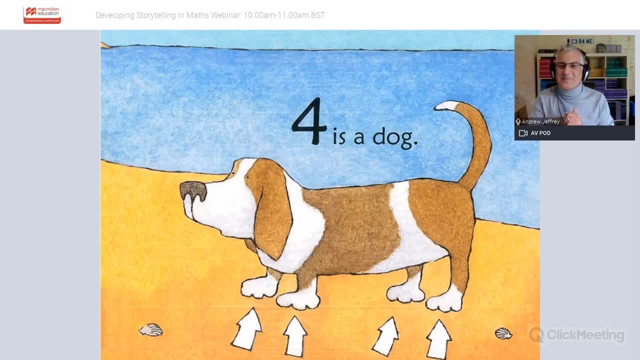 terrific. jocelyn likes this one as well. can't stop smiling. i do. you know what you've just reminded me of? my first time reading this book. i thought it was hilarious, and i distinctly remember the person sharing it with me, asking me to guess what comes next. that's probably why i did it with you, so. 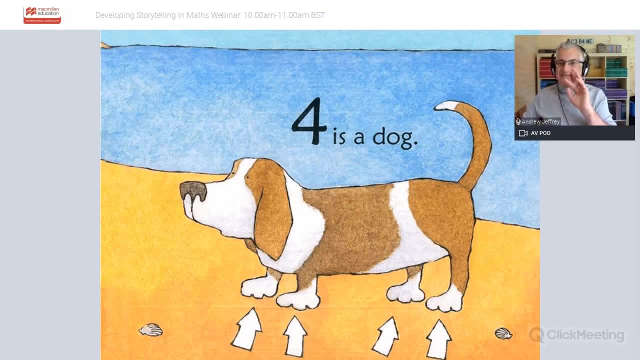 um, yeah, dude, don't, don't just show them the next page. i asked them to guess and i think it's so much. first south africa. i'll just have to change number for it. interesting, okay. yes, yeah, you will. okay, and just people draw numbers in different ways, all right. 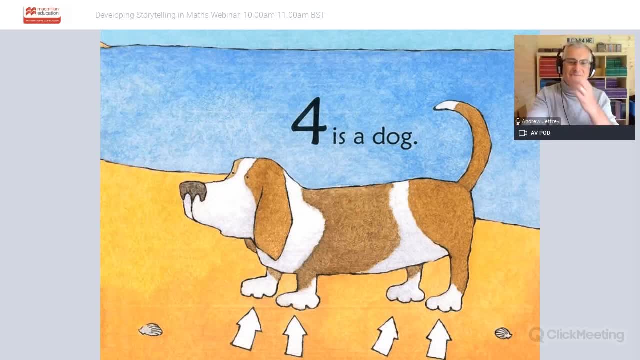 okay, now i've sort of a boner. i hope that's made you think about all the different ways you can use books: not just read them and talk about them, but actually get some practical maths going on. okay, but i want to finish, uh, if i may, before we've got some time for questions. 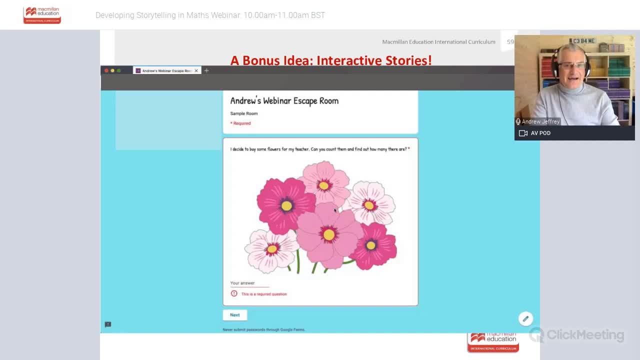 with um a bonus idea now i i had this idea from a um a session i attended myself only a few months ago. you know, i had this idea from a um a session i attended myself only a few months ago, you know, because i've never really heard of google forms. there's a couple of obvious advantages to google. 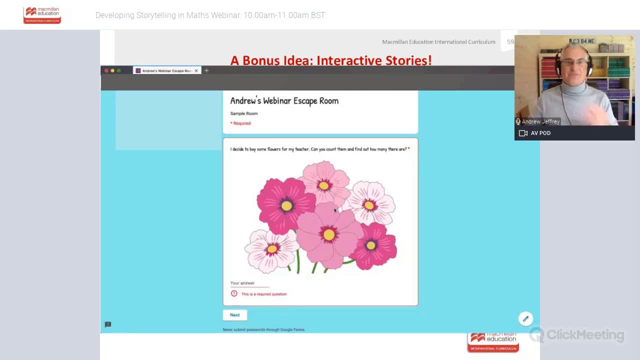 forms. firstly, they're google, so they'll they'll work in every platform. secondly, they're free- okay. and thirdly, they're pretty easy and intuitive to use and i, with a bit of practice, i made up a story. now, please don't get excited. this is just a demo story to show you how the, the technique works. 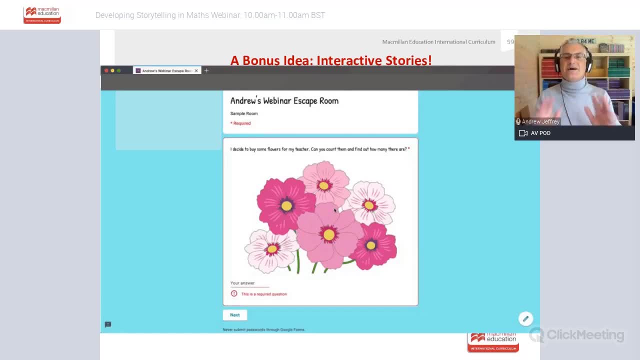 but you don't need any software. google forms is entirely web-based, okay, so this is called andrew's webinar escape room, okay, and i built it up effectively. all it is is a series of web pages with a question on, and, depending what answer the user puts in, depends on which web page it takes. 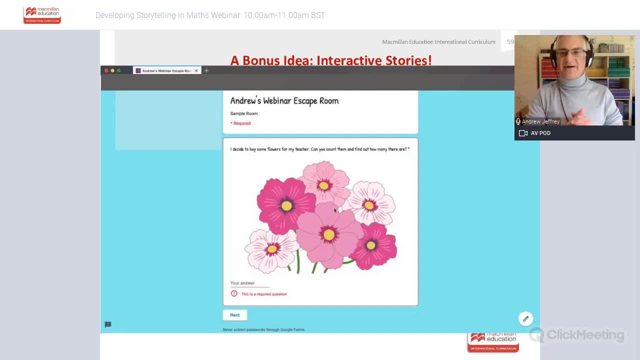 you, so you can have a page that says a question, then you can have a page that's going correct- here's another question- or a page that goes incorrect. have another go, yeah, and you can just loop it around. all right, so it's like hyperlinking. but, um, i'm gonna cross everything i have now and 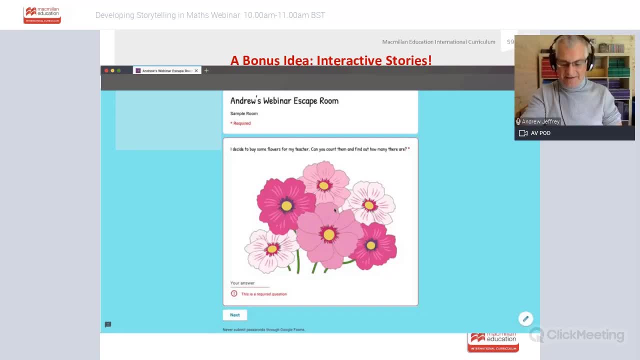 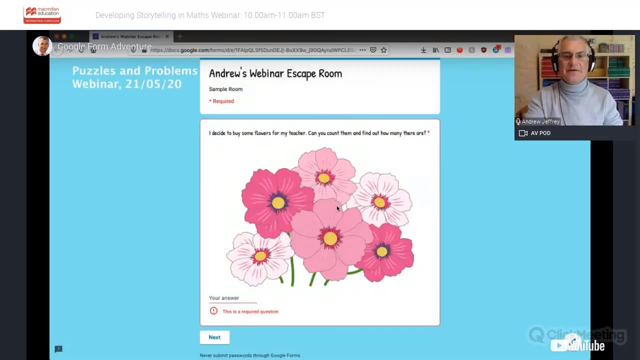 switch to youtube, and here's a very, very short one, just to show you the possibility. fingers crossed. oh, this looks exciting. andrew's webinar escape room. i decide to buy some flowers for my teacher. can you count them and find out how many there are? i'll just guess. i'll just put my answer here. no, i'll just click next. oh, it's a required question. 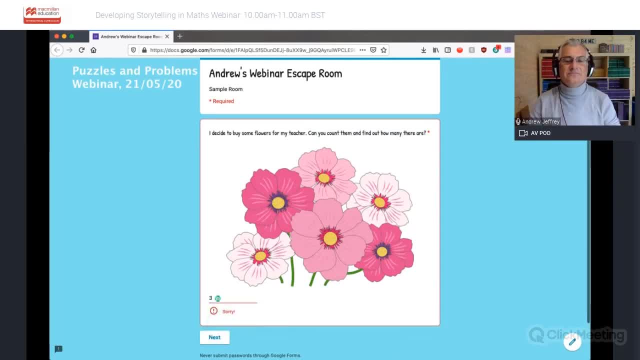 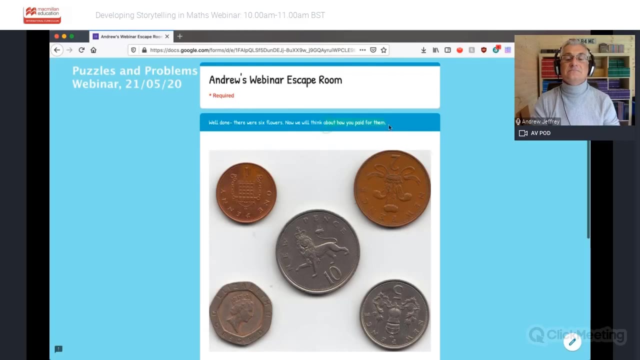 okay, three, let's try that. three next. sorry, oh, i have to actually count them. okay, so we're going to choose the assimilating ones next, right? so here we have the first one. one, two, three, three, four, five, six- let's try that. six, is that right? let's hit next. well done, there were six flowers now we. 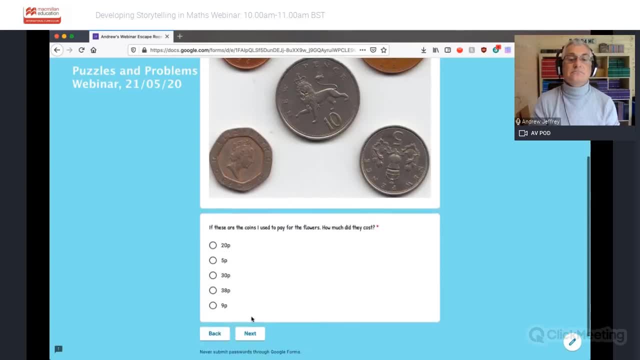 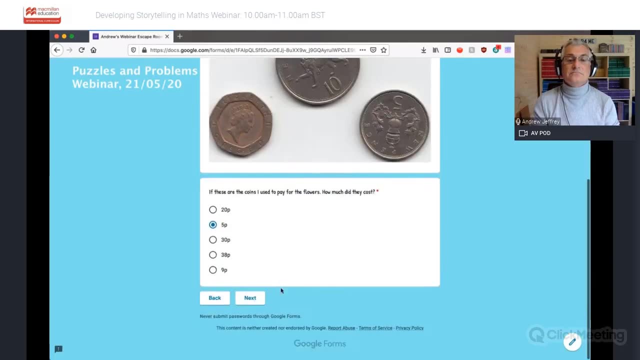 will think about how you paid for them, okay. okay, these are the coins i used to pay for the flowers. how much did they cost? 20p, 5p, 30p, 38.. oh, look, one, two, three, four, five. definitely five, there we go, got that one, all right. next. 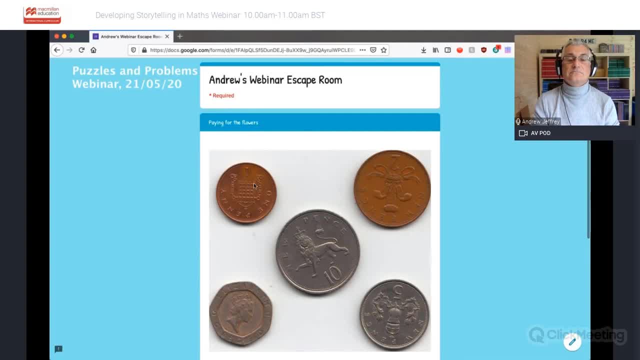 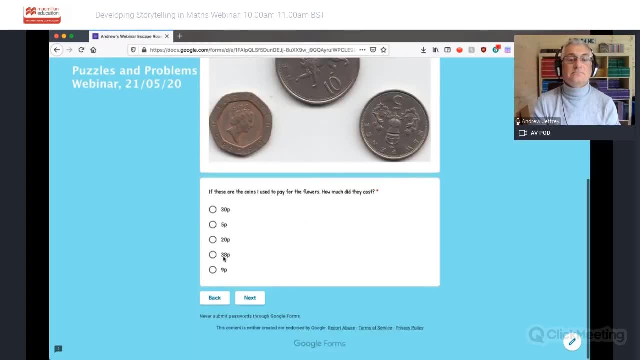 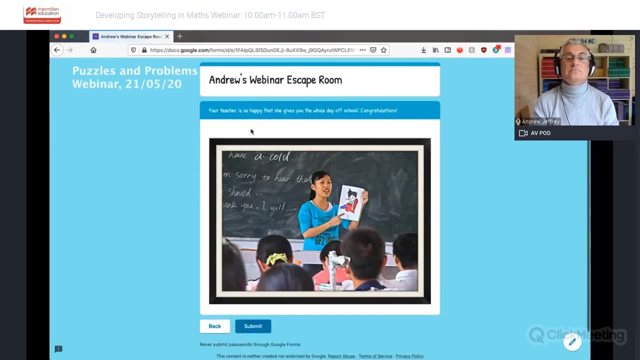 values together. okay, okay, so that's it. that doesn't say what that is, but I recognize the shape. that's 20, 30, 35, 30, 38, that's 38, oh, look so next. and it says: well done the coins out to 38 P. oh, that's good, you'll be so happy to give. 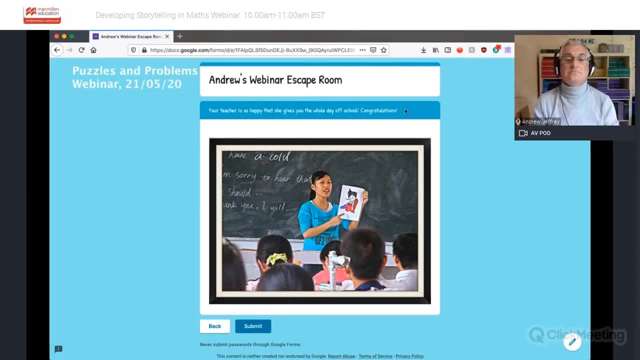 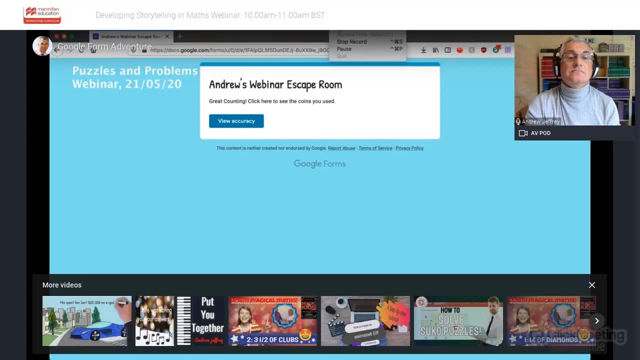 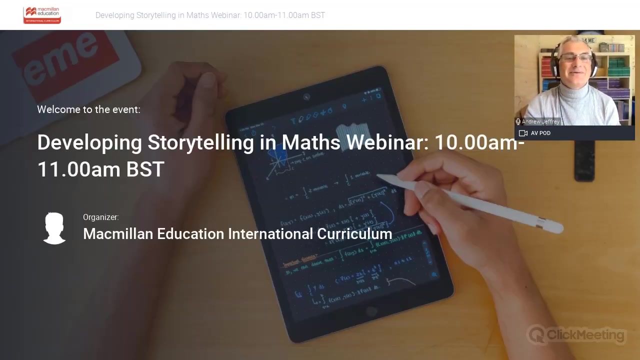 you the whole day off school congratulations. okay, that's marvelous. I'll submit that. there we go. there we go. okay, oh, hang on, hang on, hang on. oh dear, wait a minute, I've got to click this. don't tell me though. oh no, hold on a second, go back to our, go back to that, and there we go. oh phew, that was a. 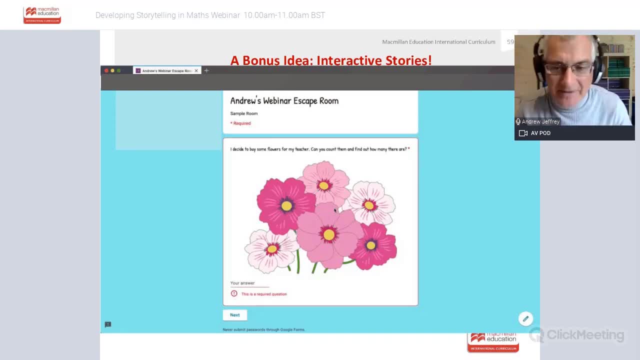 moment, right? so, um, that actually took me a bit of time to work out, um, but it's uh, it's great, uh, you can, you could create math questions and put them in, basically just a chain, so it's like a story Adventure almost like. do you remember years ago there were books called make your own Adventure and there 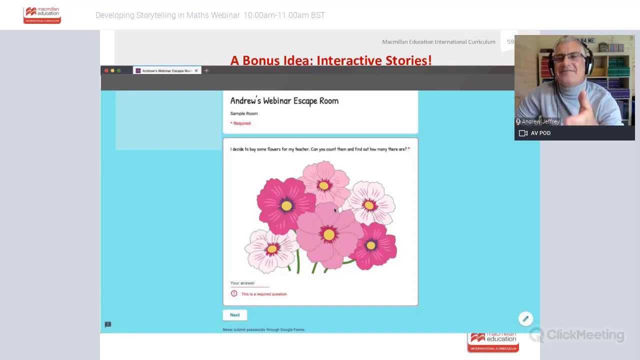 would there be an introductory page and it would say: if you want to go up the stairs, turn to page seven, and if you want to uh, go into the cellar, turn to page 12, and then the story would carry on. I thought they were genius, but you. 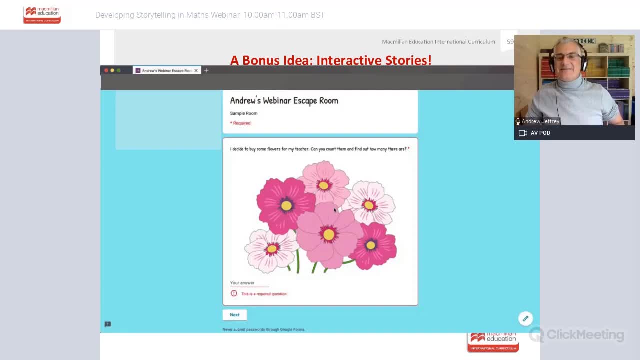 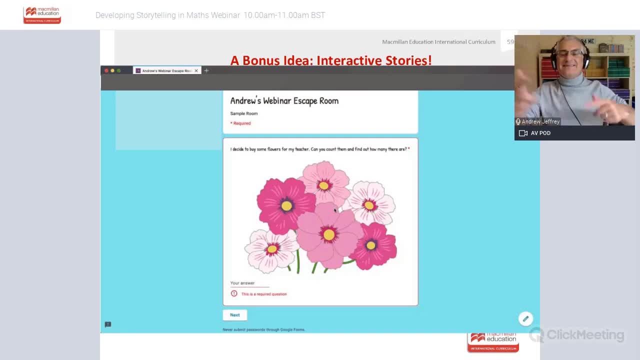 multiple choice ones, like the coins one, uh, and it can take you to different places. so that's my little challenge to you as we finish this session today. can you, can you work? get onto Google forms? it's not a hugely complex thing, uh. I, if you email me, I shouldn't have said that I will try and send out a link to a. 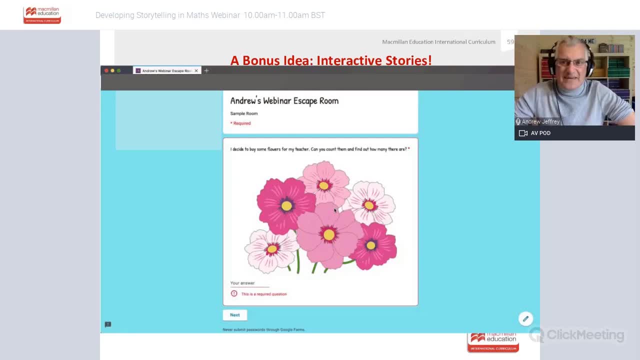 little video I made explaining how to do Google forms, but it took me. it took me work out also not much like so, look, there's some books. there's some books online. there's some books on my desk. there's some a story that you make yourself. um, I think, uh, this could be a really fun way to bring mathematics in. 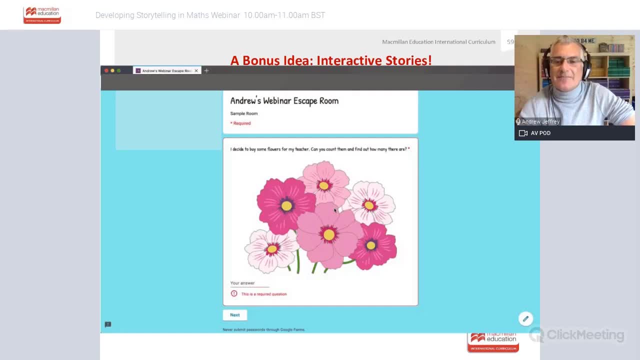 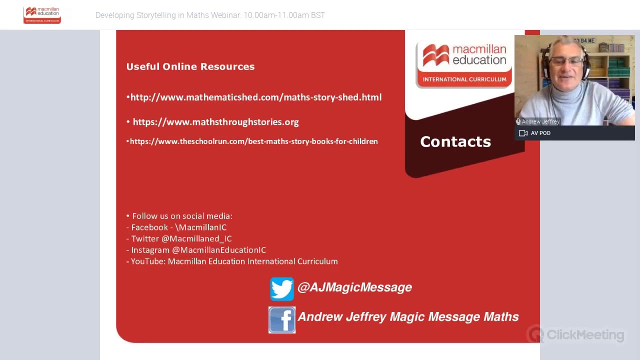 now, I promised you earlier- and some of you were asking um- what my best kind of web research was. so I spent in probably about four, three or four days just searching the internet, and there are. trust me, if you, if you type maths through stories into a search engine, you will have millions of pages. but of the millions of pages that I found, 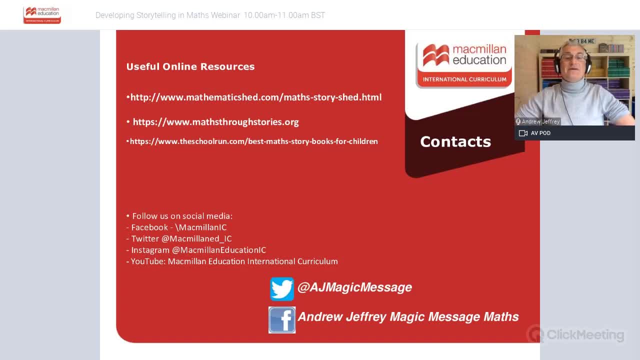 I would recommend these three to you. so mathematicsshedcom and follow the math story. shed math through stories is a whole website set up by Reading University who realized there's huge potential in math three stories and also the schoolruncom, which is aimed at parents. um they. 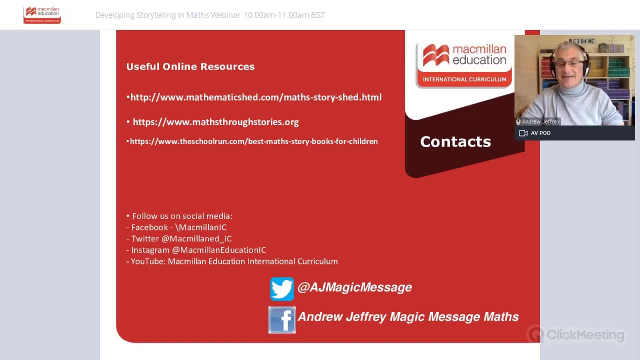 they have a really comprehensive list as well, and that's where I I certainly checked out some ideas. um, that is it from me. I'm going to hand you back to Reiner, who can be contacted. thank you to Macmillan for hosting us. here are their contact details, but for now, um, I'll be, I'll be around to. 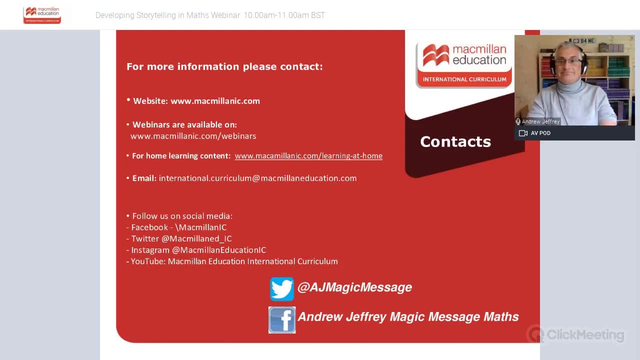 answer questions, but for now it's Andrew out. so much, Andrew, uh, for the lovely session, really engaging, and I can tell from the attendees that they really benefited both from the stories and you're getting games as well. so, uh, fantastic. um, if you'd like to ask any questions, feel free. we've actually run out of time, so, um, do contact. 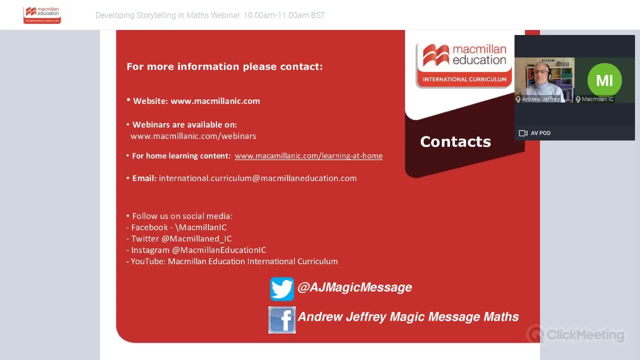 us if you have any questions. um, as I mentioned at the beginning, the CPD certificate and the PowerPoint will automatically be available via email. do check your spam and junk folder as well. do follow us on social media and also view our upcoming webinars for the rest of the year.